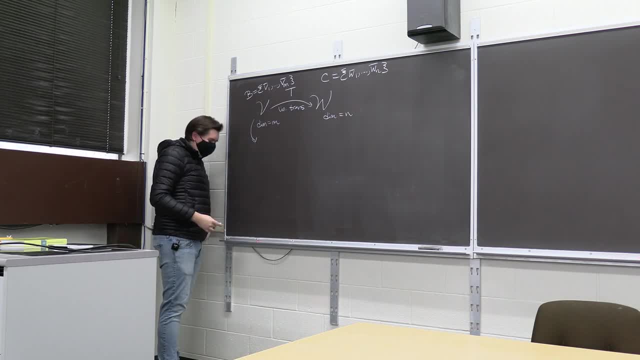 And right now we have give me a second, one second. So now I can write the Wellness s and then I can write to theold wave, since we're dimension N, any vector in V, any vector in V, if I have some vector over here. 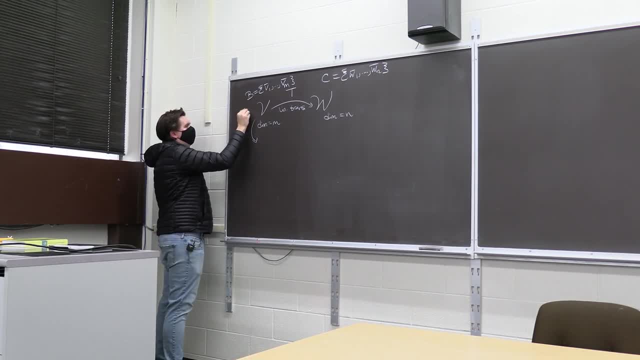 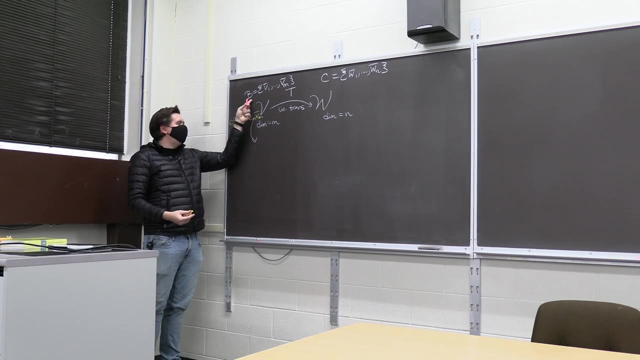 well, you can write that vector as a linear combination of V1 through Vm, right Some C1, V1 through Cm, Vm, And then one way to think about that vector. it's like: well, if I know, my basis is B. 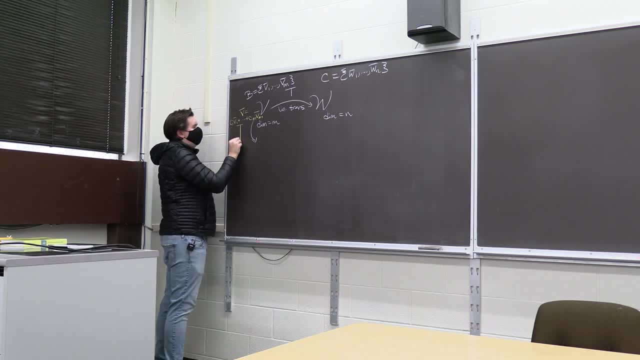 I just need to keep track of these coordinates So I can send this down to the vector. that's just the coordinates. That's just the coordinates C1 through Cm. And now this looks like the kinds of vectors you're used to from your first course in linear algebra. 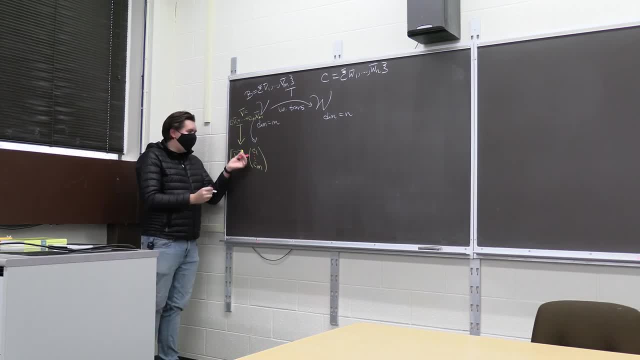 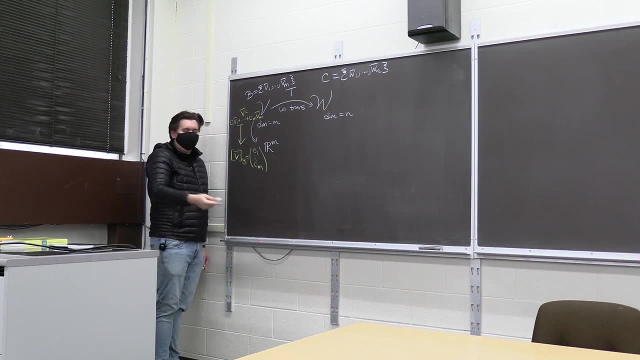 If all of your C1 through Cm are real numbers, this would be an Rm. More generally it's an Fm. I'll just call it Rm here, but this R could be like complex numbers or whatever field Your values are fun. 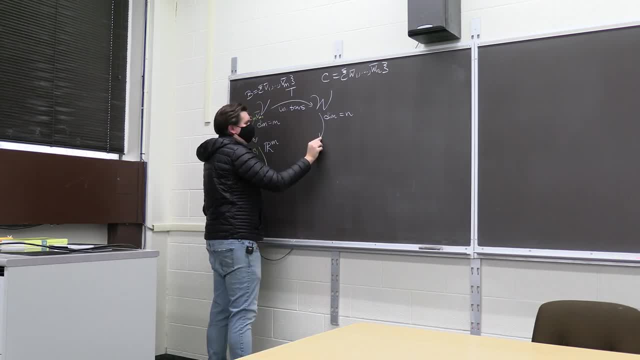 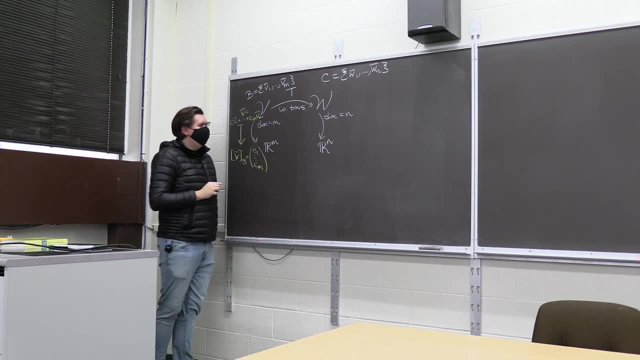 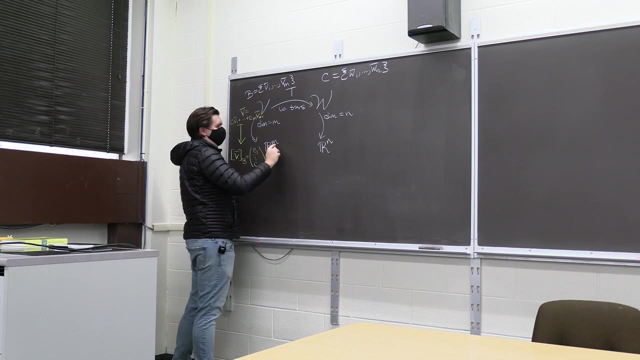 And similarly, we can take things in W and map them down to their coordinate vectors to get something in Rn. And so what we're saying is: you can represent V in W by Rm and Rn by just reading off your coordinates, And so therefore this T can be thought of. 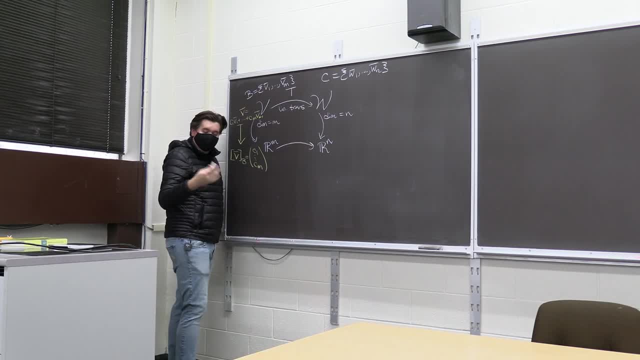 as what's the corresponding thing between Rm and Rn? And the answer is: it's a matrix. Read your notes. Note the matrix with square brackets around T. We're going to specify. we're moving from the basis in B to the basis in C. 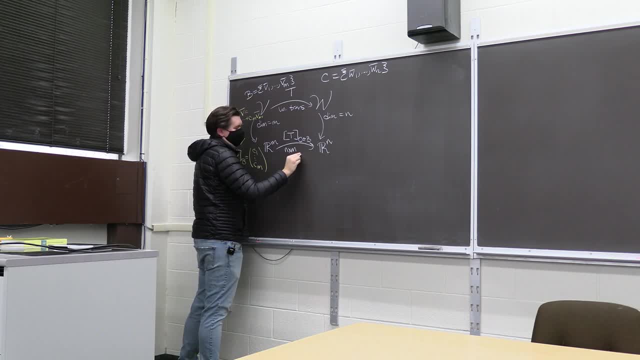 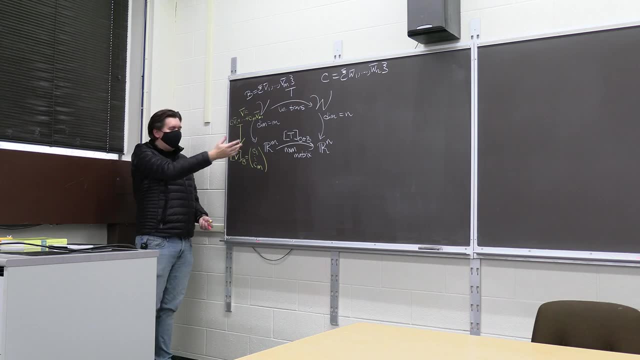 And this is an n by m matrix, Right? So that's what we said. So when you have a diagram like this, you might think there are two ways to travel this diagram. One way is you start out with a vector in V. 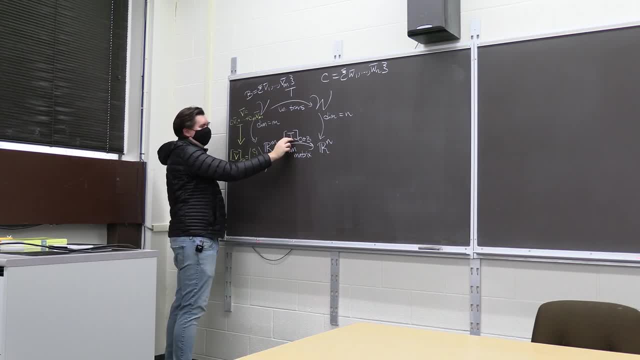 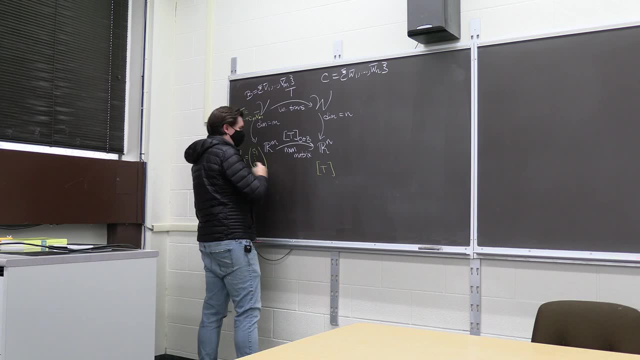 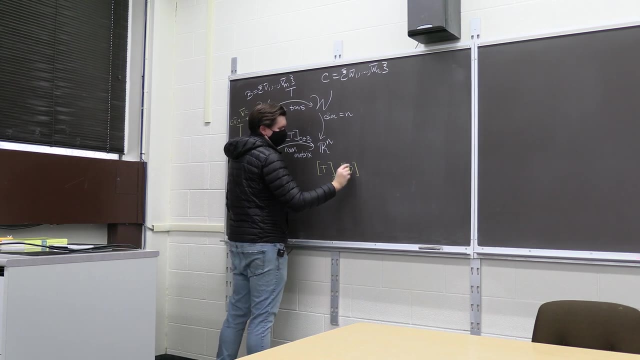 You map it down to its coordinate And then you apply this matrix T to it. So you're going to be doing the matrix T times this vector V. So this is the matrix that goes from B to C. And here's the vector in terms of the basis B. 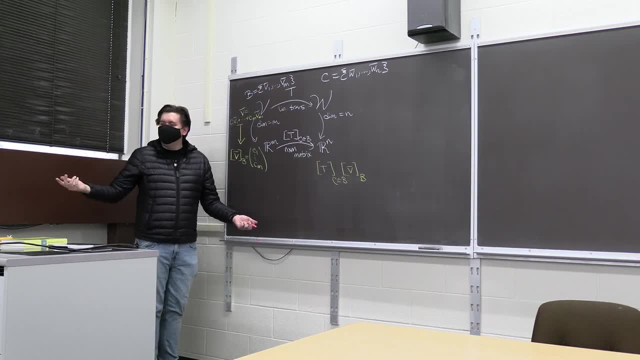 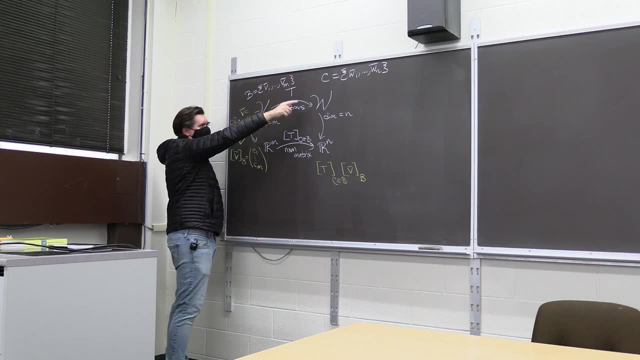 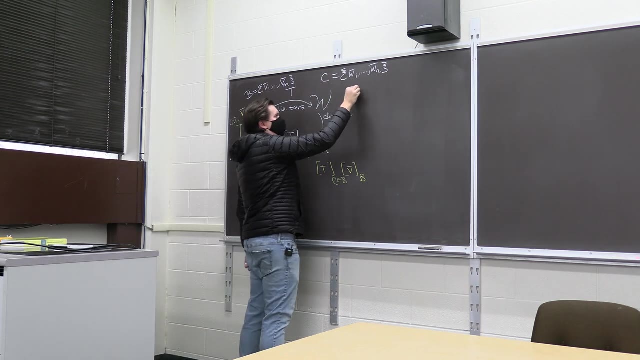 That's one way to travel. What's the other way to travel? Well, we just can go like this: Instead of going down and right, we can go across the top and down. So V going across the top will get sent to whatever T does to V. 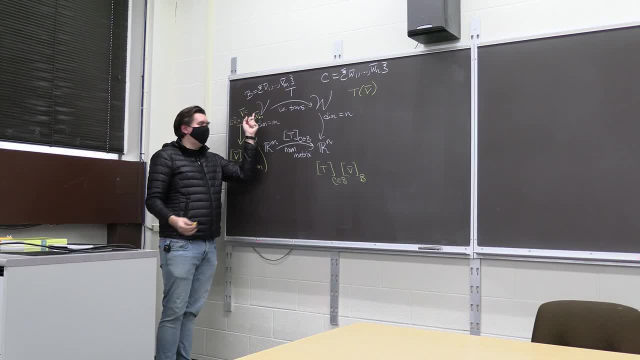 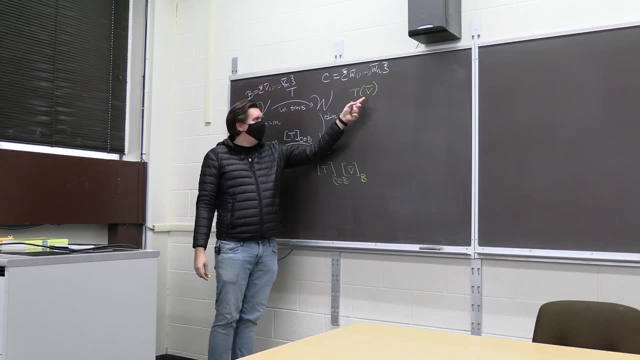 whatever your transformation does, Maybe it's taking the derivative of V, If V is like a polynomial and this is the derivative map. Maybe it's taking the transpose of some matrix. Whatever it's doing, your transformation's happening to V, And then you can send this guy down. 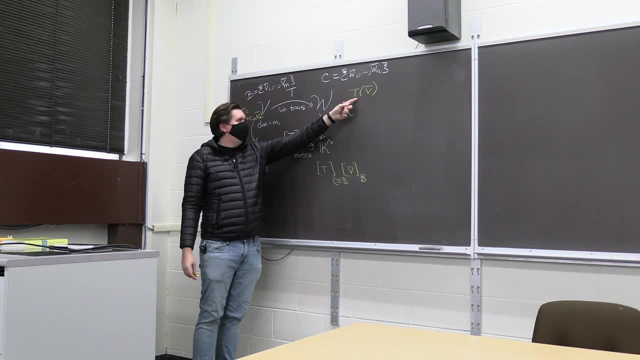 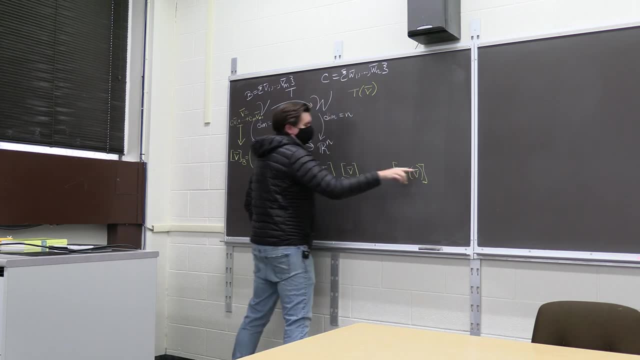 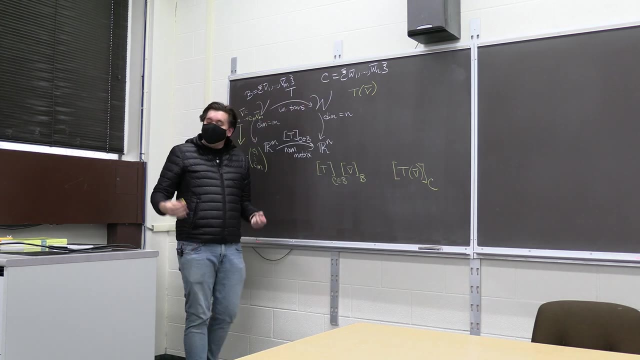 by looking at the corresponding coordinate vector for this guy. So the corresponding coordinate vector for this would be T of V's coordinates expressed with respect to the basis of W, which is C Expressed in terms of the basis C And our big theorem last time. 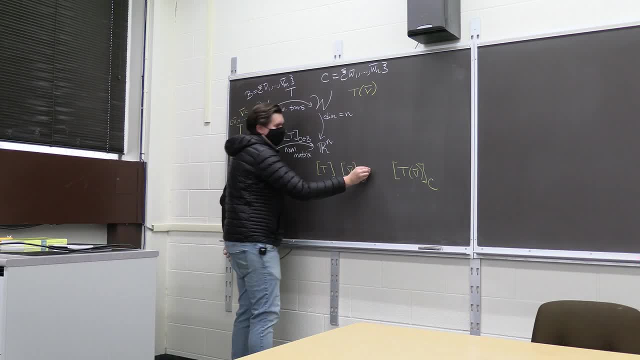 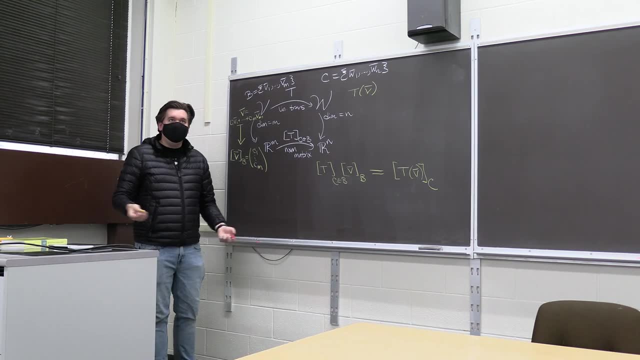 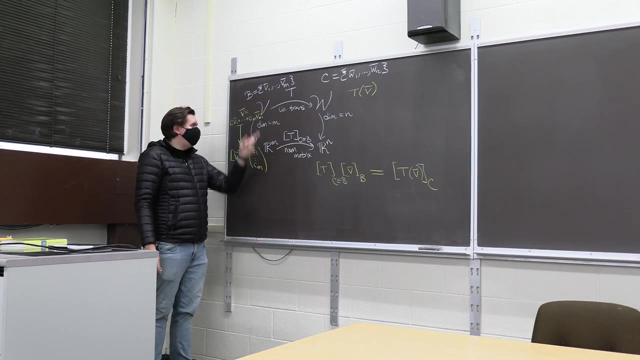 was simply saying these two ways of travelling the diagram give you the same thing. So if you take something like abstract algebra and you get into this- this is going to be called, you're going to often say things like the diagram commutes, which just means you can travel either direction and get the same thing. okay, so 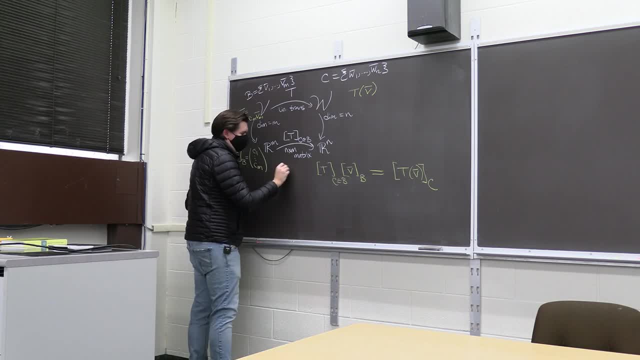 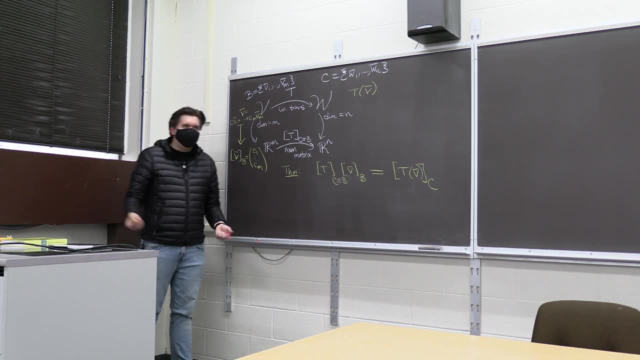 that was our theorem. this, this was where we showed last time. I don't know if I call it a theorem or proposition. let me just call it a theorem. we proved it last time already. I think what I'll do today is give you one more example of this. so 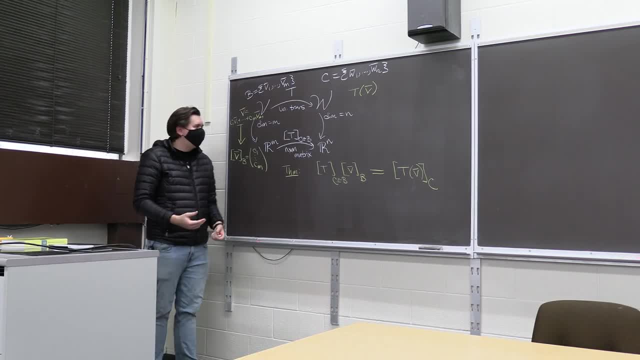 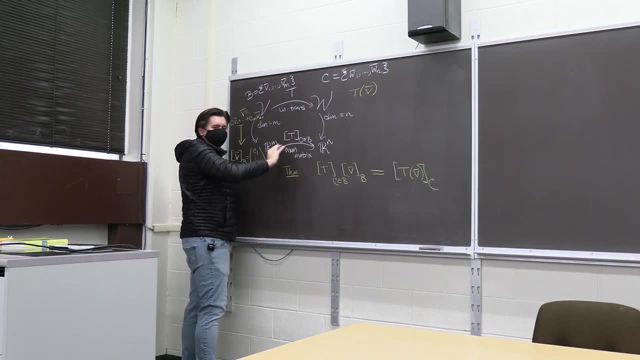 if he's a little more concrete, and then we'll look at some further properties of well, how can we think of linear transformations as being associated to matrices? how does changing this in fact this right? so that's our goal. talk about some properties, but but first let me give you one more concrete example. so, so, 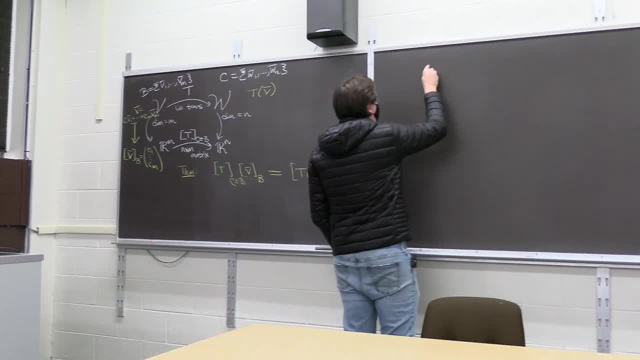 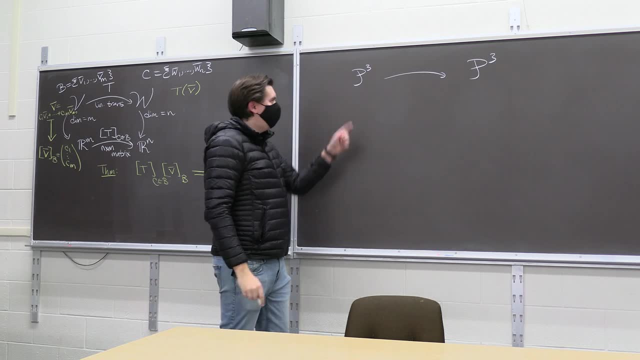 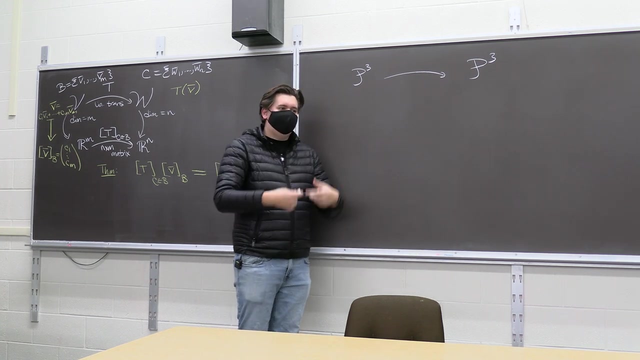 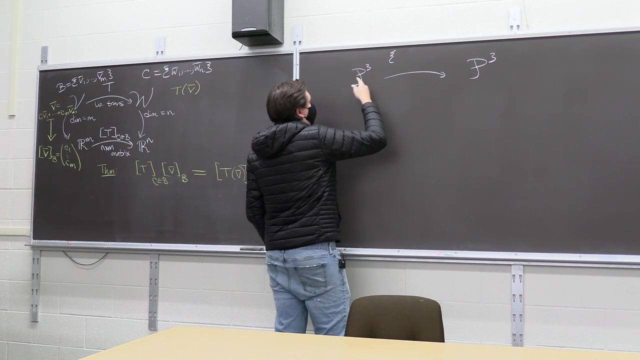 let's set this up over here. well, let's have a map, say from p3 to p3 we call. by p3 I just mean my cubic polynomials, or polynomials up to degree three, so constants, linear quadratics and cubics. that is. this guy has a basis which is one X, X squared and X cubed. that's kind. 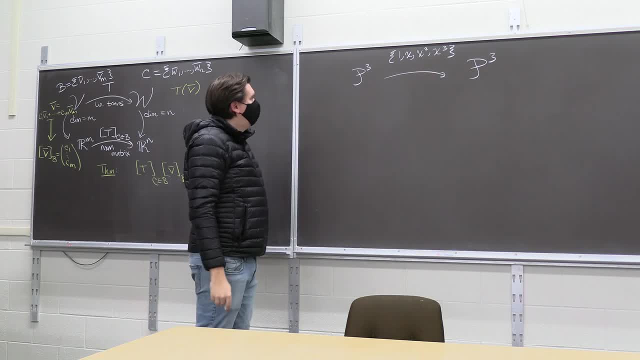 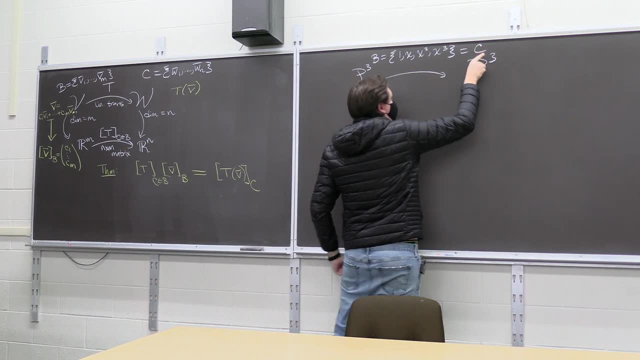 of the standard basis, that's a standard basis for p3, and both of those have the same basis. so you could say this has some basis B and this has some basis C, but they're both the same, the same basis. so we're gonna do everything with. 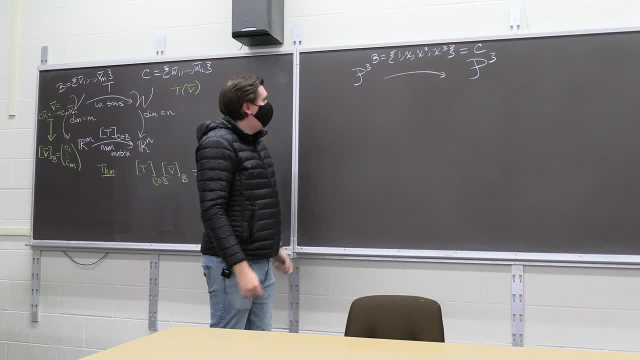 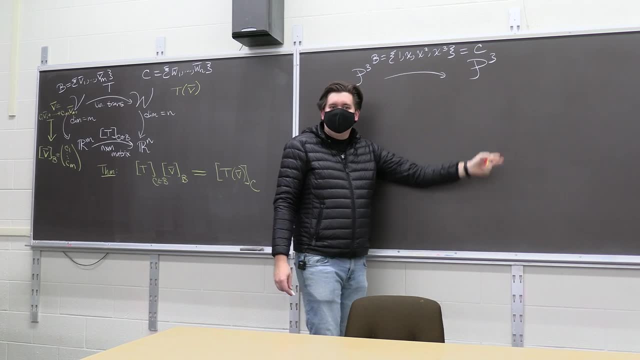 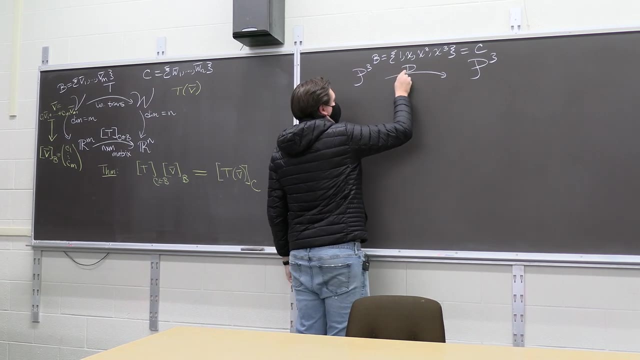 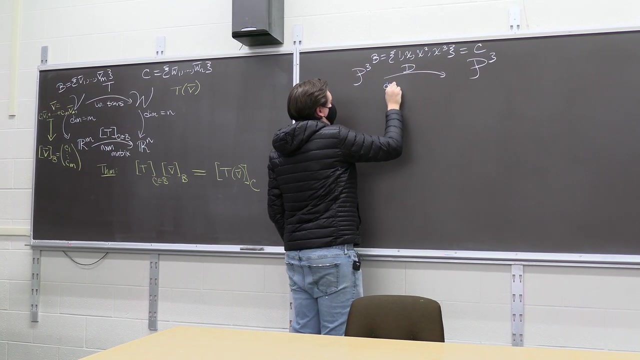 respect to that basis. now, what is like your favorite linear transformation to change some polynomial into another polynomial? well, there are lots, but let's focus on the derivative. so I'm going to say my map D here is just the derivative with respect to X. so it's my derivative. derivative with respect to X. 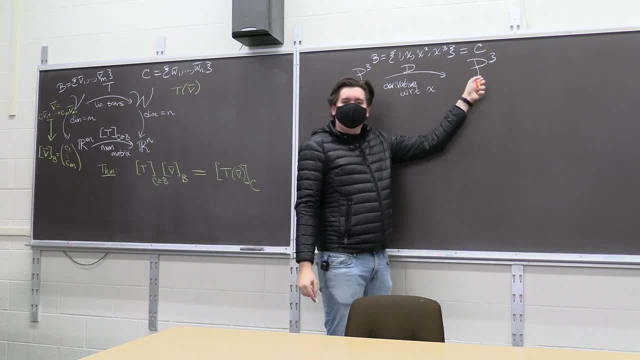 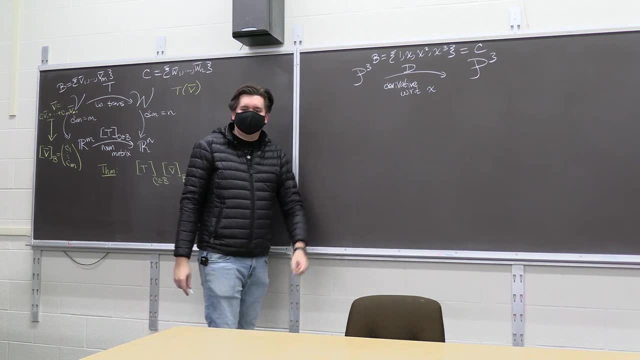 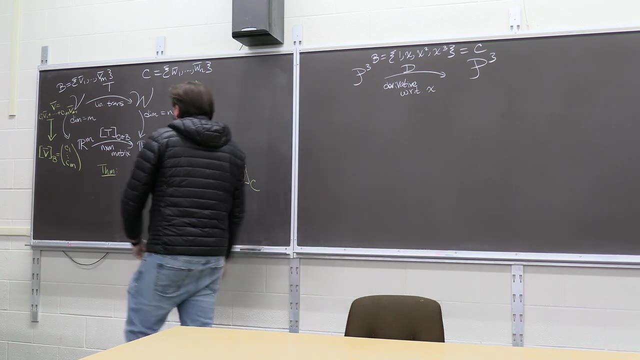 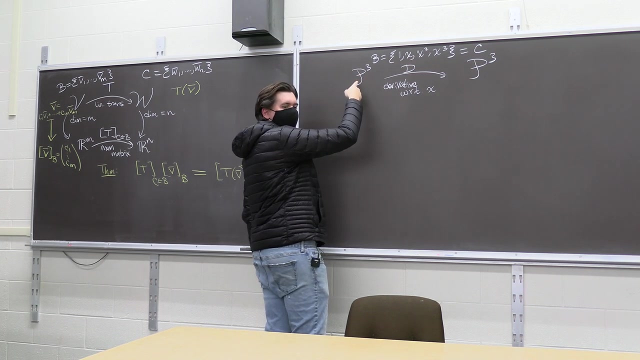 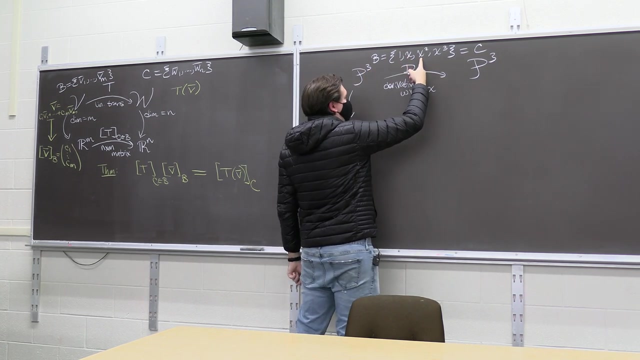 right. so like X squared is just going to get mapped to two X. so this is just calculus one. okay, well, our story is that, corresponding to that derivative, there should be some matrix. so you're like: okay, this is p3. what's the dimension of this vector space? you might think it's three, but be careful, it's actually four. 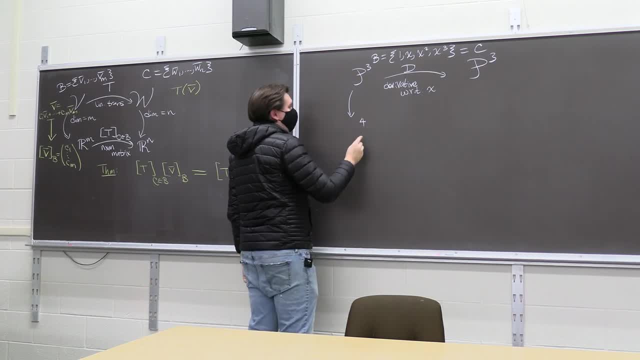 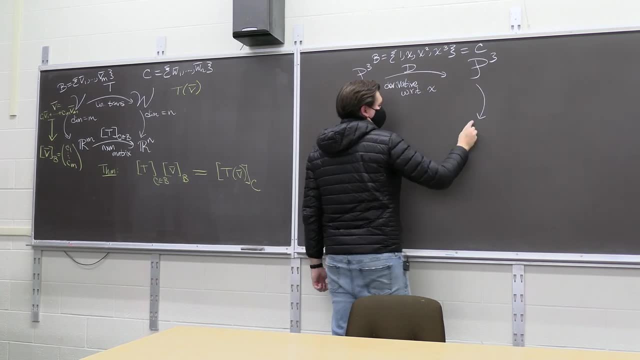 because you have a one X, X squared and X cubed, and so that's how you dimension coefficients are in the reals. so this can be mapped down to R4, and this can be mapped over here to R4 as well by just reading off the coefficients. So as a concrete example of this, 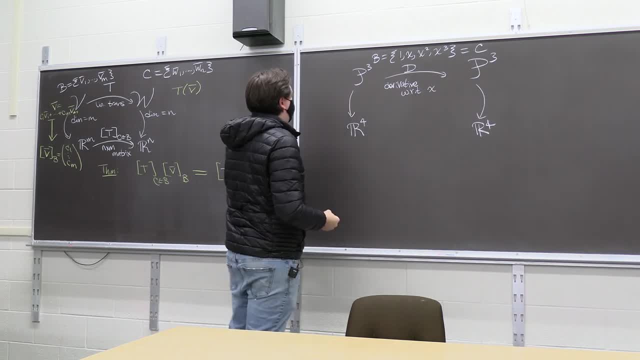 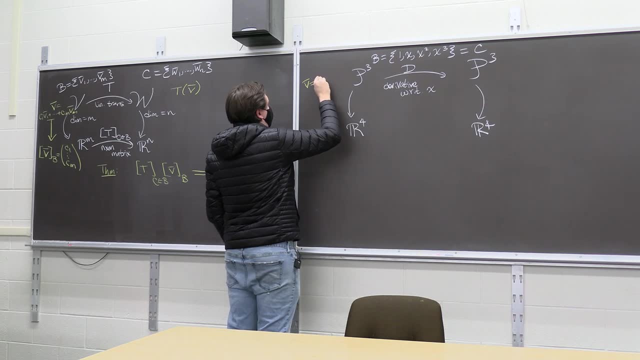 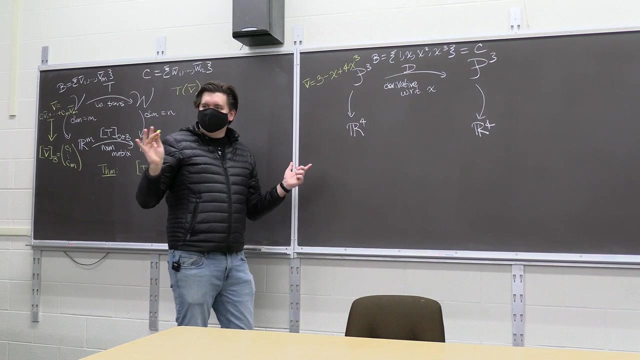 let's look at some vector that lives inside of P3.. So a vector would just be some polynomial, so something like, oh I don't know, 3 minus x plus 4x, cubed right. That's an example of. 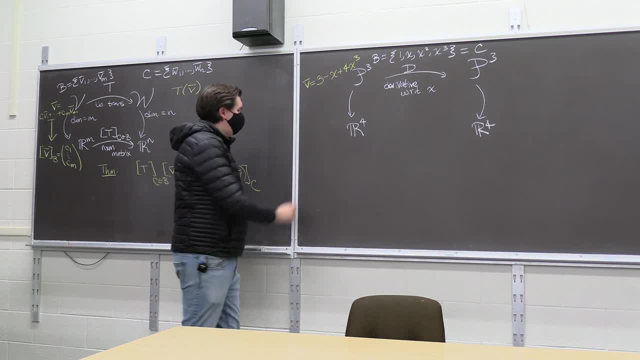 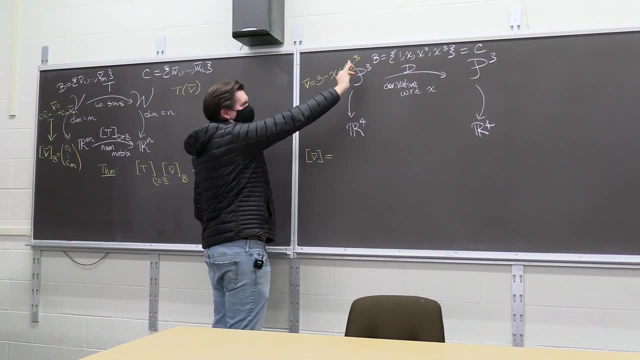 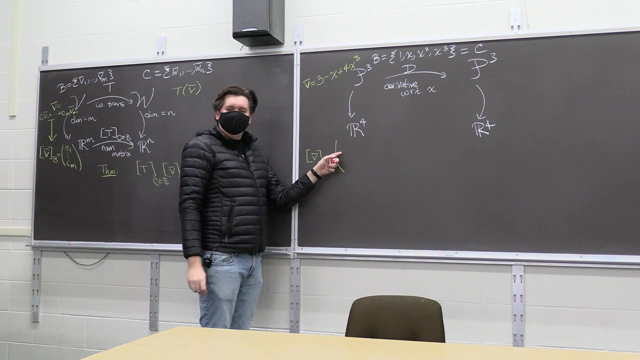 something that lives up there. So what will that get mapped down to? What's my corresponding coordinate vector with respect to my standard basis? When we have a single basis, I won't write b every time. It's clear which basis we're talking about. What's my corresponding? 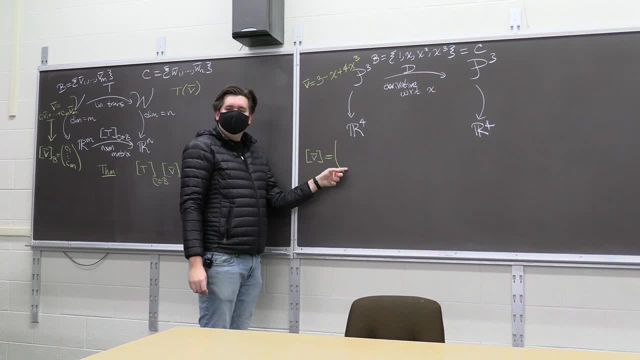 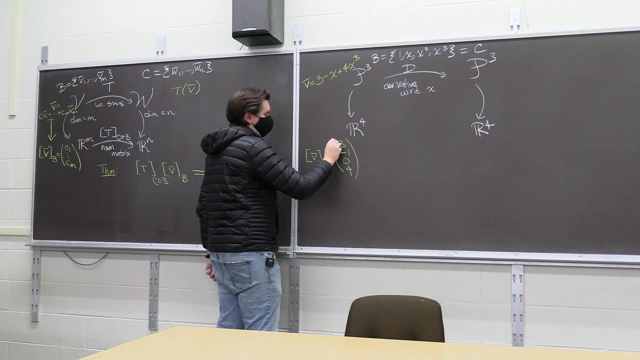 vector, A vector, a coordinate vector, that this gets mapped down. to Go ahead and shout it out. Yeah, you just read off the coordinates in the order of your basis elements, The 1,. well, you have 3 here, so that's 3 copies of the first one minus 1 copy of the second. 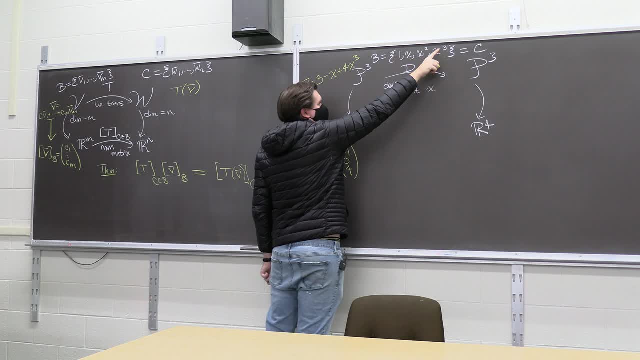 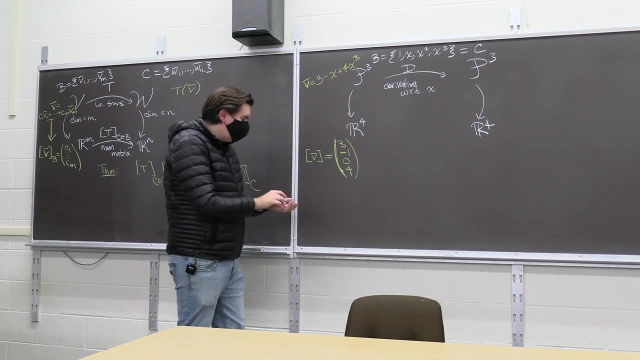 plus 0 copies of x squared, Plus 4 copies of x cubed, And so your coordinates is 3, negative, 1, 0, 4, right, Okay, what we want to do is we want to figure out, well, what is the corresponding matrix. 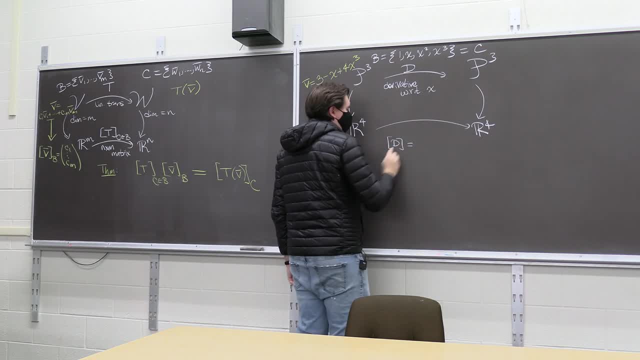 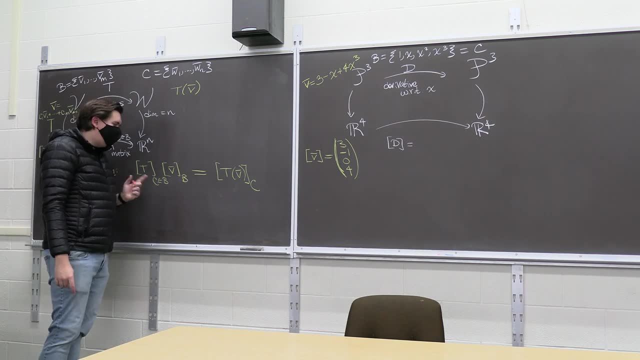 here. What does the matrix of D look like? And so, if we go back to our theorem, our theorem actually gave us a little bit more. Our theorem told us what a matrix looks like. Last time we said that this is equal to this. where? 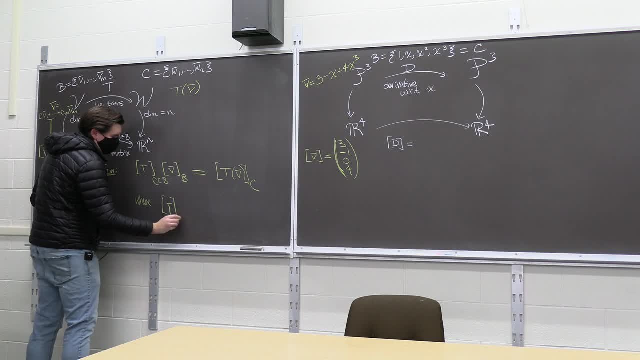 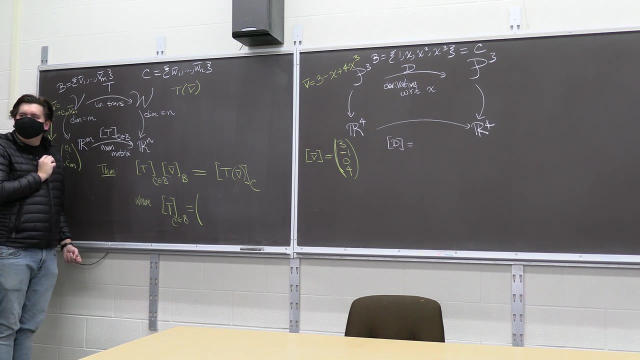 This T, the matrix crossbinding to T, is. just, do you remember? Do you remember how we get it? How do we figure out what the columns of this are, The basis vectors in B, Exactly, We just reach column we say: what happened, We're going to get a vector, exactly. We just make a column. So the idea is we typically get the Maar-Somers minimum, The numerical number, remember the variable A is E, And so maybe the E is the number up, so the E is the number down, The 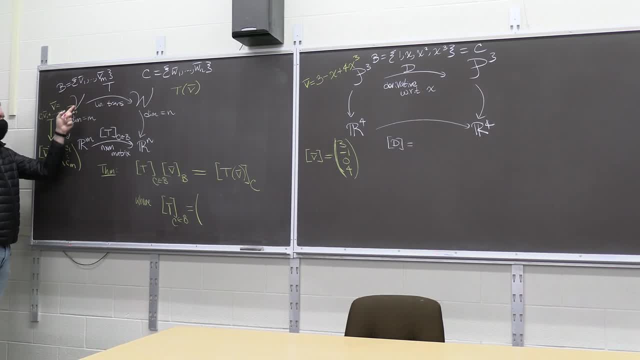 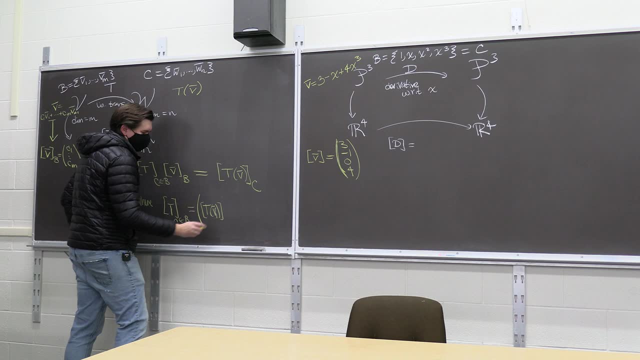 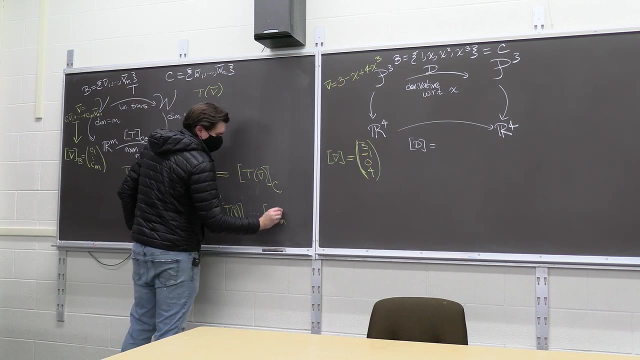 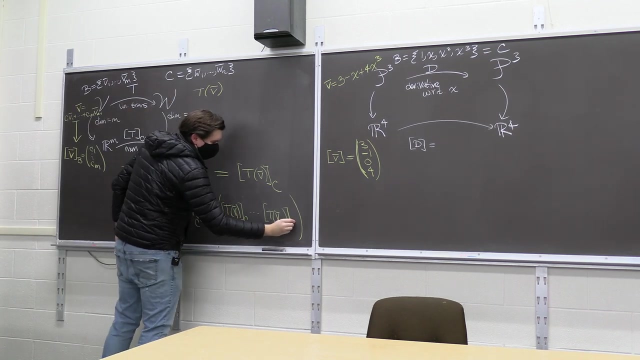 happens to the basis vectors, starting off with these basis vectors in V. So we say, what does the transformation do to V1? and then you can turn that into a column vector down through. what does the transformation do to the last guy, Vm, and then you express those in terms of your new coordinate system, C And like no sure. 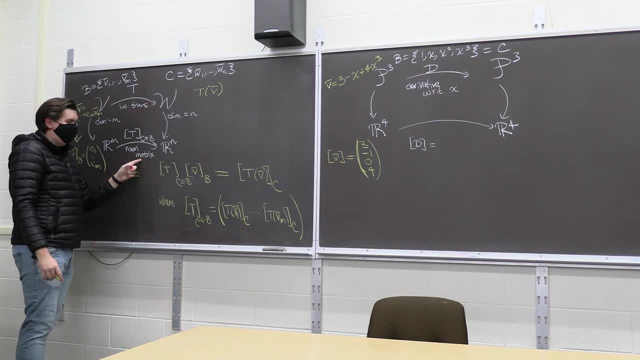 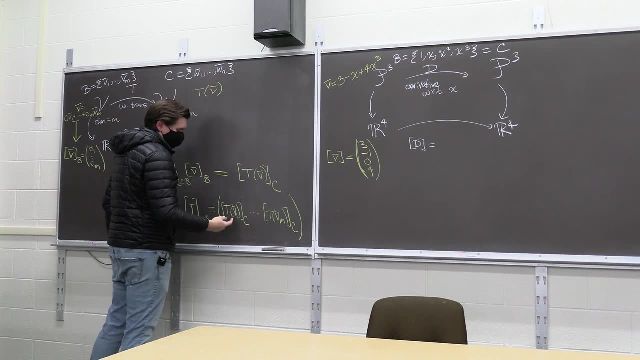 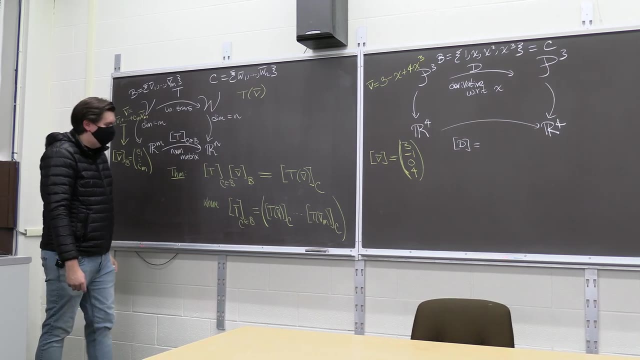 enough. this will give you an n by m matrix. There'll be n rows, because these guys are in C, where there are n entries, and there'll be m columns- m columns corresponding to the m basis elements in B. So we can just do that here like what. 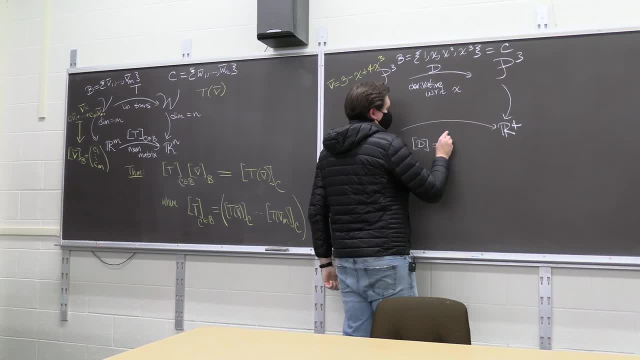 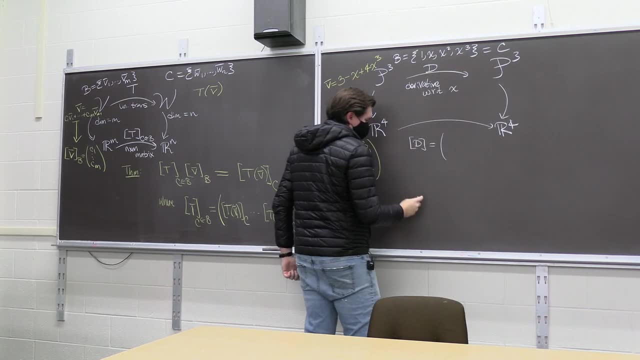 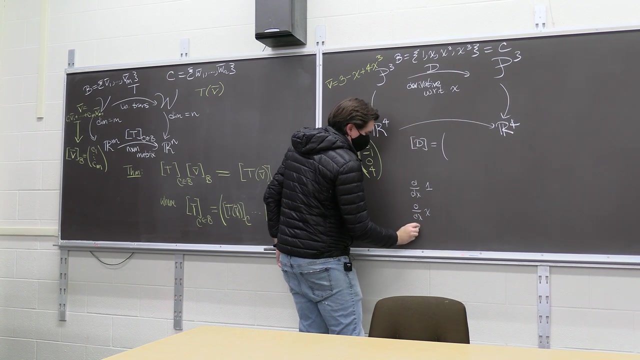 should your D be? Well, D is going to be found by just asking: what does the derivative do to each of these elements? So I mean we can do it here. What does the derivative do to like 1?? What does the derivative do to x? What does the derivative do to x squared And? 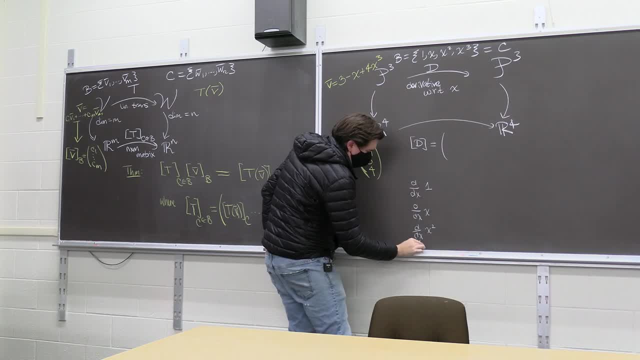 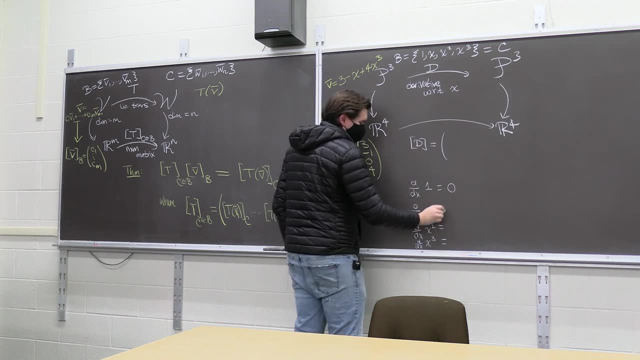 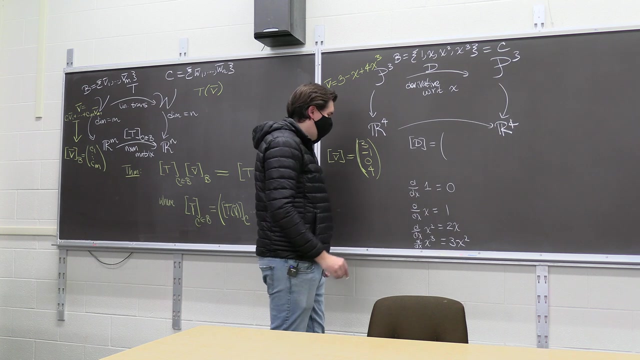 what does the derivative do? squeeze them in down here to x cubed, Like 1 just gets sent to 0, x gets sent to 1, x squared gets sent to 2x and x cubed gets sent to 3x squared. And what we want to do? 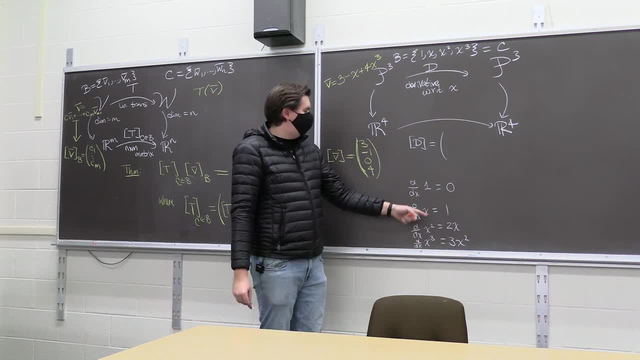 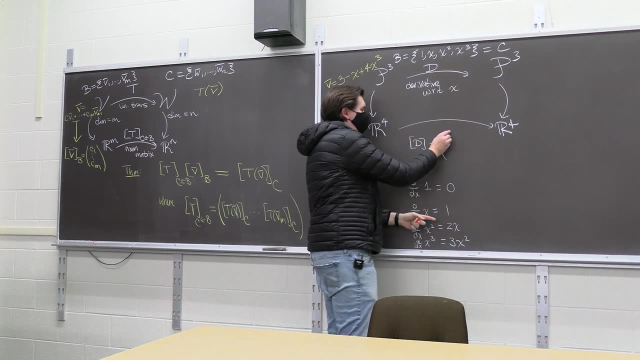 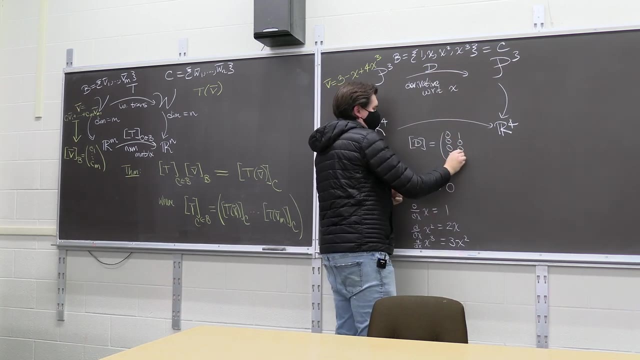 now is, we want to write those in terms of the coordinate vectors. So so what are these polynomials written in terms of this basis? Well, 0 is just 0, 0 of everything. 1 is just one copy of the first one and 0 copies of the rest. 2x is 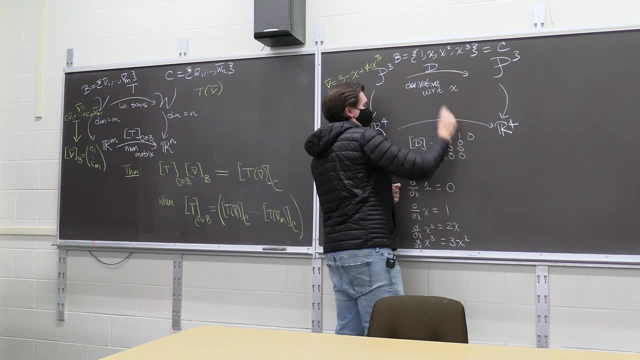 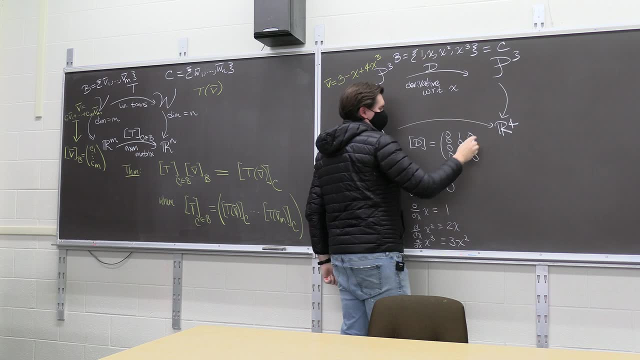 0 copy of the first, 2 copies of the second and 0 copies of the rest. And 3x squared is just going to go to x squared and x squared is going to go to x squared. So this is going to be 0 copies of the first two, 3 copies of the third and 0 copies of. 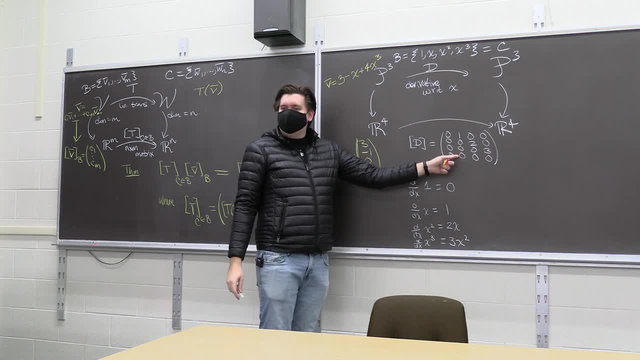 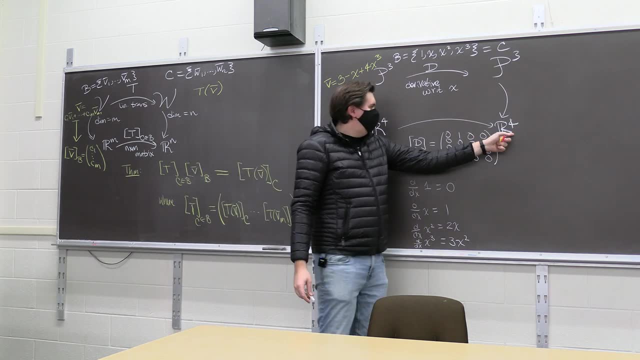 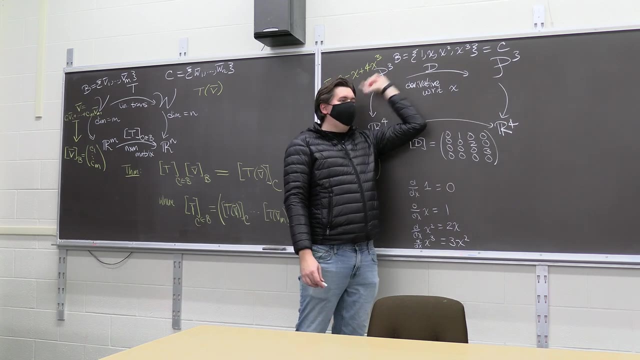 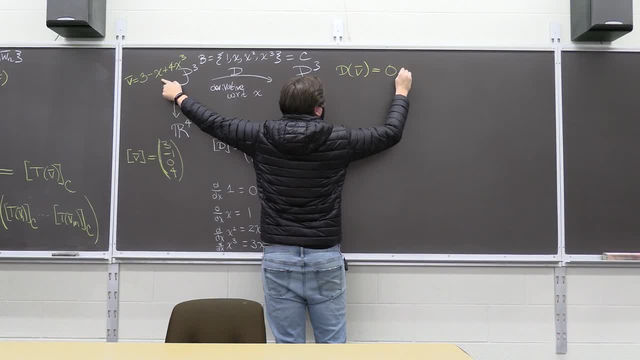 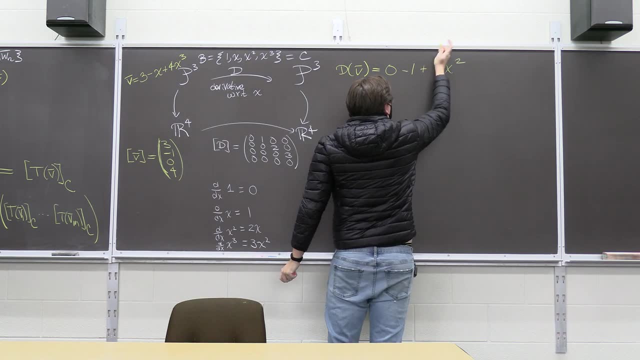 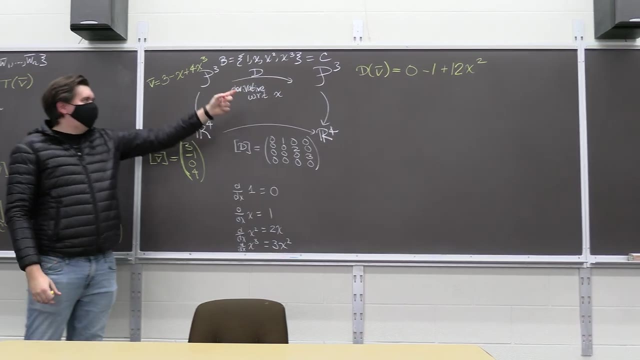 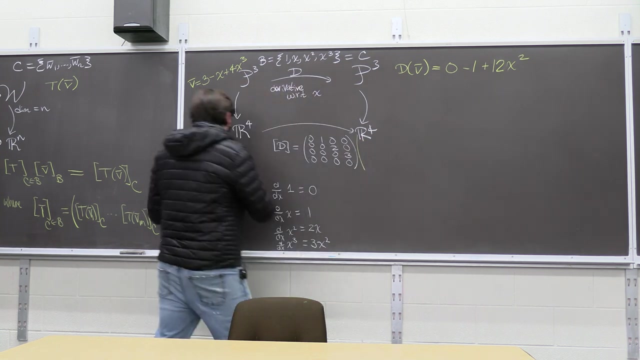 of v is just going to be 0 minus 1 plus 8 x squared, Nope, Plus 12 x squared. We know the derivatives, But what's the corresponding thing do down here? Well, you take your matrix and you multiply it by your vector. 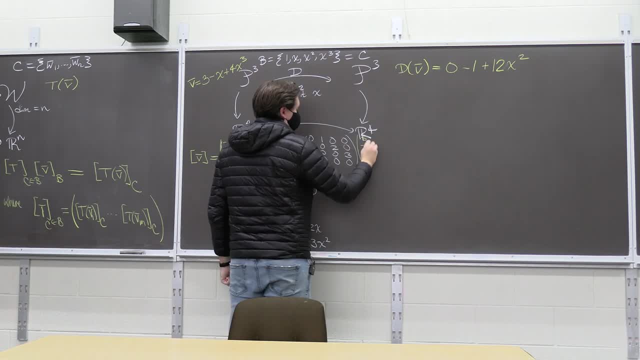 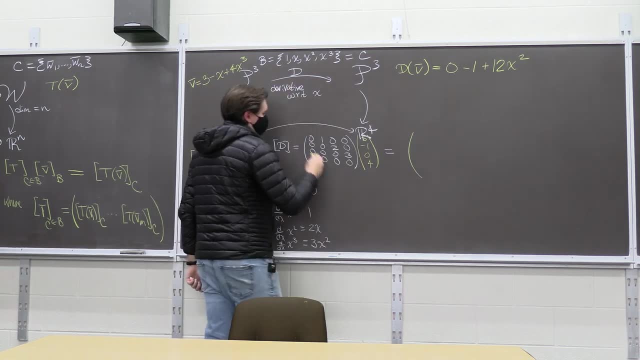 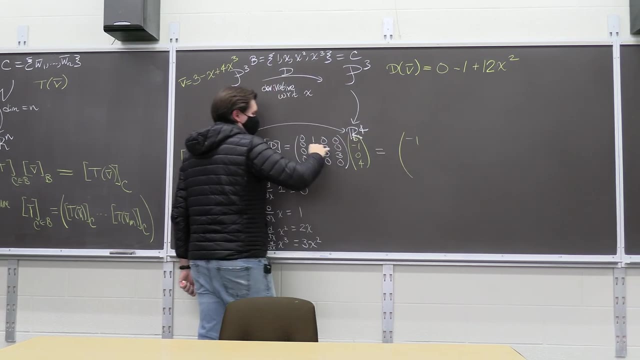 D of it 0.. Enemy: negative 1 equals d minus 1.. a four. and what does that give you? What's the resulting guy Row times column. so on top you'd get a negative one. Next row times column: the two gets times by zero. 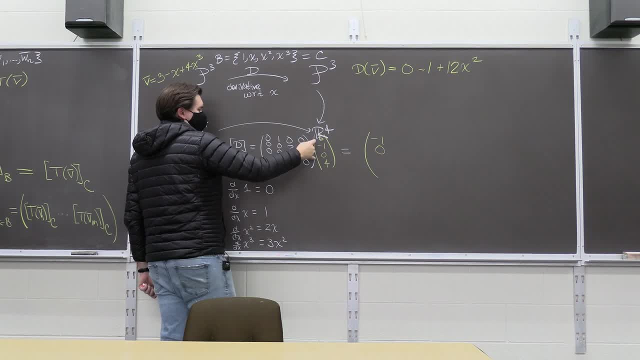 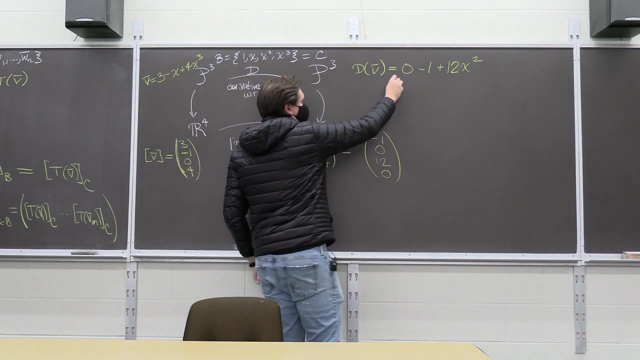 the rest is zero. so it's zero. Next row times column, you get three times four, which is 12, and last row times column is also zero. and notice, this is exactly the coordinate vector that corresponds to this matrix, to the polynomial. 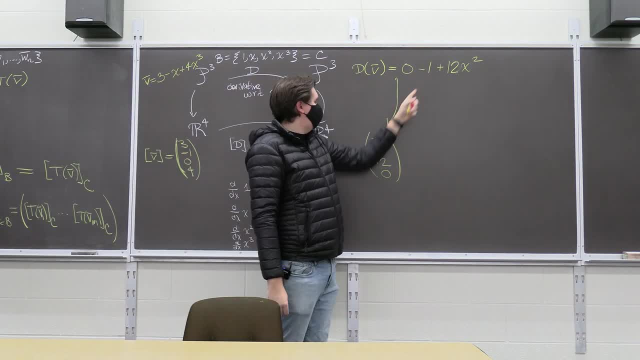 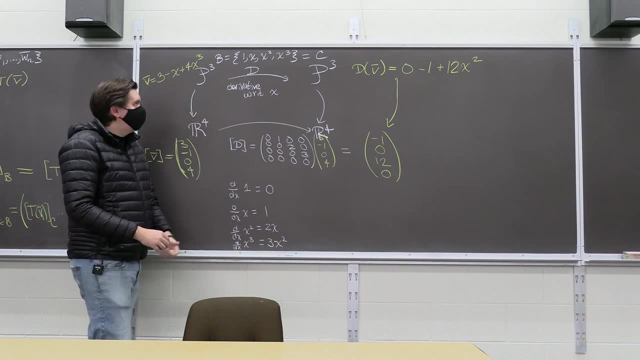 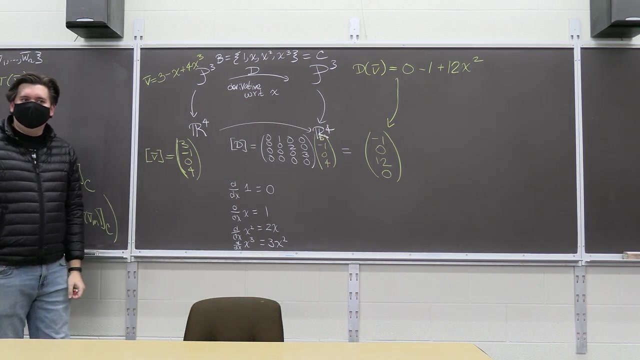 Negative: one copies of one, zero copies of x, 12 copies of x squared and zero copies of x cubed. So we can find the derivative by multiplying by the corresponding derivative matrix. Okay, are we happy with this story? I mean, this is a cool story, right. 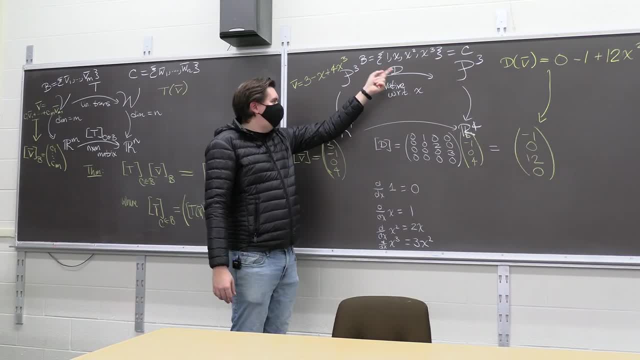 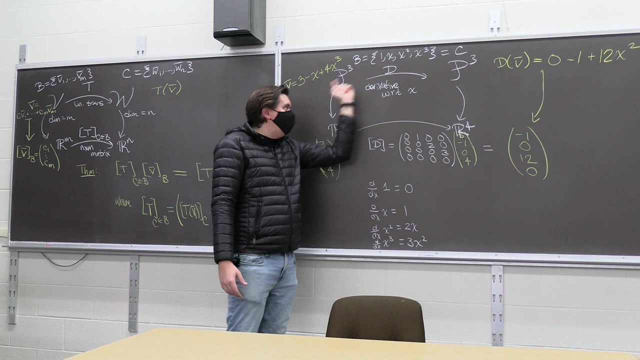 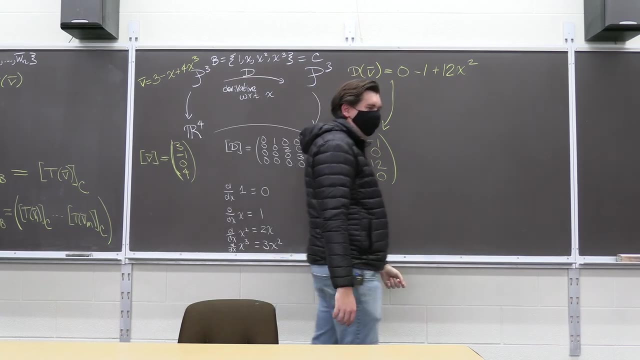 Like we just took something that's like a very calculus-y thing and we expressed it as a linear algebra kind of thing as matrix multiplication, And our theorem tells you you can do this for any linear transformation between finite dimensional vector spaces. 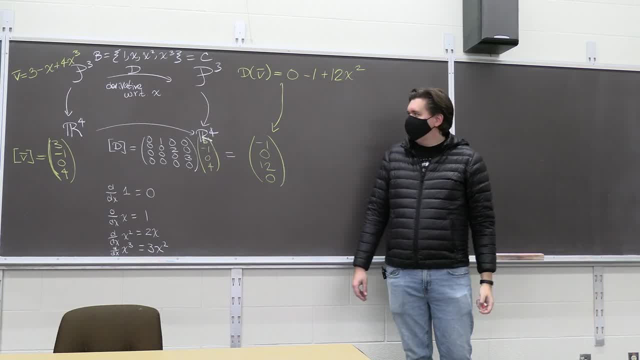 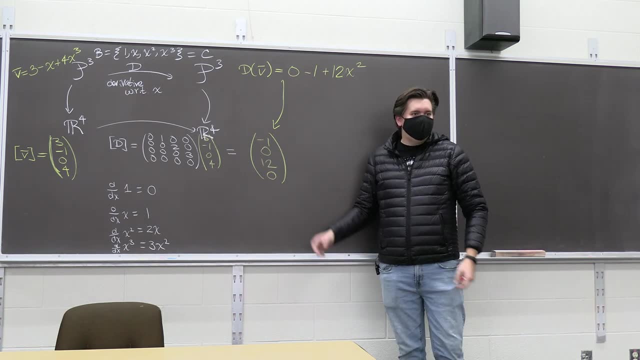 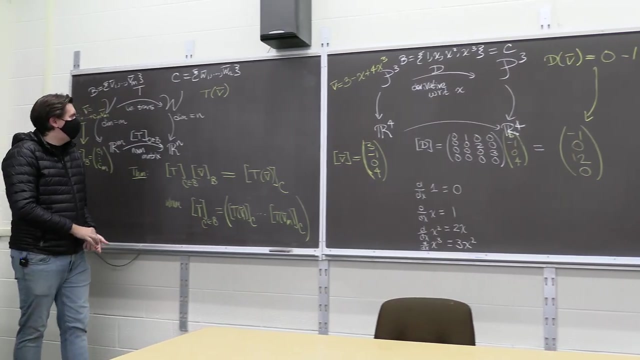 So what are some questions you have about this story before I mention some properties? Good, Happy, Yeah, Okay, Well, I don't want to belabor the point, but hopefully that makes it very concrete what we're doing here. 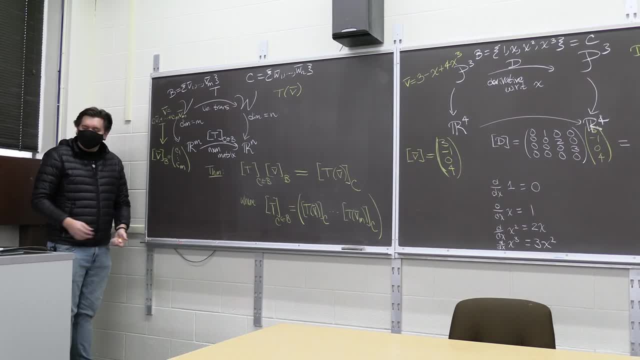 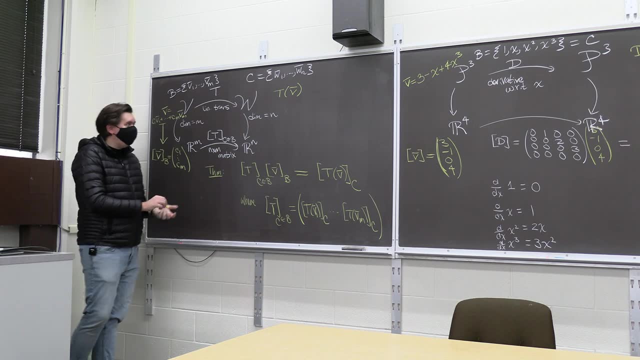 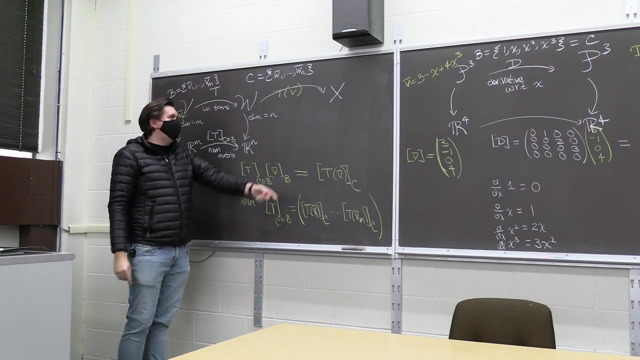 And if we come back to this picture, though, we might imagine a scenario where we don't just have vector spaces v and w and one linear transformation between them, but you might have another vector space- I'll call it, say, x- and some other linear transformation. 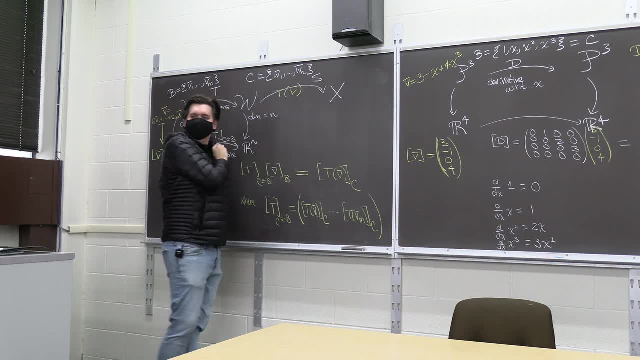 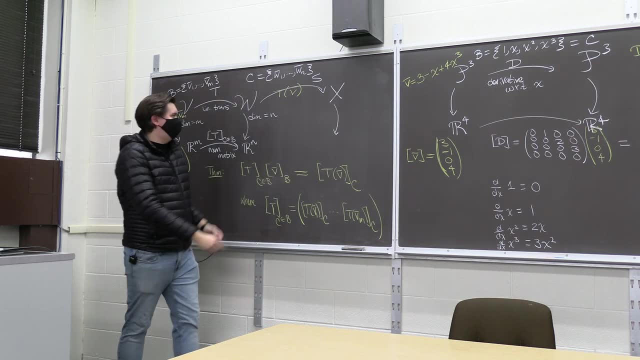 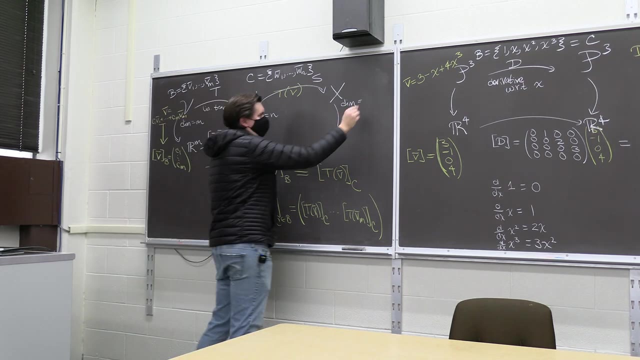 between w and x, some linear transformation, s, And then x has some corresponding. I don't know what's the dimension of x. Well, I've already used m and n, so this is kind of not following the order of the alphabet, but I'll call it l. 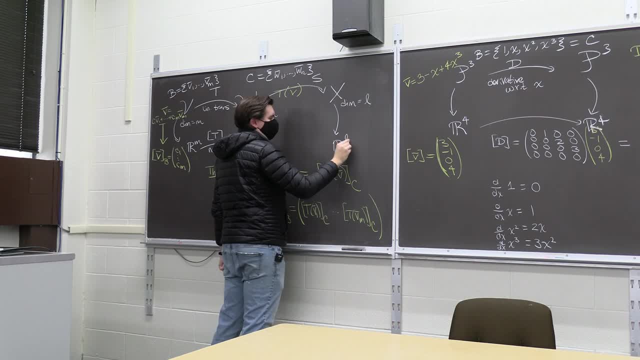 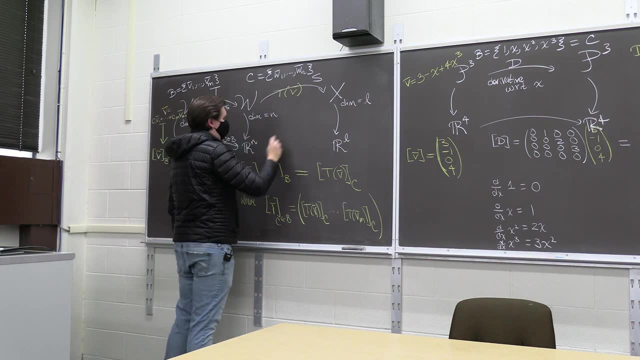 So you can take vectors in x and find the coordinate vectors which would be in our l say, if you're working with real, these scalars are real-valued, And then you can represent s by some matrix corresponding to s, and you know. 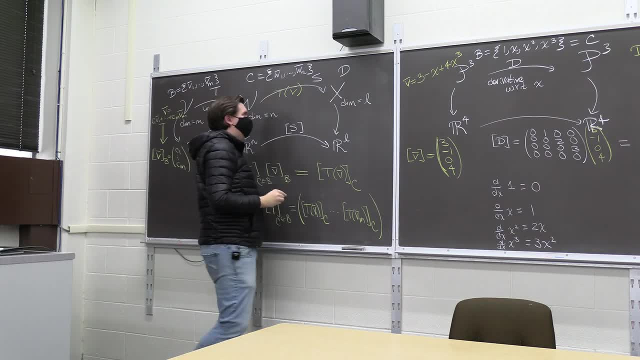 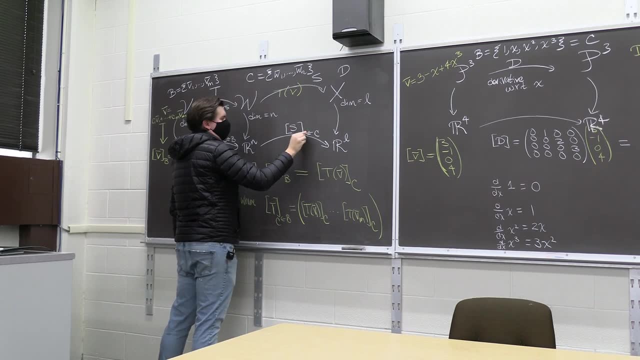 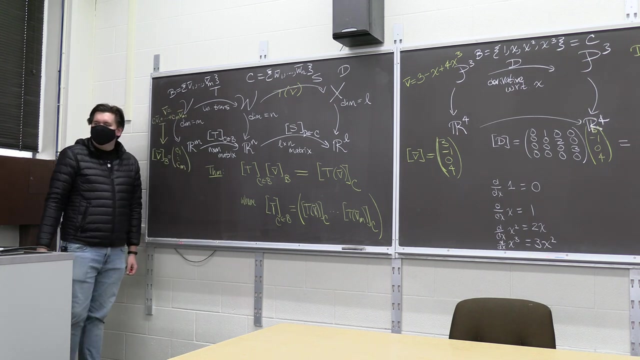 this is going to have some basis. so let's say this has some basis d. So s is a matrix that's taking things in basis c into basis d. This is now going to be a l by n dimensional matrix. And you might wonder: OK, I have two linear transformations. 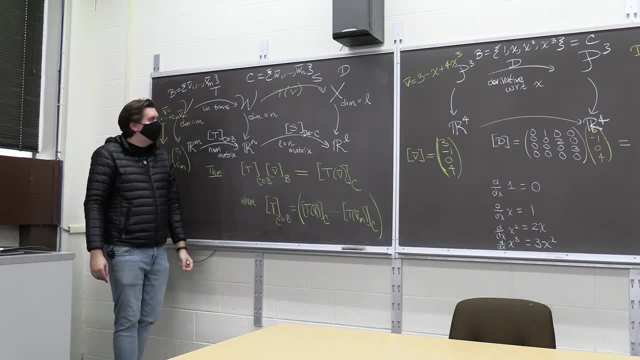 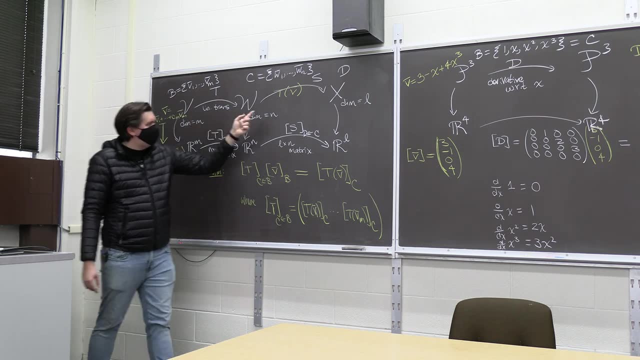 up here. I have two matrices down here. Well, with linear transformations I can combine them. Instead of just thinking about the linear transformation from v to w or w to x, I think about the composition of those linear transformations. that takes me from v all the way. 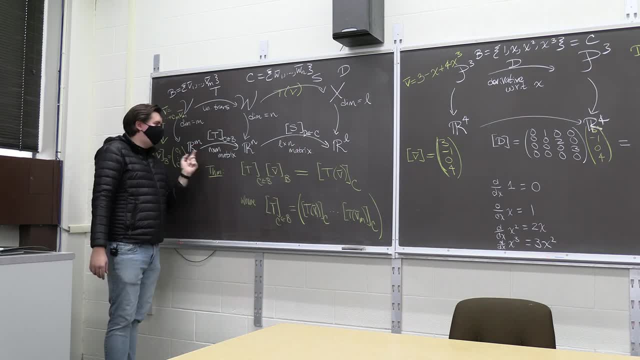 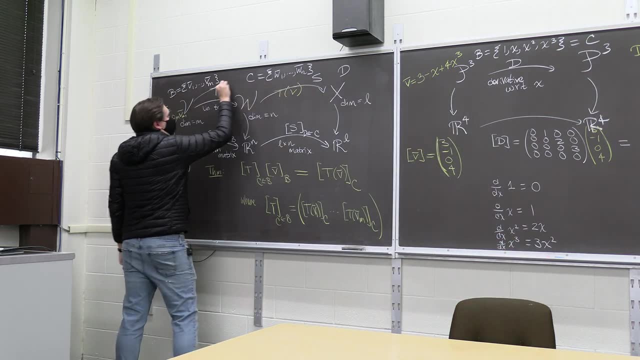 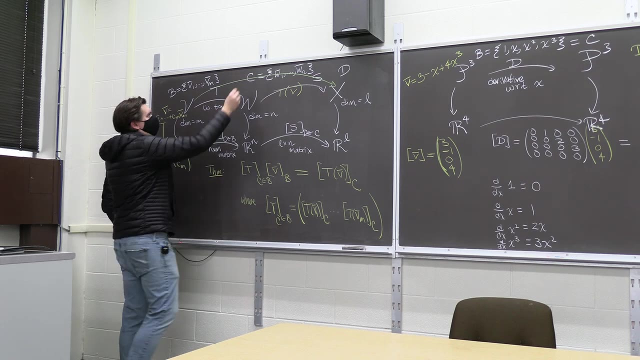 to x, And we might wonder like: OK, what's this? What should be the corresponding matrix down here? So up here there's a linear transformation that takes you from v all the way to x. You can achieve that by first doing t and then doing s, right? 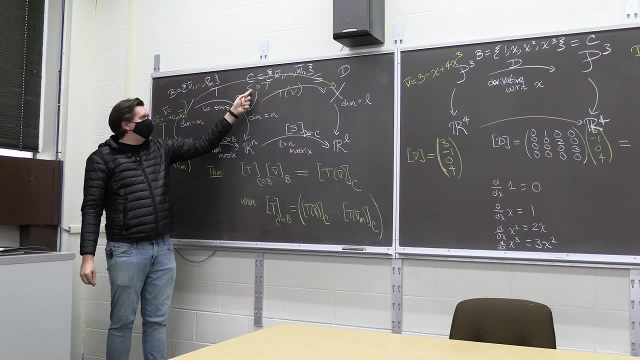 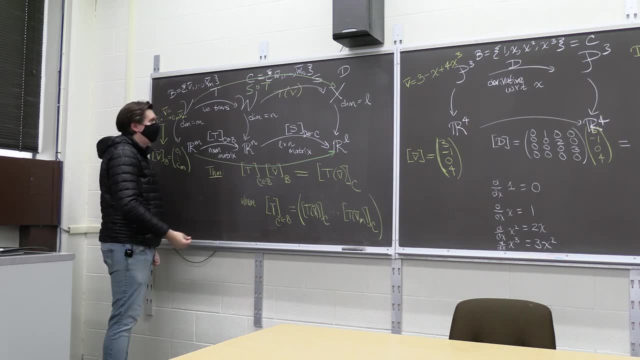 So, given some vector, you first apply t to it, then you apply s And it's like: OK, what should the corresponding matrix be down here We're out of space, but maybe writing in a new color lets you. It's like these old scribes. 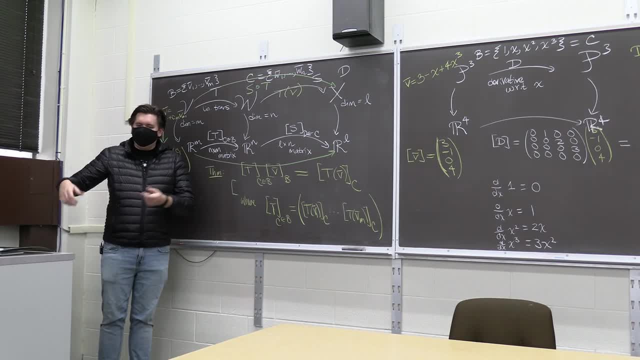 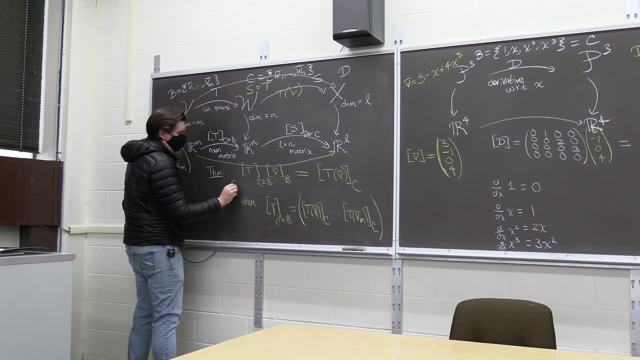 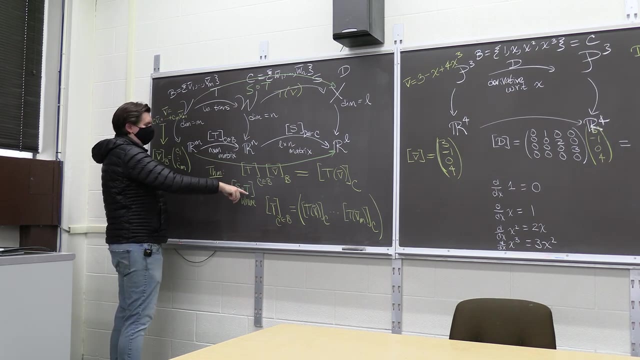 They would write on a text and when they ran out of paper they just rotated the text and wrote over it. I guess we're doing that right now. What matrix corresponds to s composed with t? What should that matrix be which is now going to be moving you from basis b to basis d? 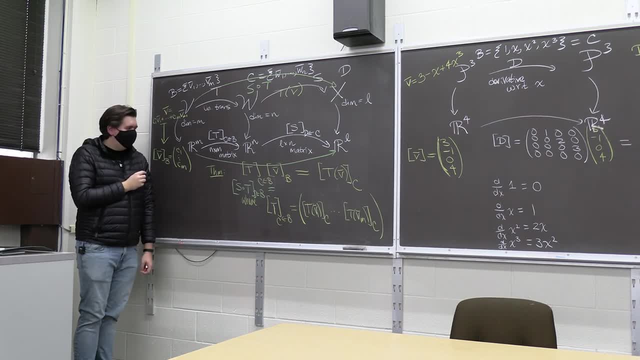 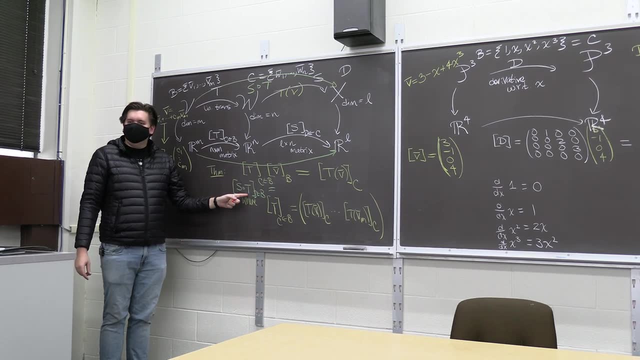 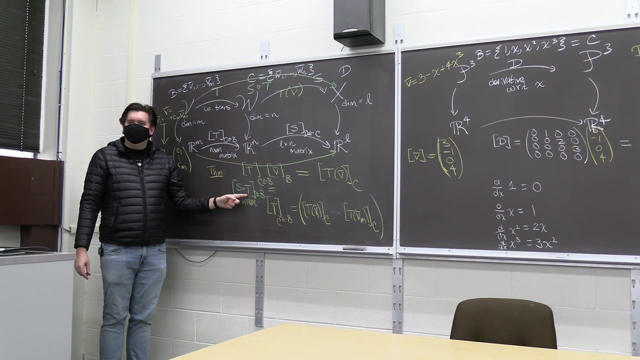 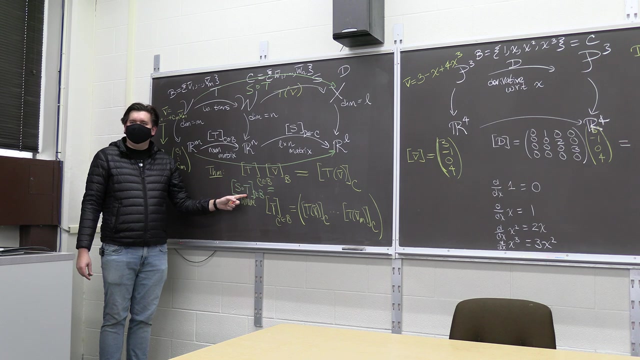 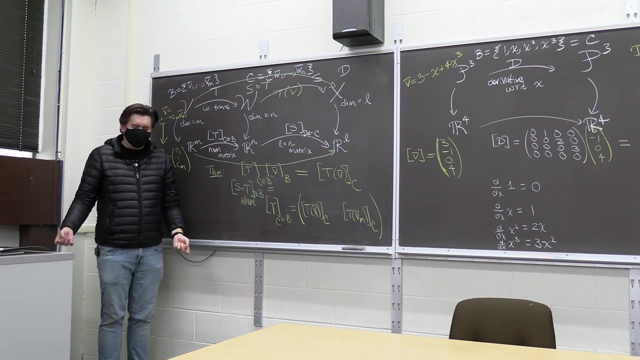 It's like: what is this matrix? Well, we already have a matrix here and we already have a matrix here, So any guesses on what this guy should be? Yeah, we just want to multiply these matrices right Now. we want to make sure we do the order of it correctly. 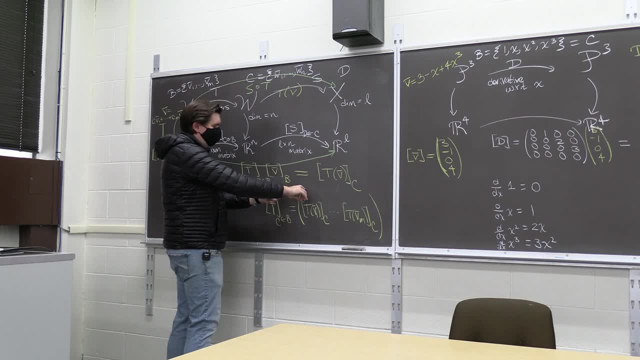 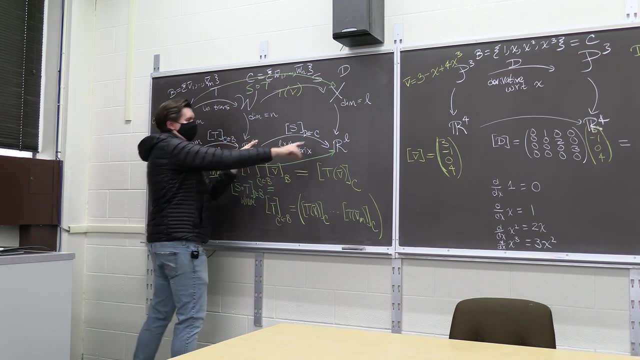 So the vector's going to be here on the right. You're first going to apply this matrix and then you're going to apply the matrix to the left. So what matrix should we apply first? Well, probably first the t matrix and then the s matrix. 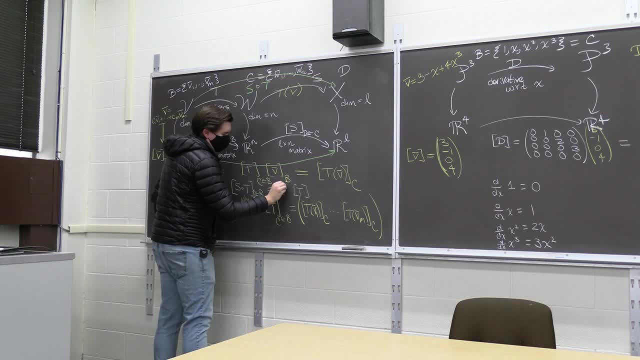 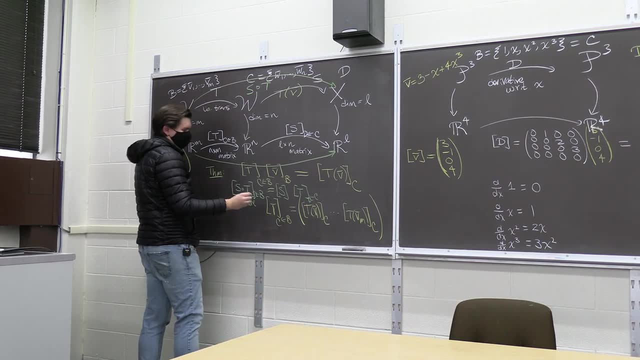 So the t matrix will be to the right and then the s matrix is to the left, And so this is our claim. We'll come over here and prove it here in a second, But hopefully from the picture, which is now quite convoluted. 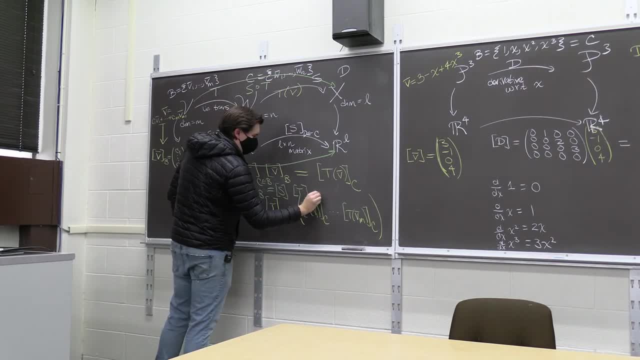 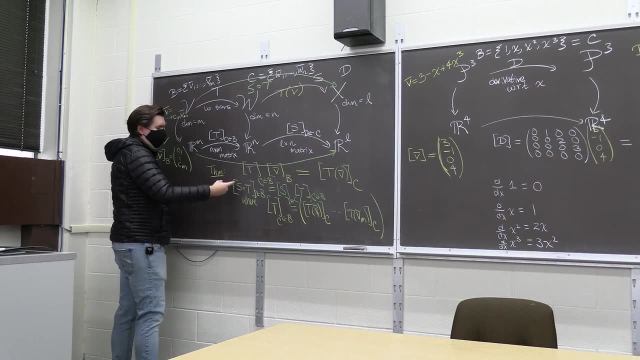 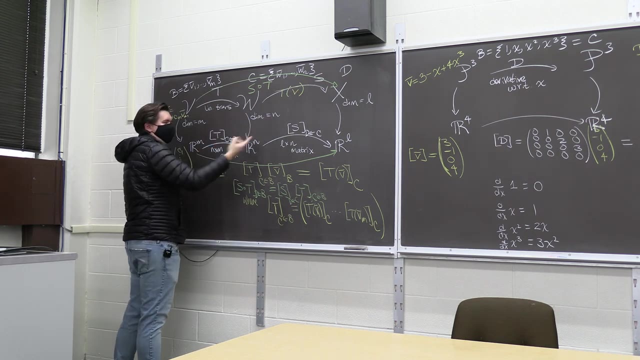 it's: t is going from b to s, b to c And s is going from c to d. The claim is the matrix that corresponds to the composition of two linear transformations is just the product of the two matrices for each part of the composition. 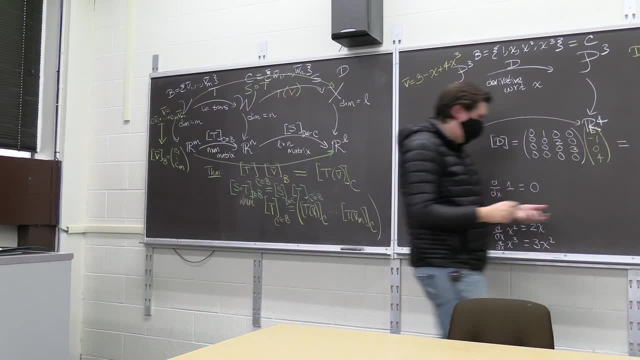 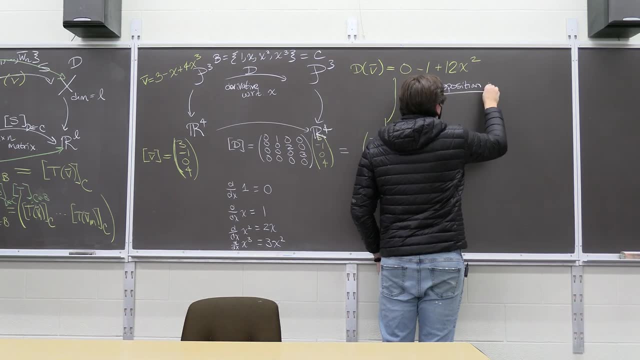 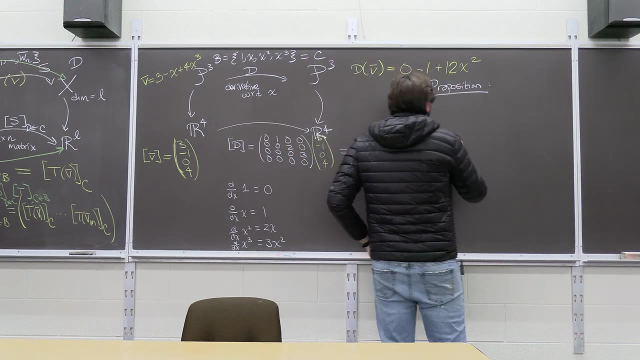 Yeah, so that's my claim. So I'm going to come over here and prove it. So here's my proposition. OK, I'm assuming the setup as before. I'm not going to write all of the v, w and x again. 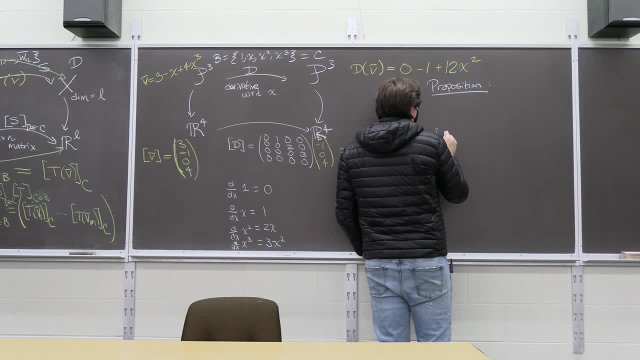 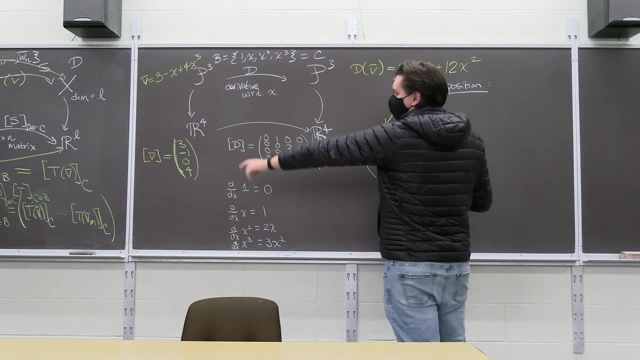 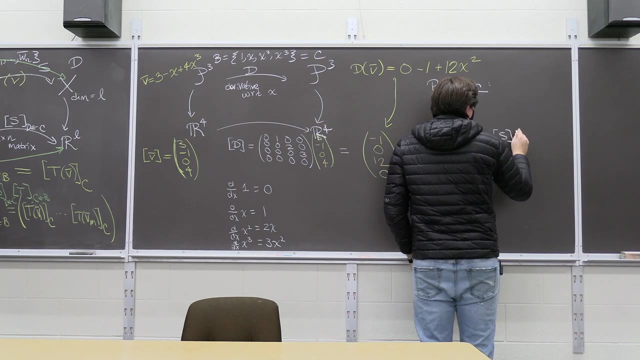 But I'm just arguing that my matrix corresponding to s composed with t, which is changing you from basis b to basis d, is equal to the matrix for s times, the matrix for t, where t was a matrix that moved you from basis OK. 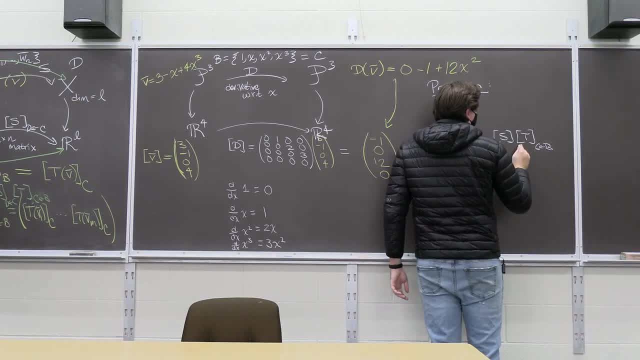 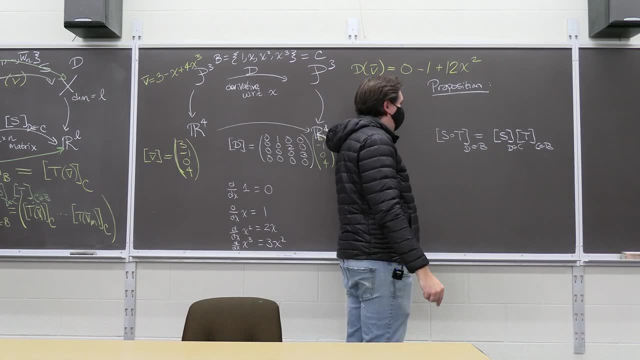 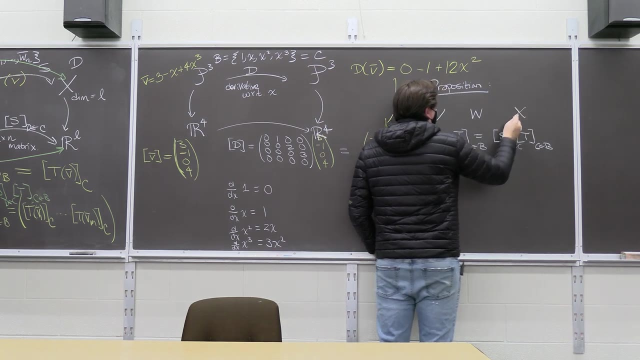 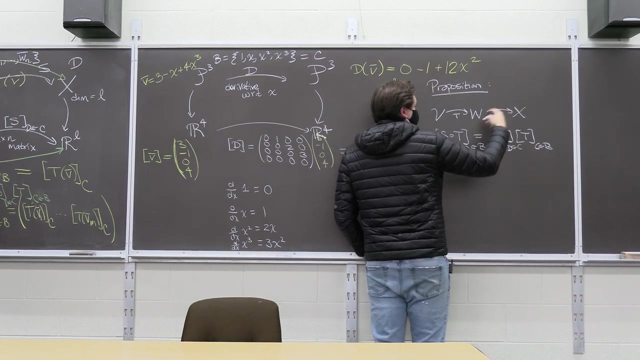 From basis b to c And s moved you from c to d. That's my claim. Well, let me just draw the picture a little bit to remind us. This is where we have vector spaces v, w and x. t was a transformation between the first two. 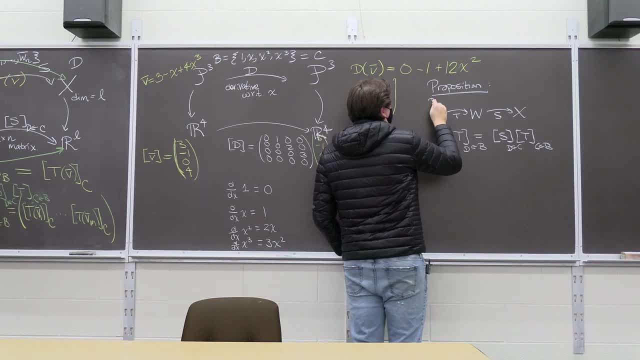 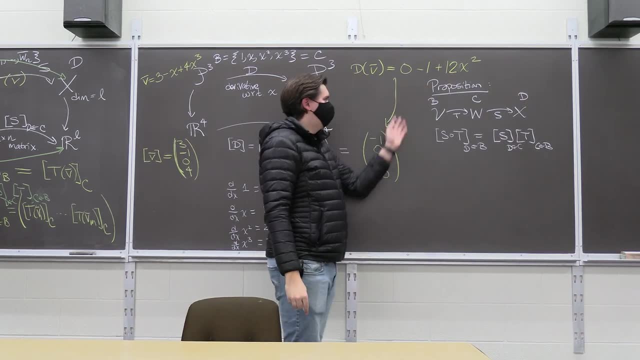 s were between the last two, And v had some basis b, v had some basis c And x had some basis d. So that's the setup. I don't want to write all the words, But we understand what this is saying. 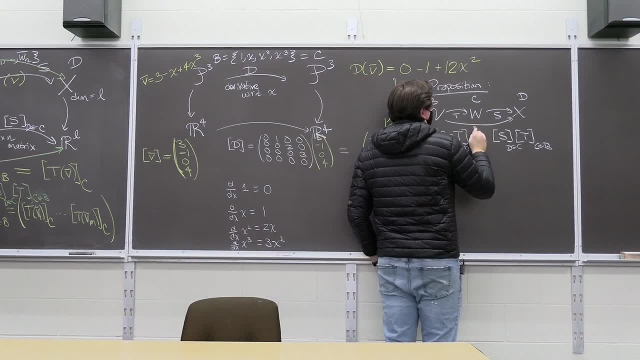 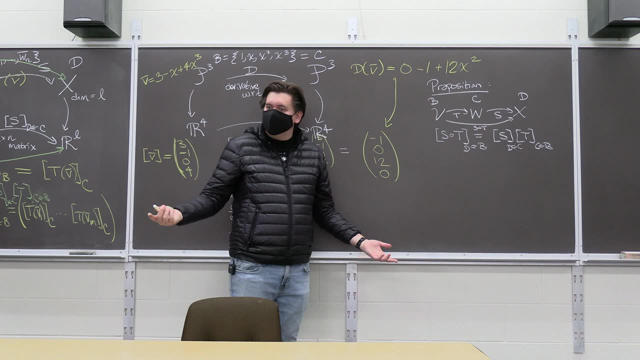 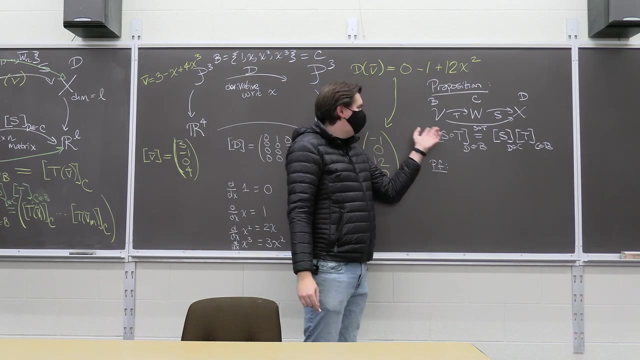 So we're saying something now about this composition. map s composed with t. OK, so let's try and prove this. It's like, well, it's kind of like, once you see the picture, like it should become sufficiently obvious. 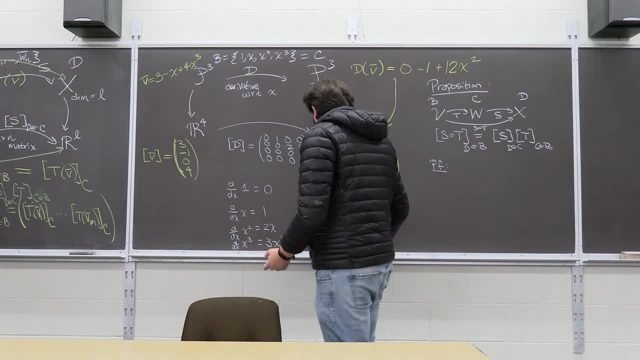 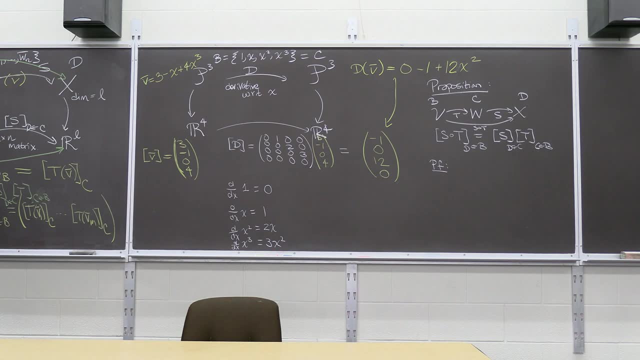 And you're like: what is there even to prove And how would you prove it? Well, the key way we're going to prove all these properties is we're going to come back to this theorem from last time, which is now covered with this green mess. 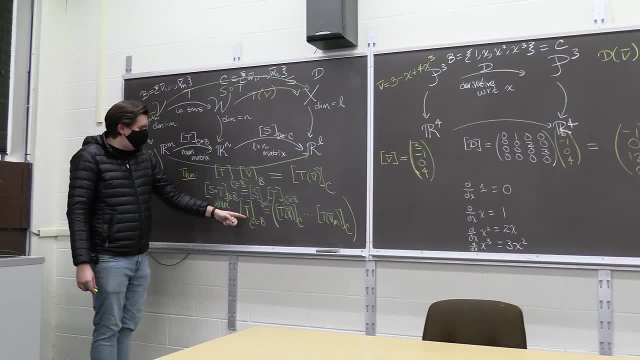 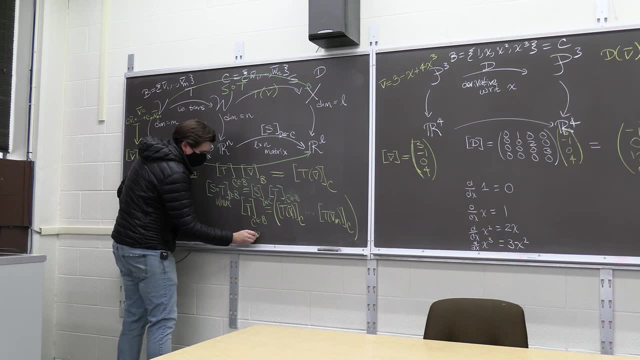 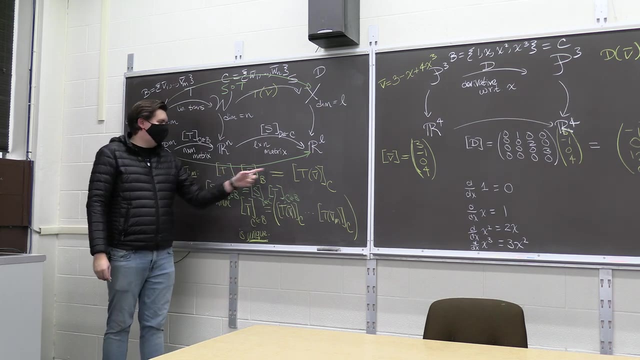 We're going to come back to this theorem, And this theorem gave us a formula for the matrix And it also told us that this matrix is unique. We stressed that last time. We proved it last time that this is a unique matrix that satisfies this for all v. 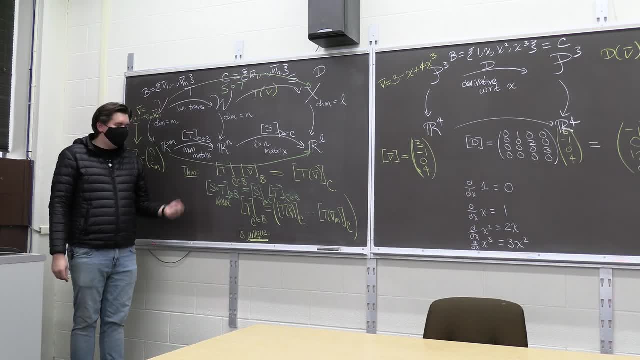 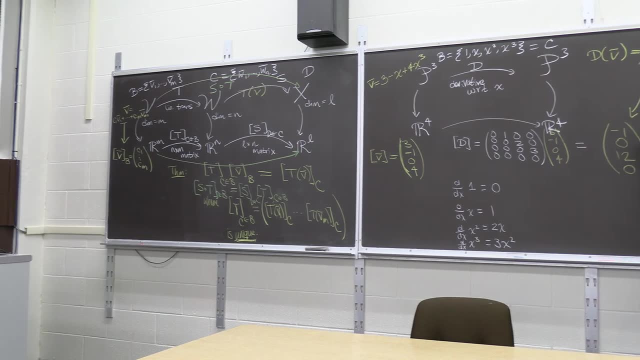 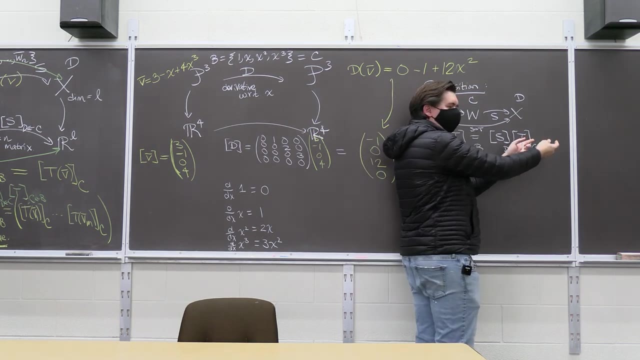 in your vector space, And so we really want to take advantage of that uniqueness In particular. I'm just going to show that this product of matrices does the same thing to vectors that the single matrix does, And since they both do the same thing for all your vectors, 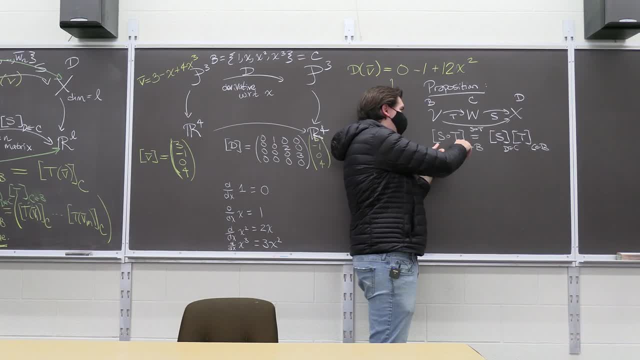 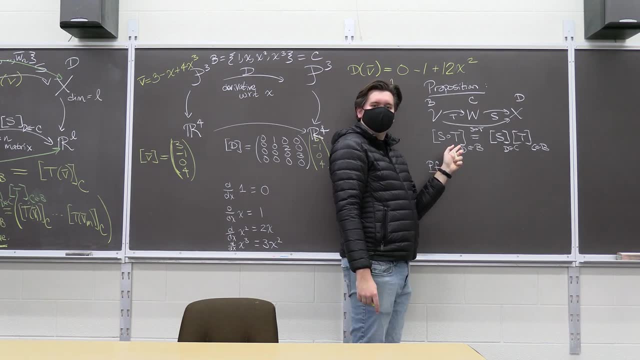 that means that they must actually be the same matrix, Because there's a unique matrix. There's a unique matrix that transports your vectors in v to vectors in x, according to the instructions of the linear transformation. That is all I need to do, is I just? 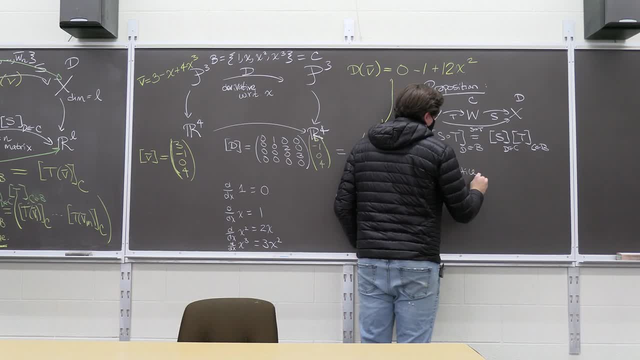 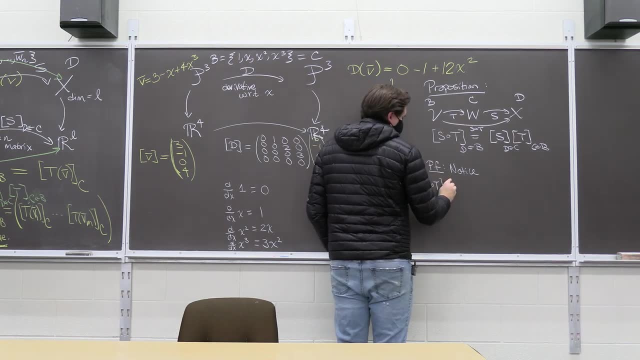 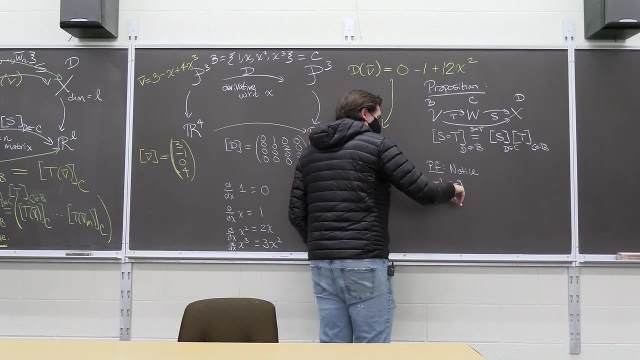 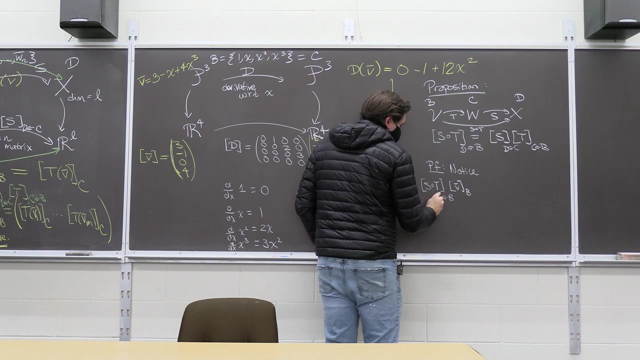 need to notice the s composed with t of some vector in v. I'm not going to always write my basis, But it should be clear which basis we're talking about. I'm in v, So I'm in basis b. This is a matrix that's going from basis b to basis d. 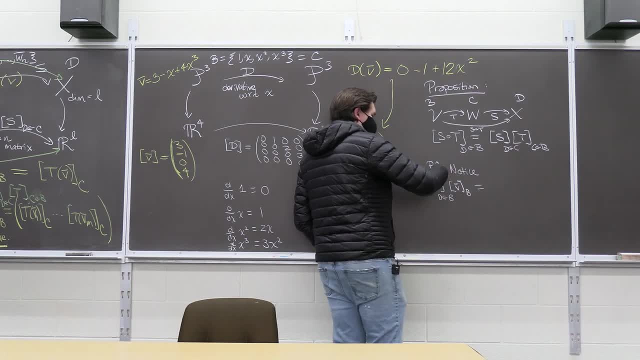 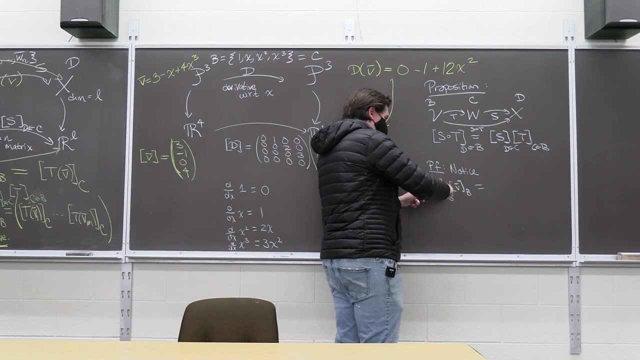 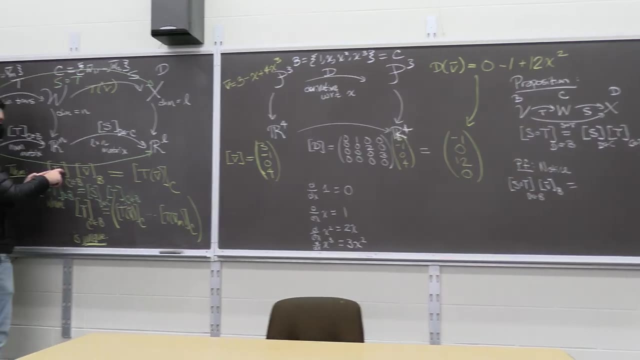 Maybe I will write them. What is this? What is this going to come out to be? Well, this is a linear transformation matrix times the coefficient matrix for a vector which, by a theorem, a linear transformation matrix times the coefficient matrix for a vector, is just the coefficient. 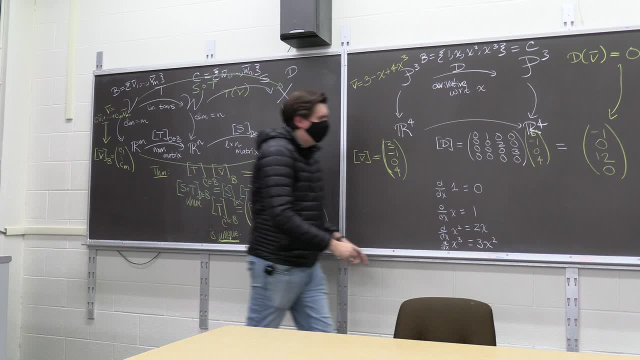 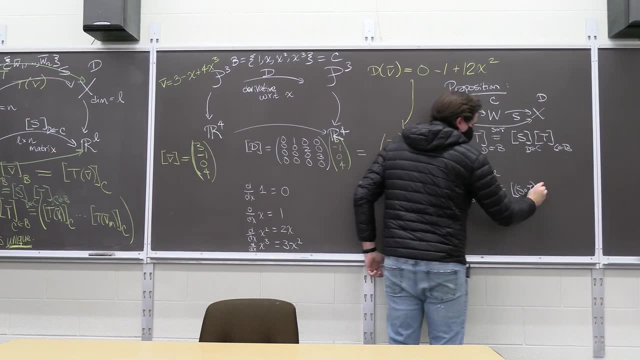 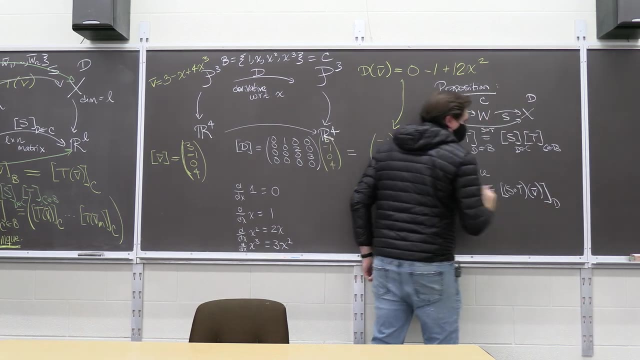 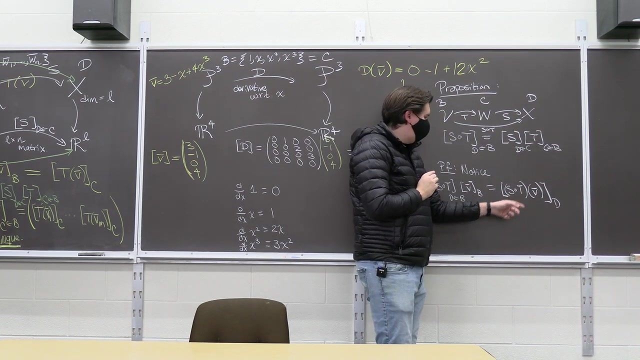 matrix of the linear transformation applied to the vector. So you just apply that linear transformation, as composed with T to the vector V, And now we're going to be living in X, so this is going to be in basis D. But what is S composed with T? 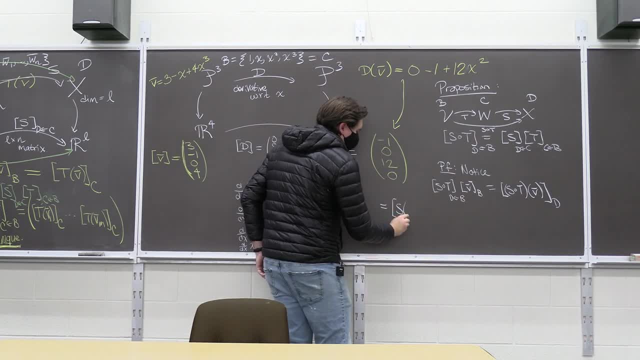 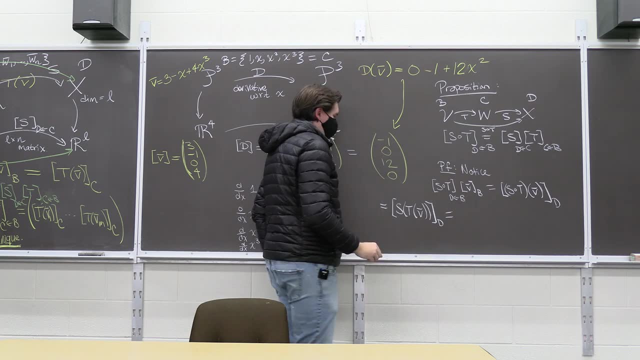 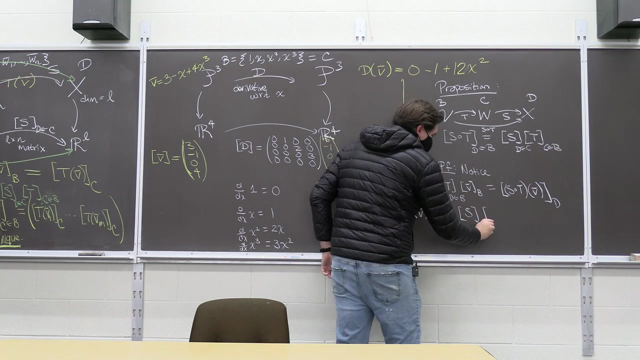 That's the same thing as just S of T of V, But this is the linear transformation S applied to T of V. So by our theorem that's the same thing as the matrix corresponding to the linear transformation of S times the matrix for T of V, the vector. 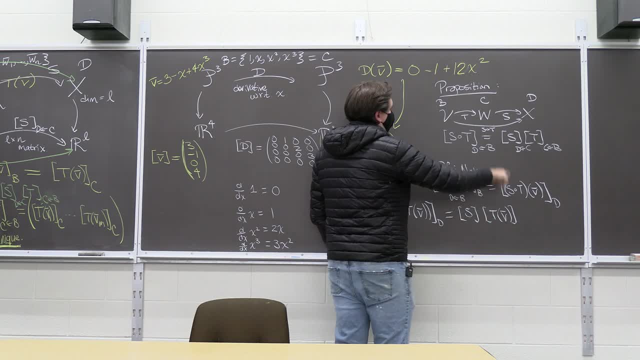 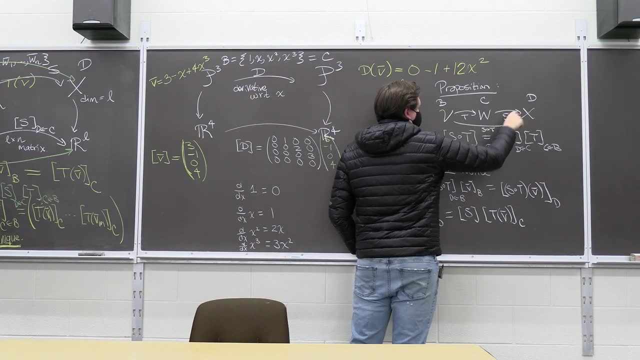 the coefficient vector of T of V, So this is now some coefficient vector. This lives in W, so this is in terms of C, And your matrix for S is a matrix that's taking you from W to X, So that's from basis C to basis D. 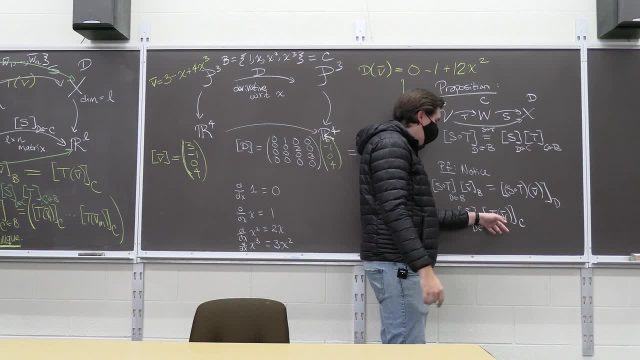 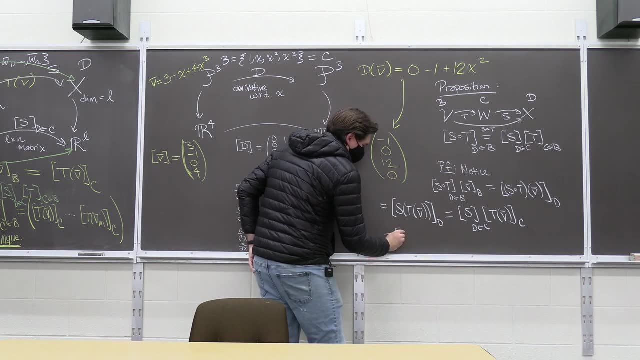 But then by another application of the theorem T of V. that's just some linear transformation applied to the vector V. So that's just going to come out to be the matrix corresponding to the transformation T times the coefficient vector of T of V. 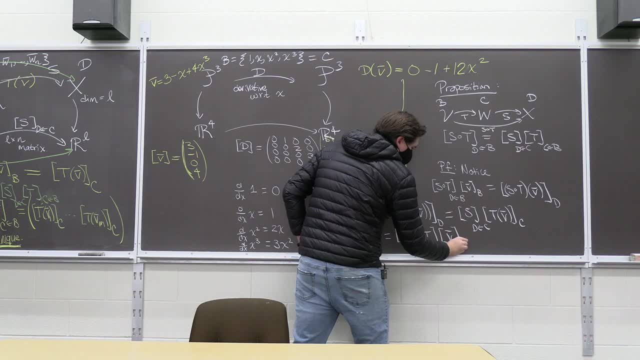 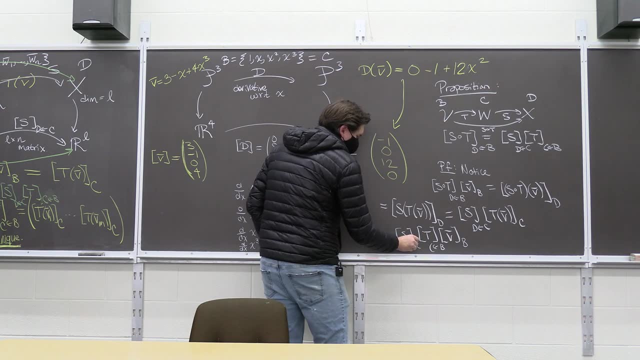 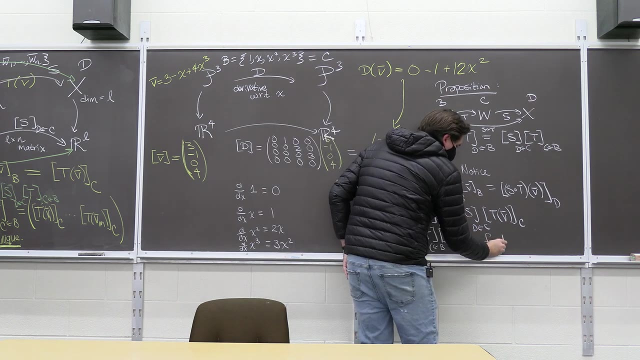 So that's just going to be the coefficient vector for V. Well, this is in terms of B, This is a map from B to C, And this is a map in terms of basis C to basis D. And now this is true for all V in your vector space. 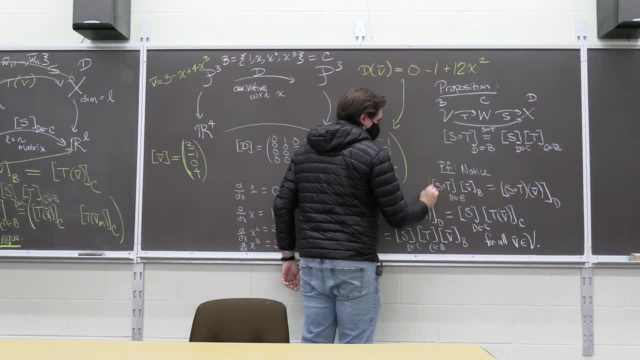 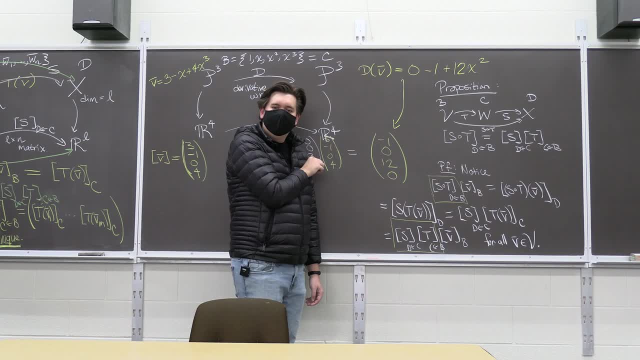 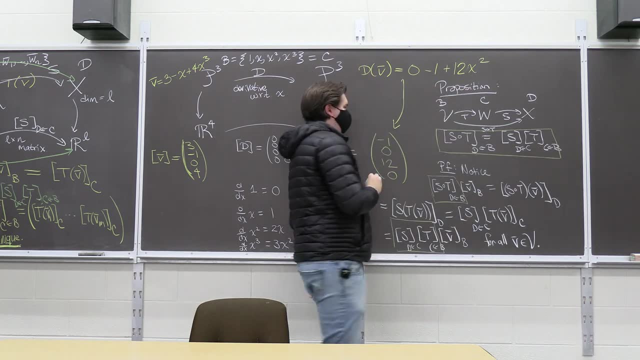 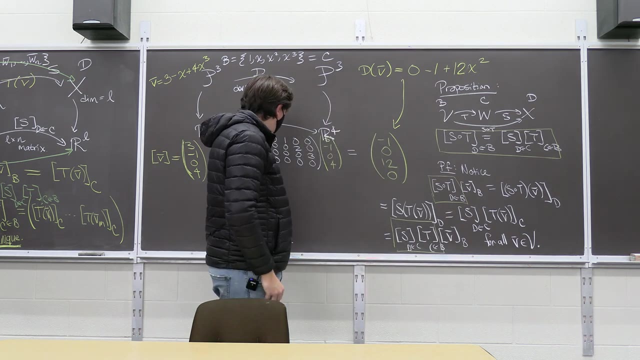 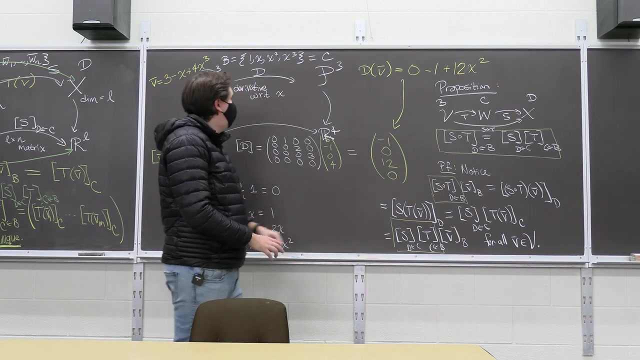 of those two matrices for any vector V. Thus, by uniqueness, they must be equal to each other. This matrix must just be the product of those two matrices. So to think about a really quick application of this, let's go back to our concrete example here. 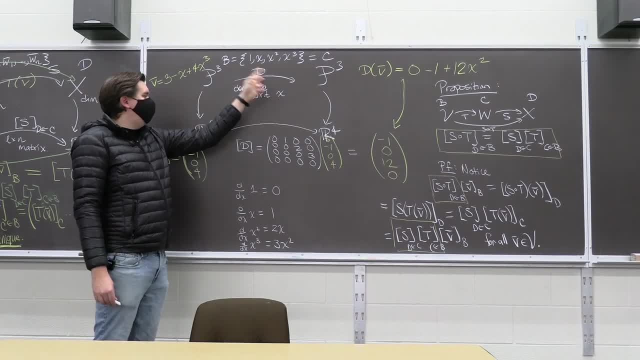 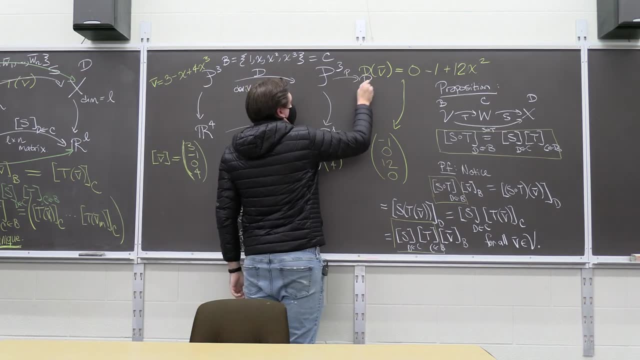 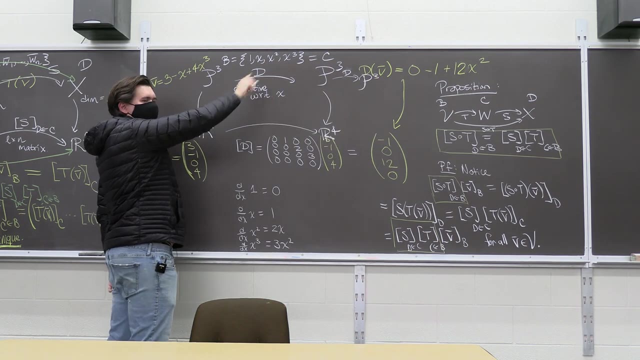 Let's look at the question. You can imagine taking a derivative once as a map from P3 to P3.. You can also take the derivative again as another map from P3 to P3.. So you can do the derivative however many times you want. 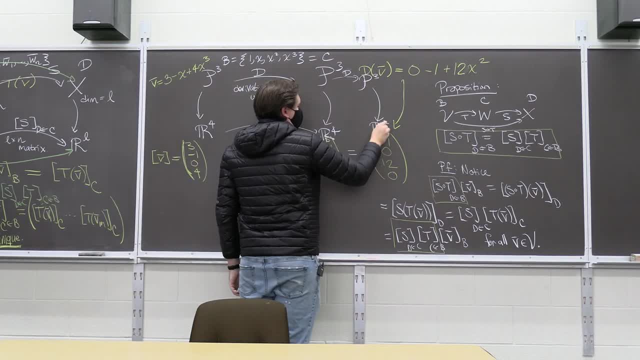 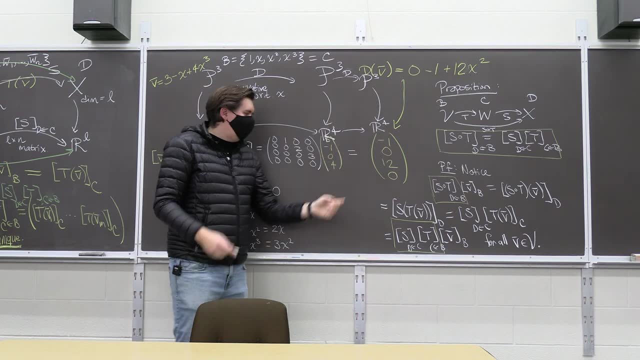 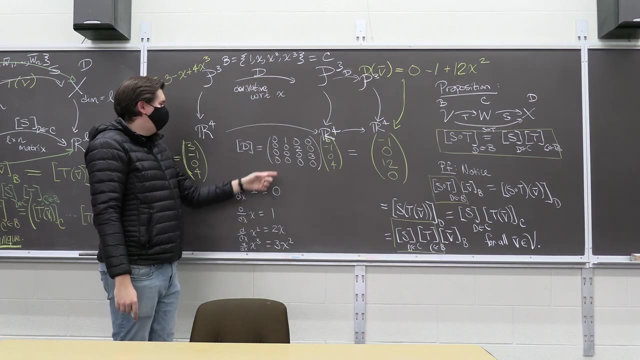 And you know this also corresponds to something down here in R4.. And then the question is like: taking the derivative twice, taking the derivative twice corresponds to what matrix? Well, taking the derivative twice should just correspond to this first matrix times the second matrix. 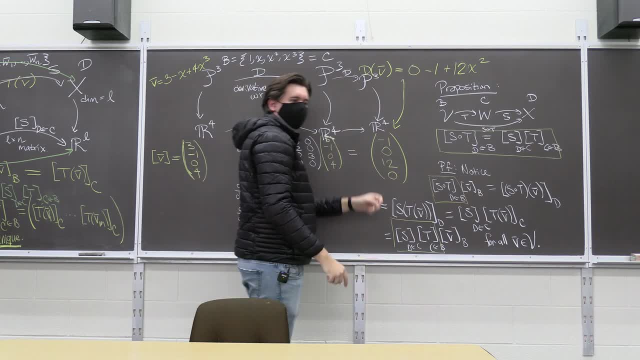 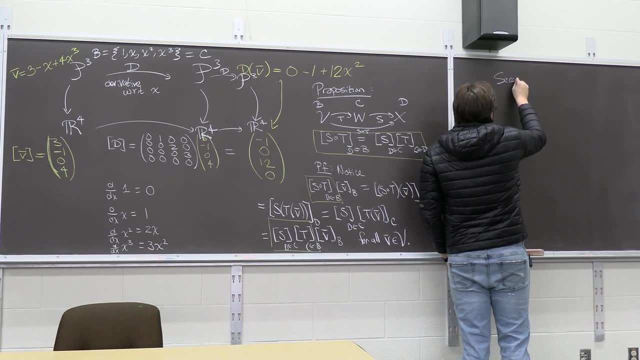 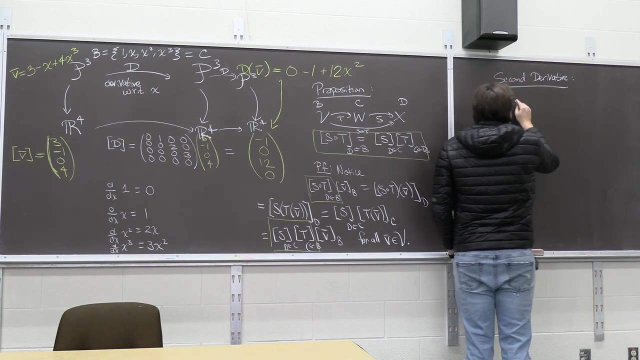 which would be the same matrix because it's the same linear transformation. Hence, if we want to find what is the matrix corresponding to the second derivative, that is, what is the map corresponding to D squared, which is just D composed with D. 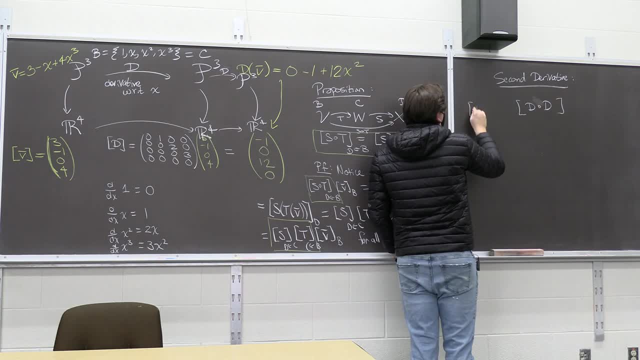 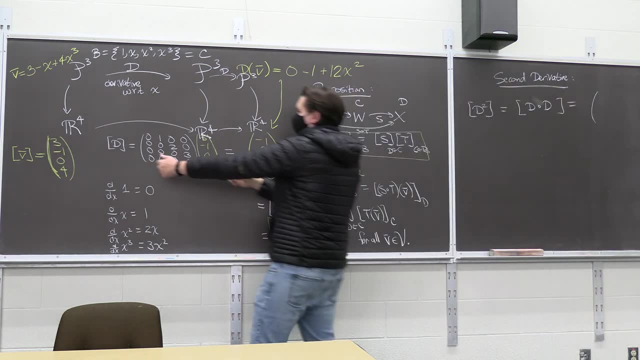 What is the matrix corresponding to that? I'll often denote this by just D squared. It's just going to be your original matrix times. whatever the next one is these two times together, but they're both the same matrix. So if we want to find the derivative, 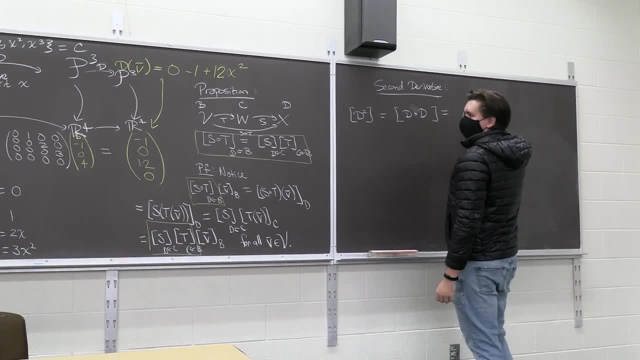 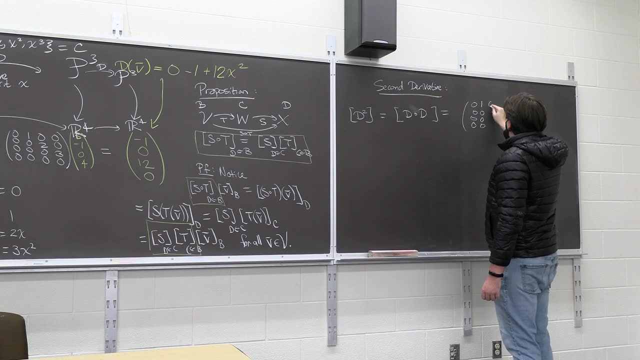 so it's just going to be that first matrix squared: 0, 0, 0, 0, 1, 0, 0, 0, 0, 2, 0, 0, 0, 0, 3, 0,. 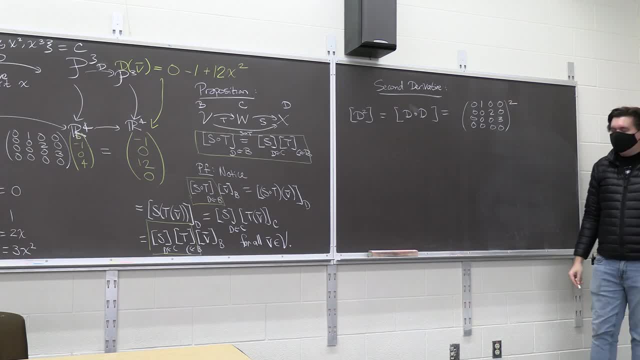 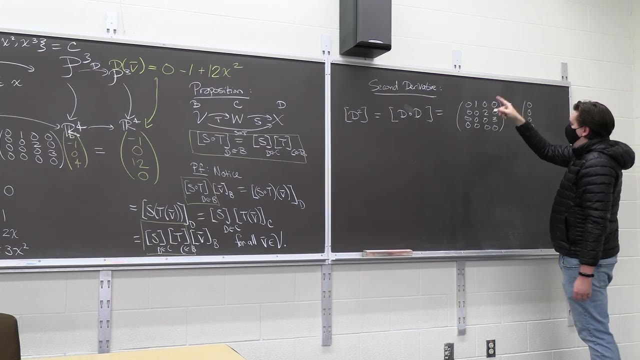 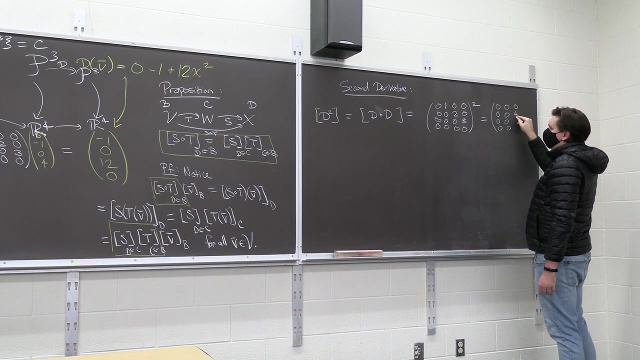 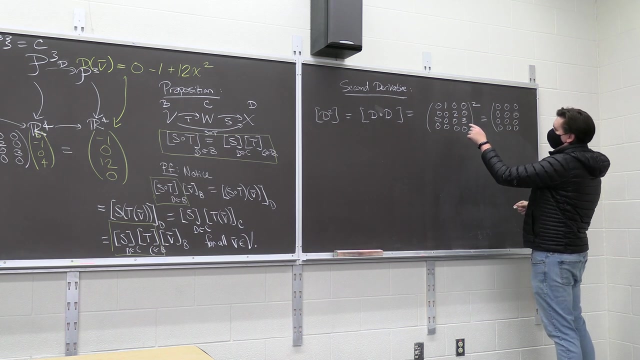 that guy squared. And so what is that guy squared? That guy squared rho times. row times column. row times column. do row times column? I think we get a 4 here. No, Are those all zeros? Does any row that's not zero? 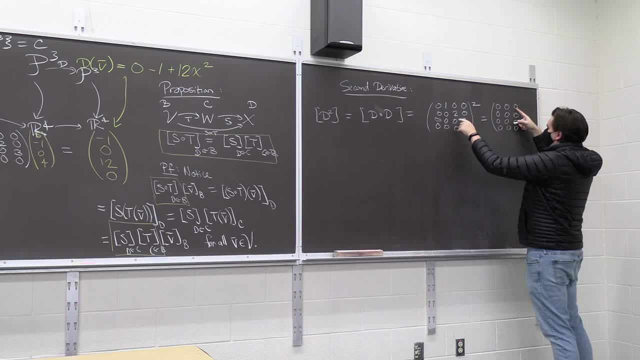 Right here, Row times column. Very good, There's a 2 there, Because this row times this column would give you a 2.. And any other non-zero values. This row times this column would give you a 6.. Second row, last column. 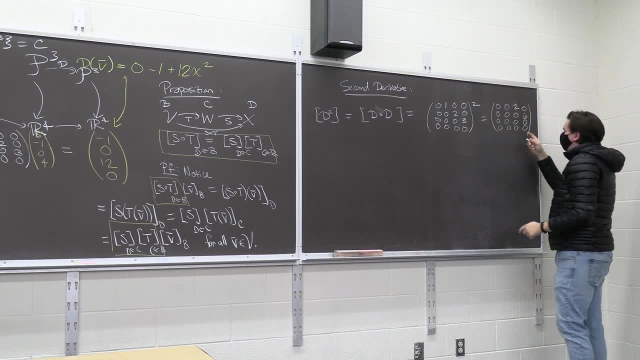 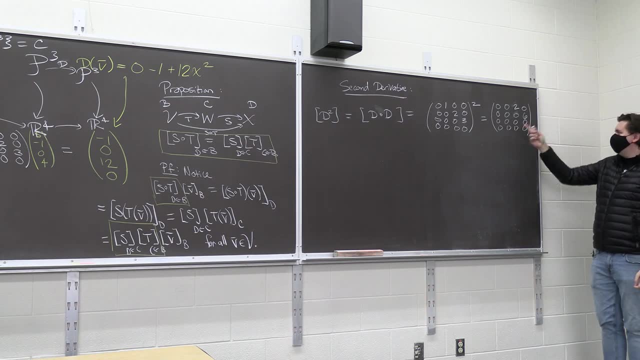 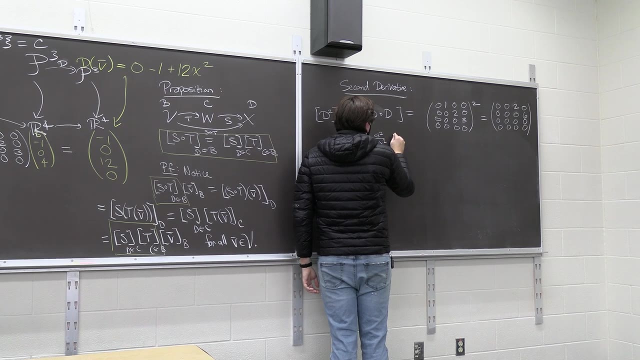 gives you a 6. That corresponds to your second derivative. It's like: why is that the matrix for your second derivative? Well, what is your second derivative of? And we can go through and do all the different values We can feel. what is it of 1?? 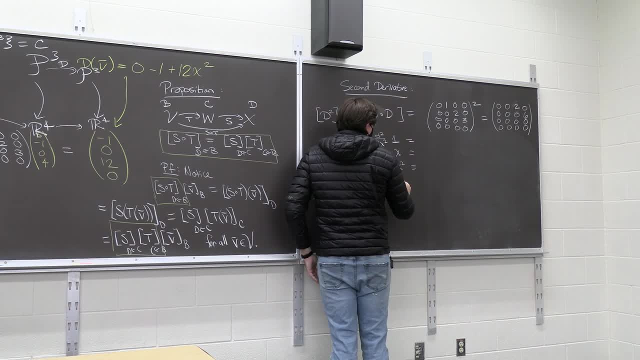 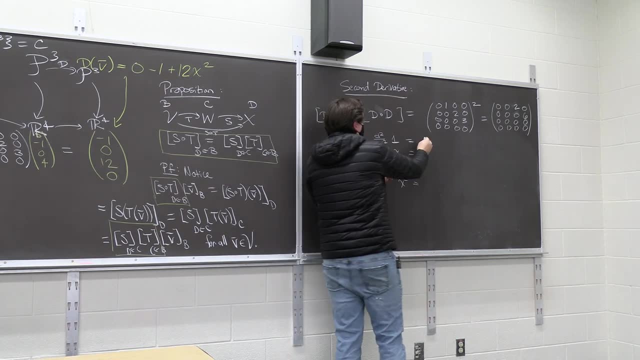 What is it for x? What is it for x squared? What is it for x cubed Right, taking the second derivative for all of those? So for 1, it's just 1.. For x it becomes 1, then it becomes 0.. 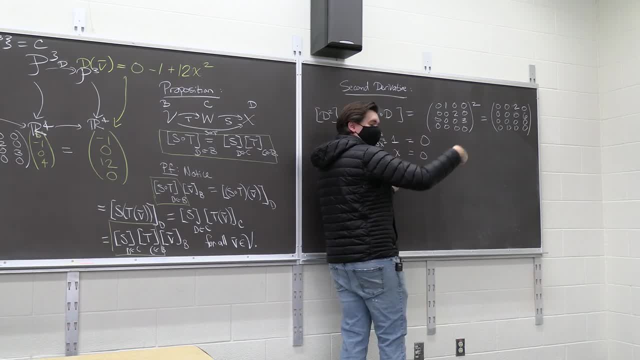 I'm sorry. for 1, it's 0.. For x, it becomes 1, then it becomes 0.. For x: squared, it becomes 2x and then it becomes 2.. x- cubed, it becomes 3x. squared, and then it becomes. 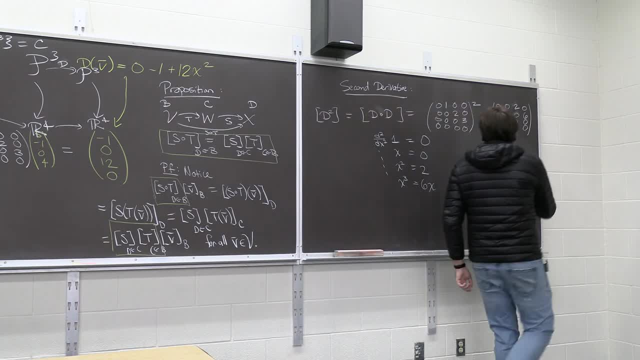 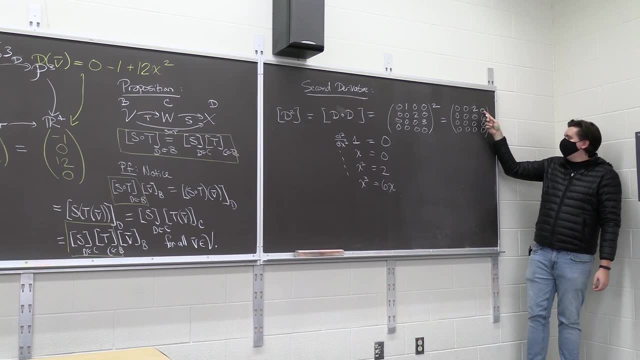 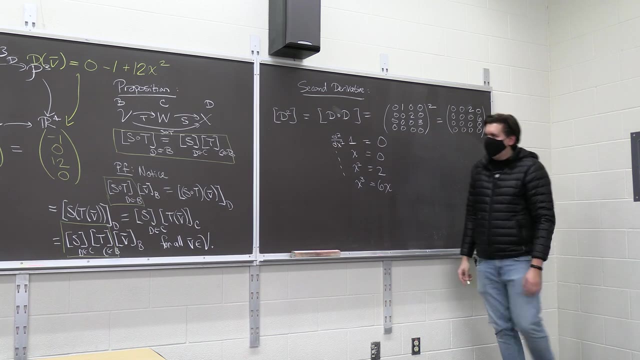 6x, which exactly corresponds to this matrix. For x squared, it was 2.. For x cubed, it's 0 copies of the constant, 6 copies of x, 0 copies of everything else, And if you took our original vector here, 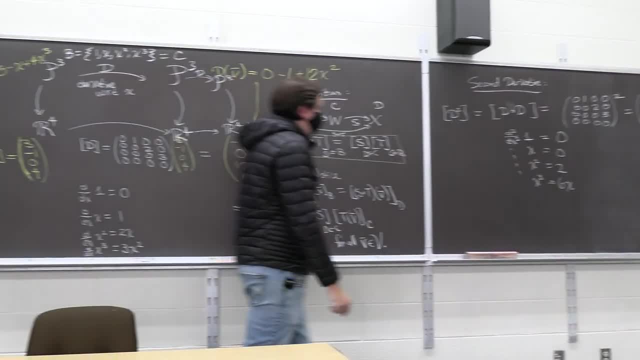 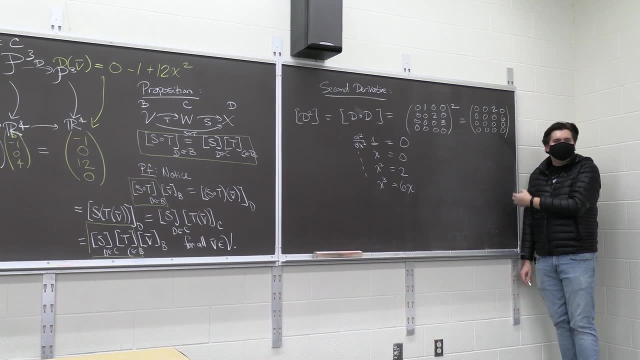 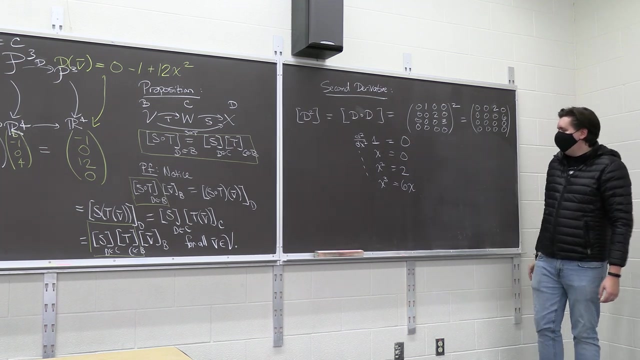 v and you would multiply it by this matrix, you would figure out what the second derivative is, And you can keep doing this. If you want to know what the third derivative is, you can do d3, it will be whatever the matrix was for d. 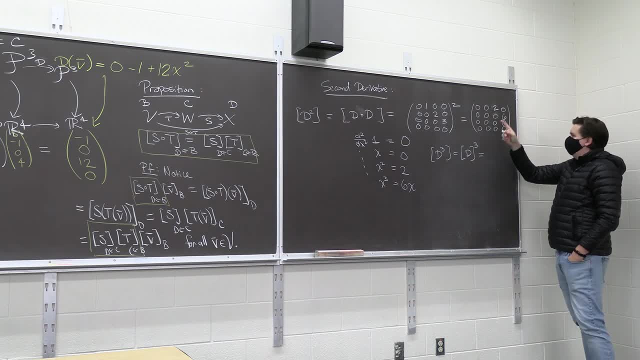 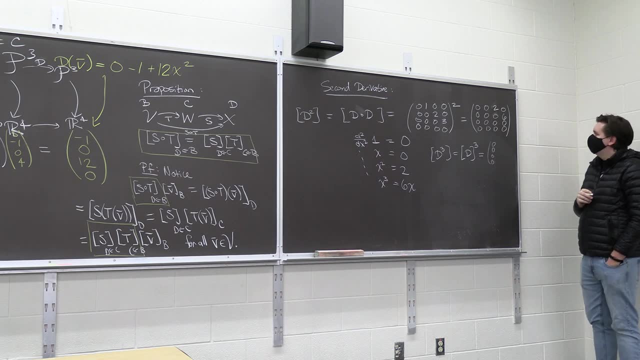 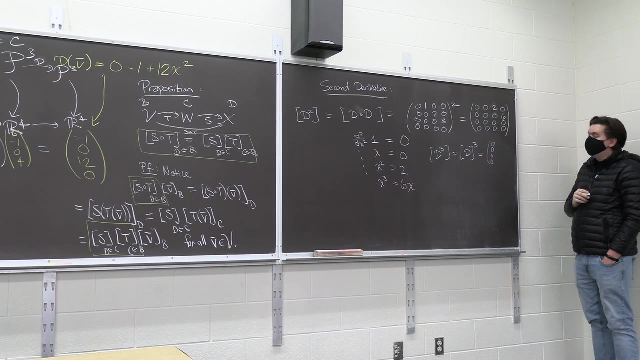 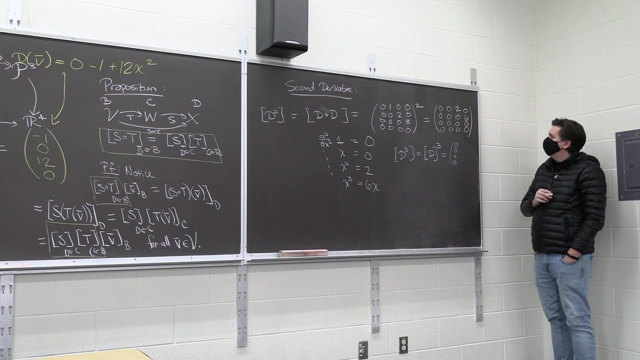 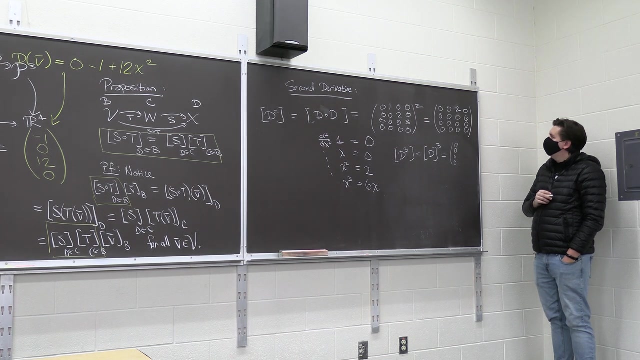 cubed, and so you can do the same thing. row times column: Now it really is almost all 0s, whereas the only place you don't have a 0.. Do we see it? Maybe that is a 0.. Maybe that is a 0.. 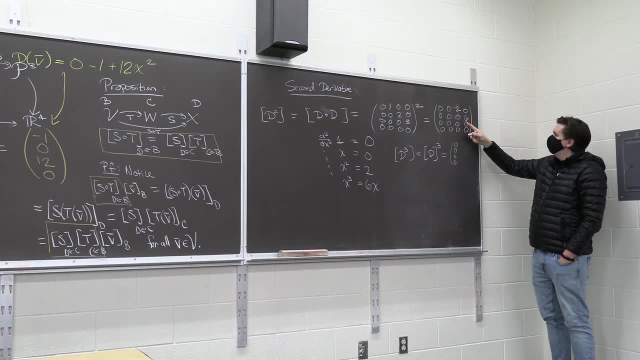 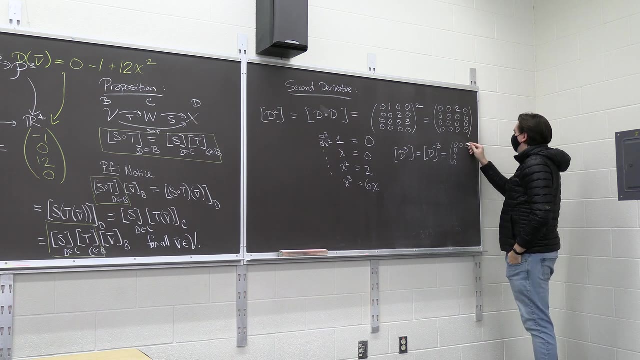 Did I do this one wrong? This row times this column. Oh duh, this guy times this guy. So this row times this column gives you a 6 up there. Very good, very good, Very good. These guys are great. 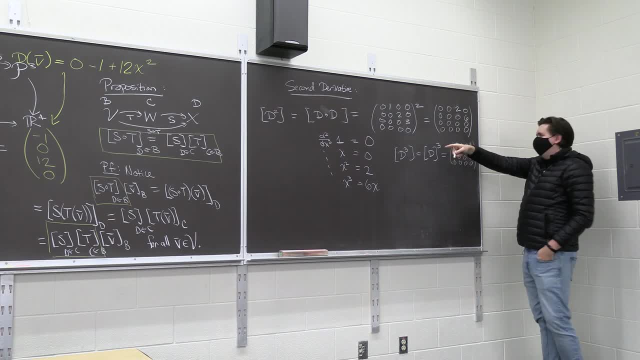 Gives you a 6 up there. I was doing d4, which would be this guy times himself, But the original guy times him- will give you a 6 up there, And if you did d4, you would see you end up with just the. 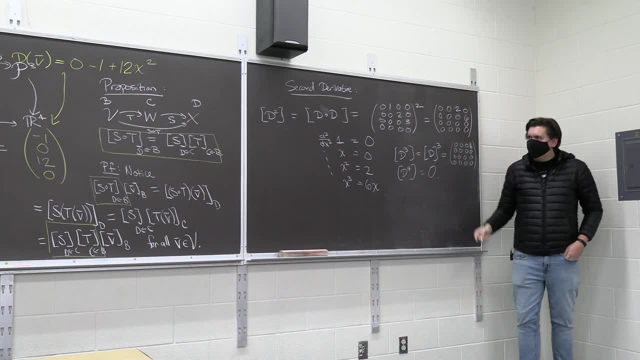 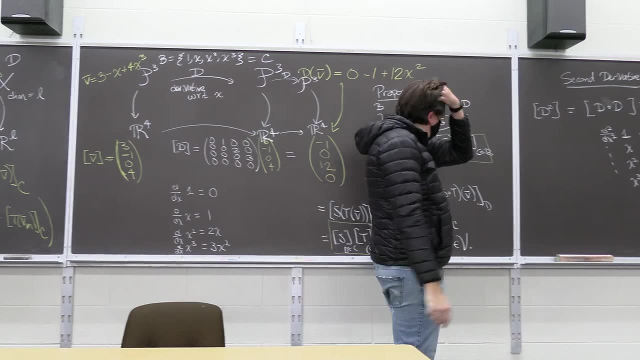 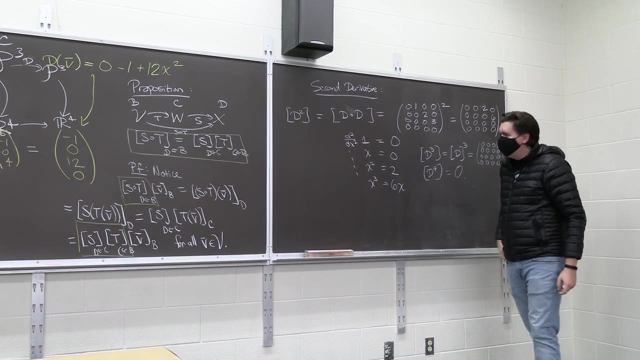 0 matrix, Which makes sense, because if you do the fourth derivative of anything in p3, you'll end up with just 0.. Okay, so is this making sense? Are you happy? Is this good? Well, I guess I want to say one more thing now. 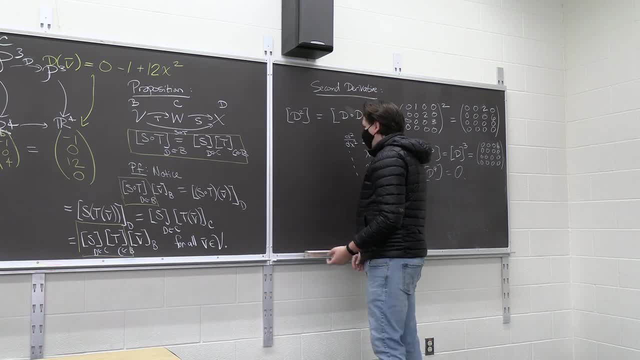 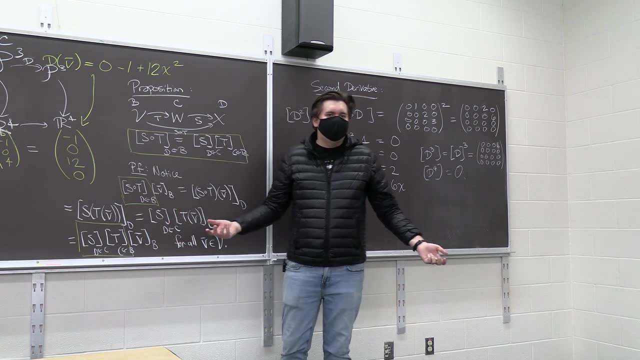 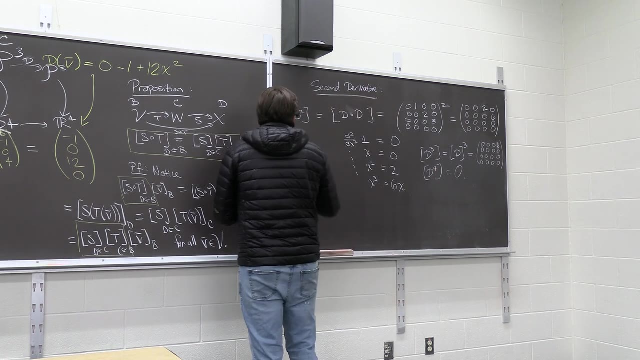 A similar proposition And that's like we can do. composition. What's another kind of thing you might want to know about Inverses? So let's say we're about inverses, So let's see if I can fit this in here. 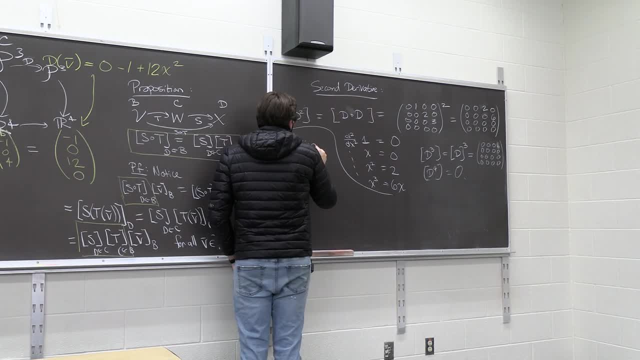 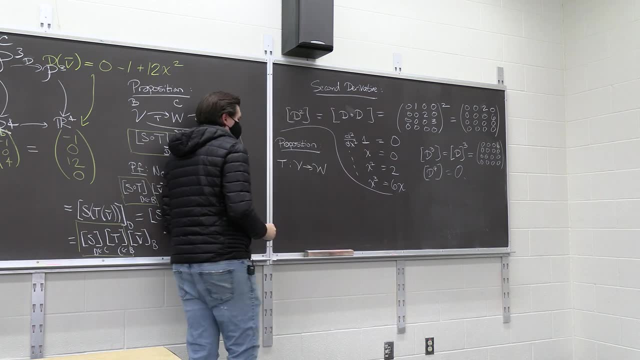 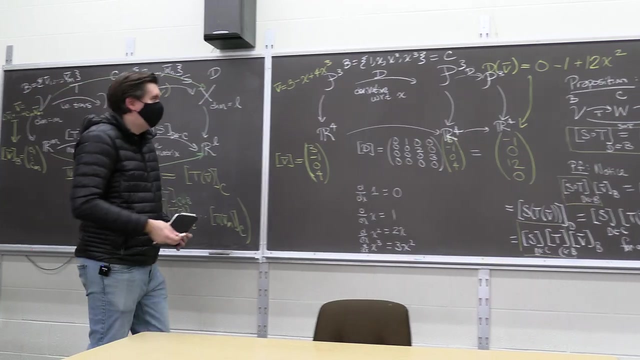 So proposition Like say, t is some linear transformation from v to w And suppose it is invertible. Now it may not be the case that your linear transformation is always invertible. Can you think of an example of linear transformation that's not invertible? 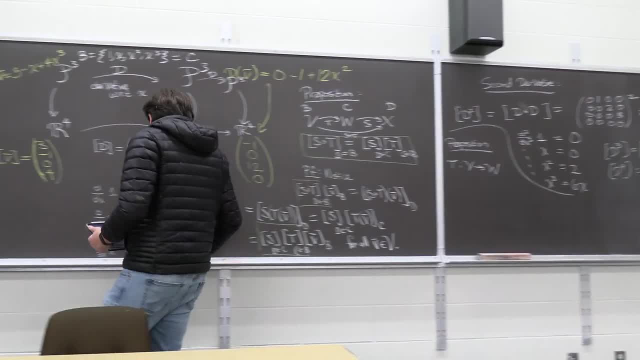 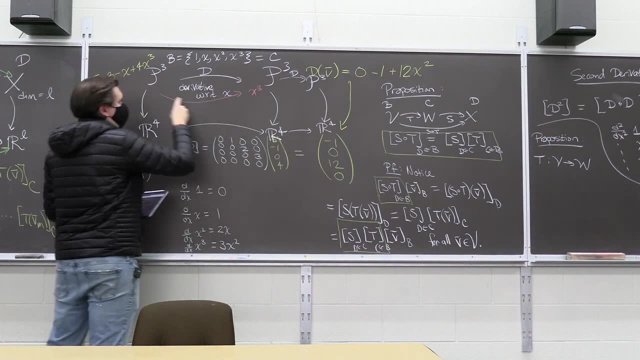 What? This one? It's like what gets sent to x cubed, Right, like what would get sent to x cubed. And you'd be like, well, the derivative of what is x cubed. And you want to say it's like. 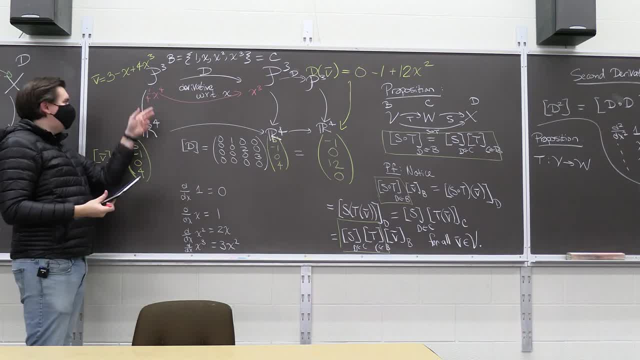 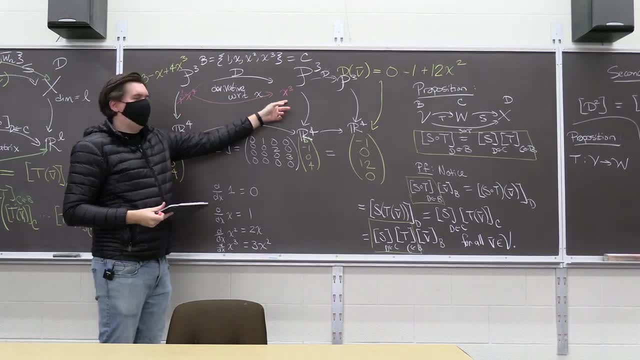 1. fourth x to the fourth right, But that's not a thing that lives in p3. So we can't say that. So nothing gets sent to x cubed. So we can't invert this Because, like you know, the guys 1 through x. 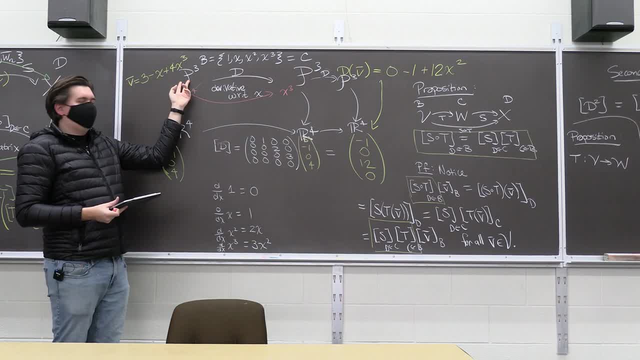 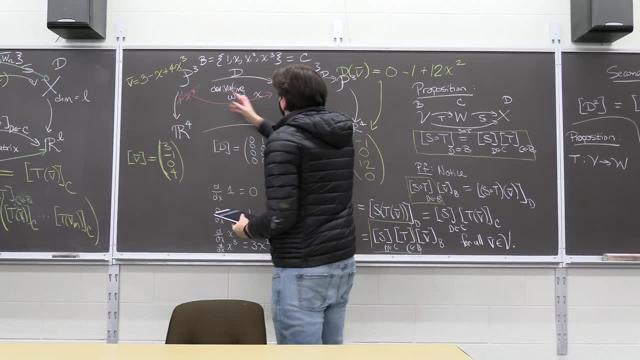 cubed. they don't all have inverses when you just restrict yourself to p3.. So this is not invertible. But we want to say like sometimes it is And it's like: why isn't this invertible? Well, look at its. 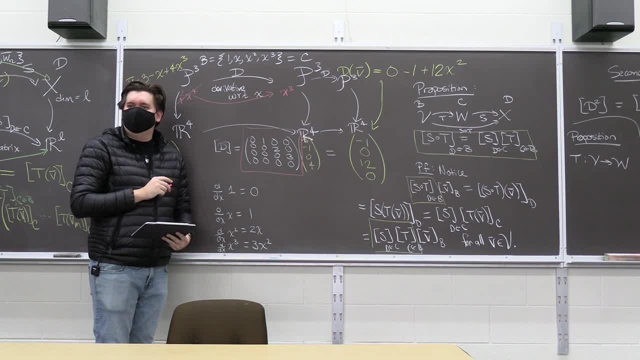 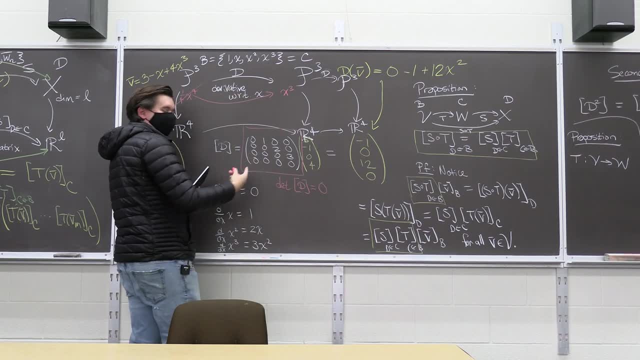 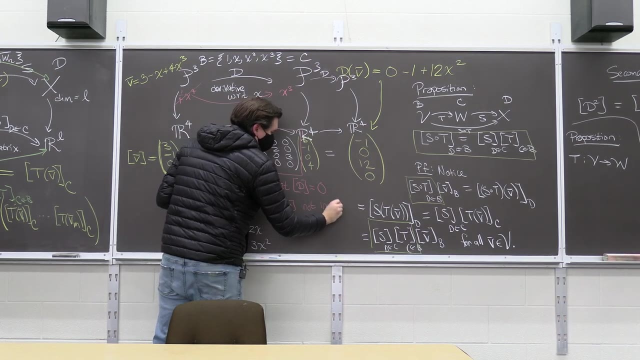 matrix. What do you notice about this matrix? Good, The determinant of this matrix is 0,, which means the matrix is not invertible. This guy d is not invertible And our linear transformation is not invertible, So it seems. 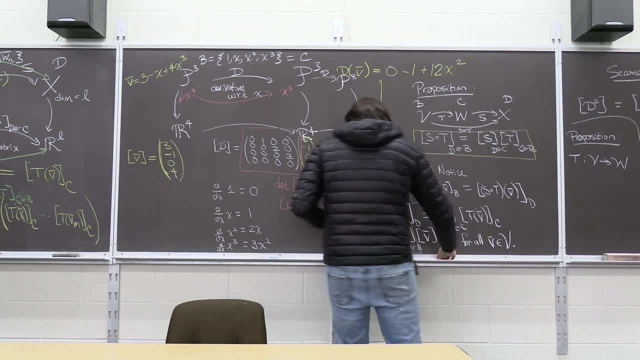 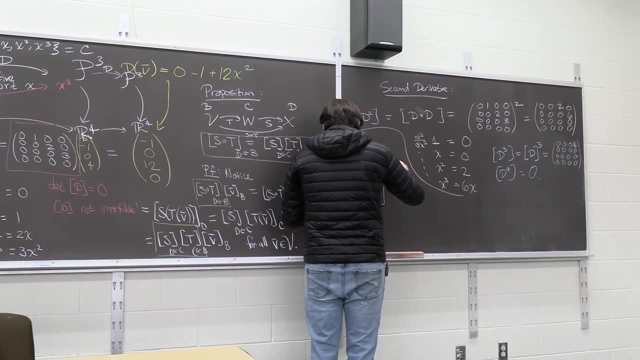 like these things are tied together And that's exactly what we want to say. So let me make sure I get the wording of this right. We're going to say that t oops, I guess I'll give you a definition. So first let's define. 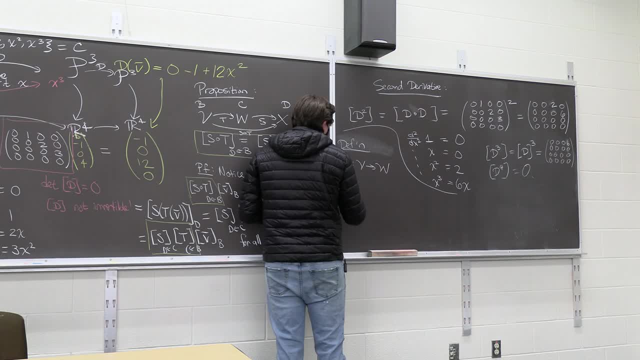 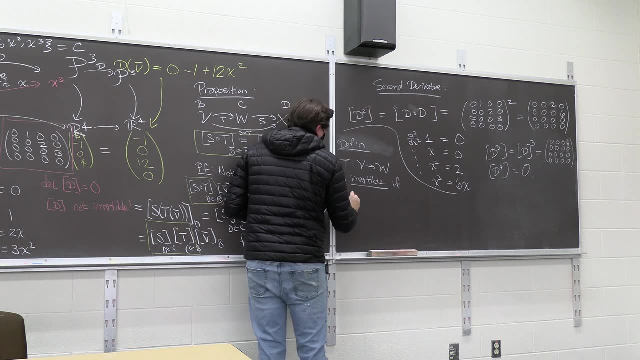 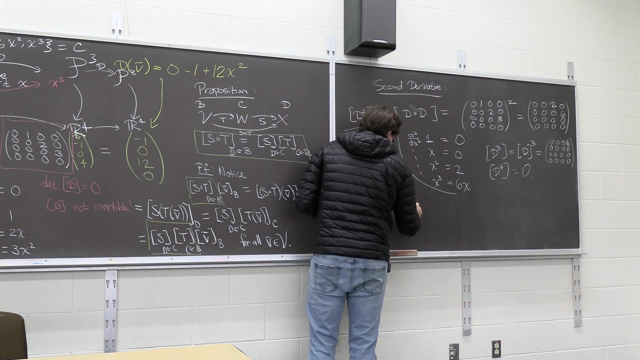 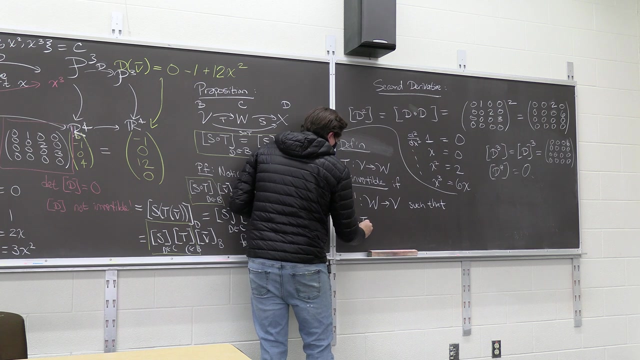 we're going to say that this linear transformation is invertible. Like what does it mean to be invertible? It means that there exists some inverse map, t inverse, a linear transformation from w to v, such that if you compose t with t inverse. 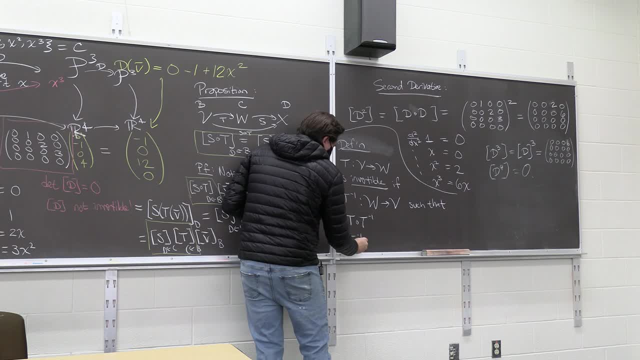 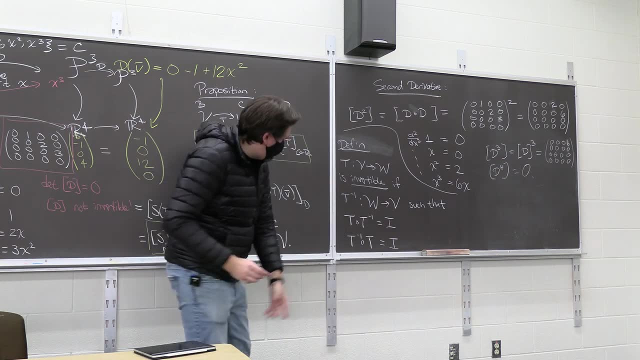 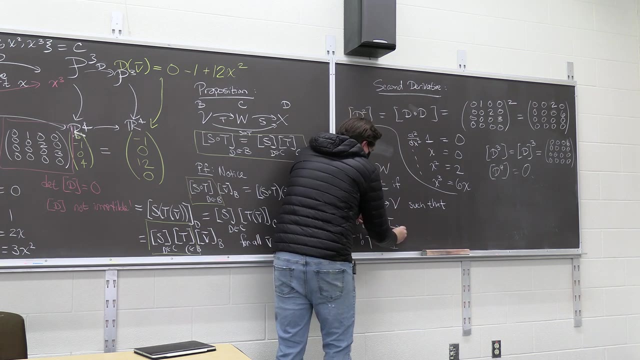 or you compose t inverse with t, you'll just get the identity map on. well, let's think about it. If I do t inverse composed with t and start off at w, I go to v and then go back to w. that's the identity map. 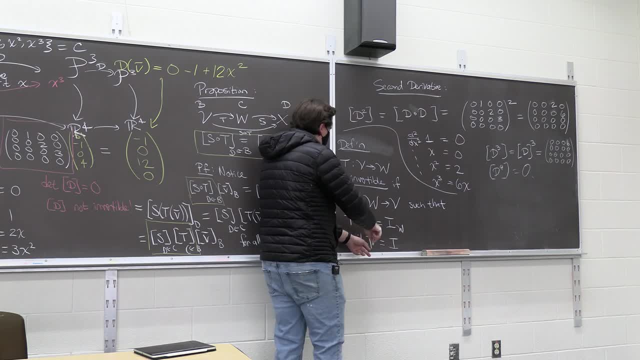 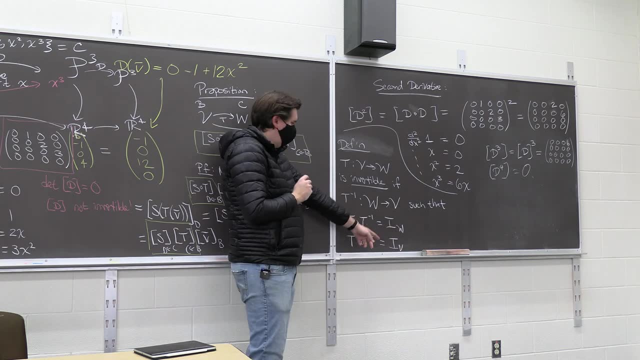 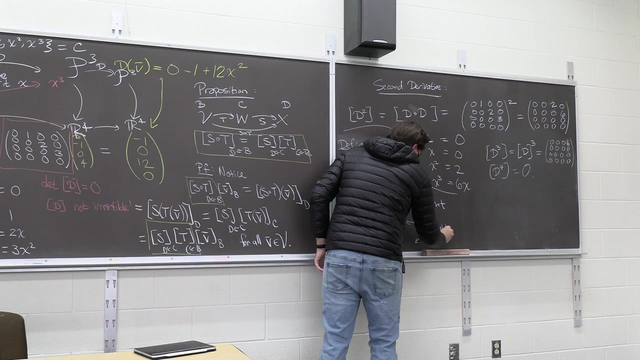 on the vector space w. if I do t inverse composed with t, I start off from v, I go to w, I go back to v. so this is the identity map on v. So this is just identity. No, the identity map is a linear transformation right. 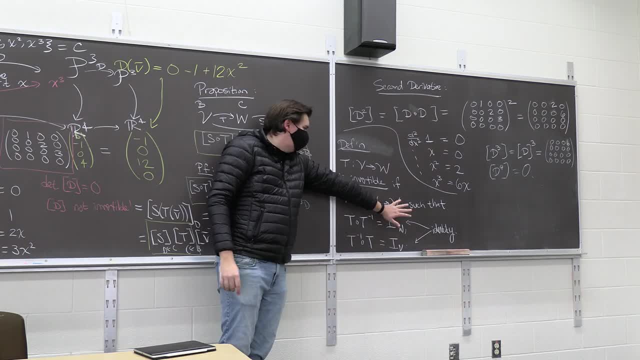 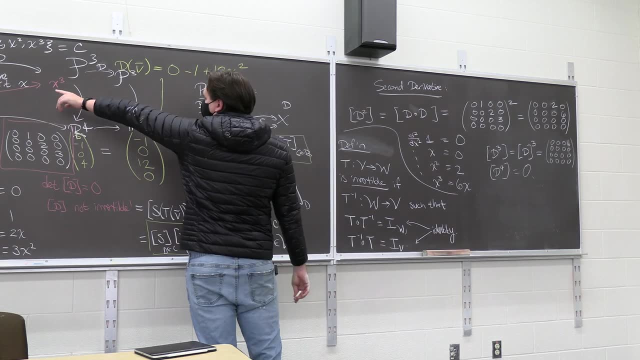 It's not a very interesting one, but keeping everything the same is a linear transformation. So that's what it means to be invertible. it has some inverse. we just saw this derivative map doesn't have an inverse, and that corresponded with its matrix not having an inverse. 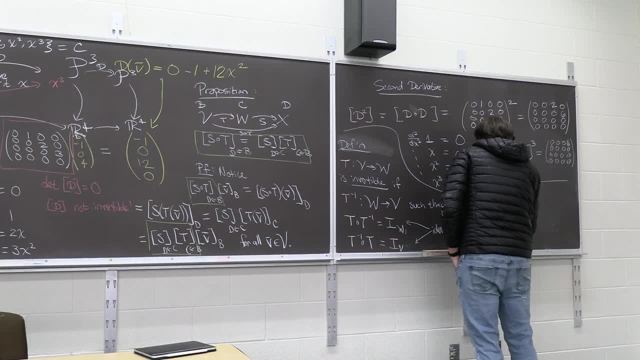 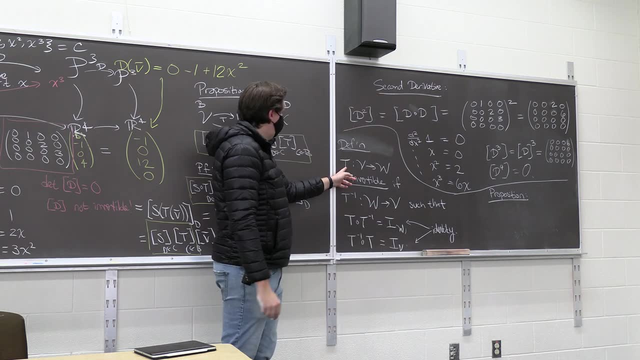 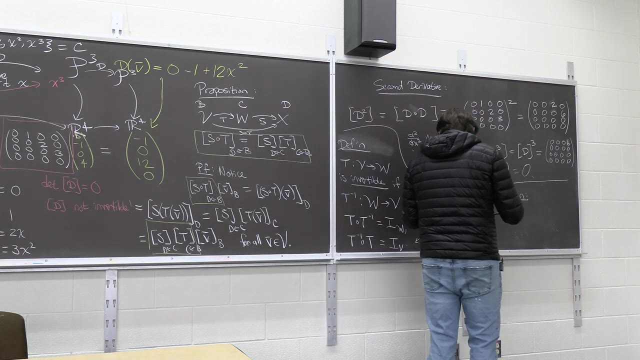 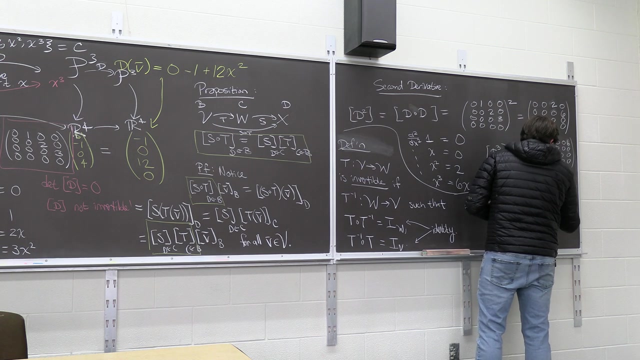 So that's now my proposition. I want to say for my proposition that your linear transformation is invertible exactly when the matrix is invertible, so if the dimension of v is the same as the dimension of w, if they're not the same, 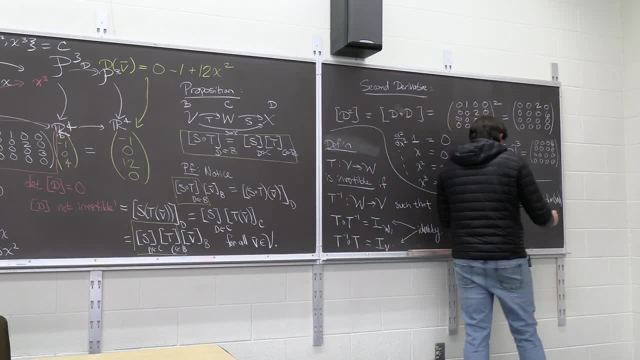 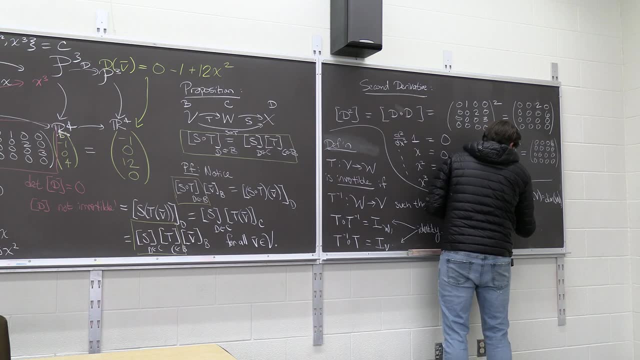 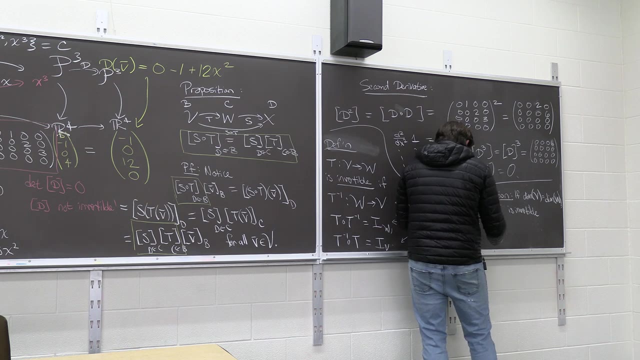 you don't even have a square matrix, there's no hope of it being invertible. then a linear transformation, t, is invertible precisely when, if, and only if, its matrix is invertible and the inverse of its matrix is the matrix of the inverse transformation. 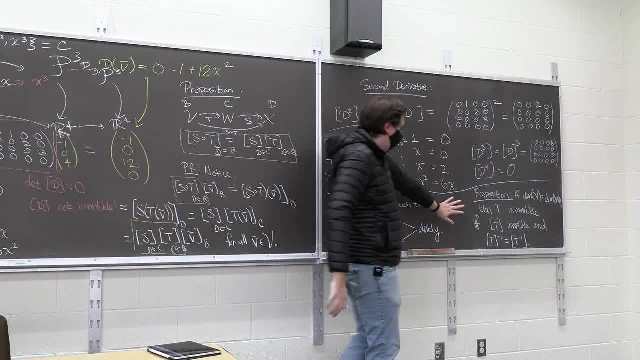 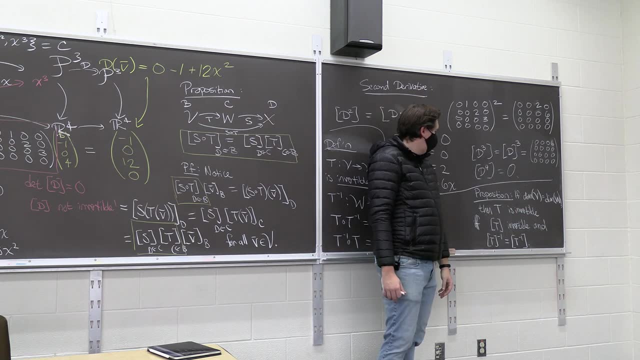 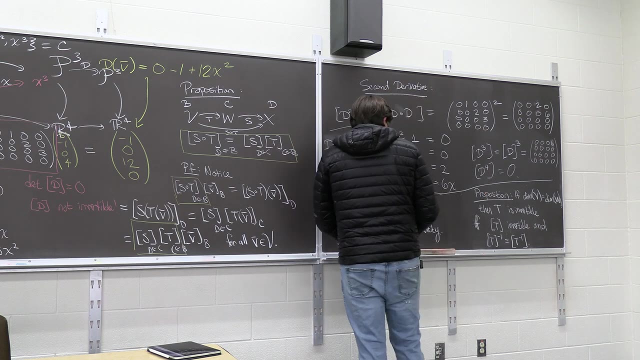 Okay, I didn't keep track of all the bases I was working with, but it's whatever the bases are for v and w, you know b to c or whatever our matrices are. So this guy wasn't invertible, so it's not a really good candidate for this. 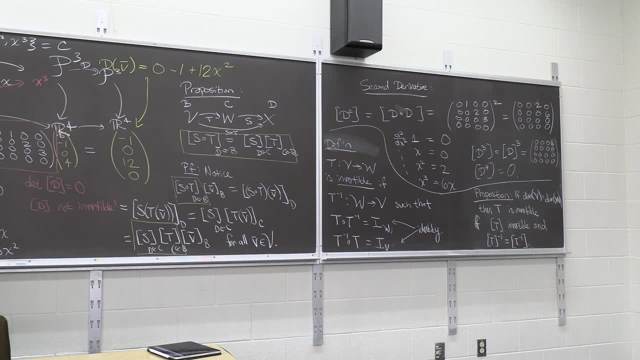 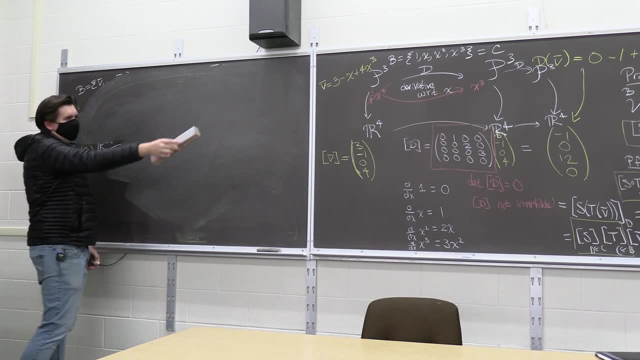 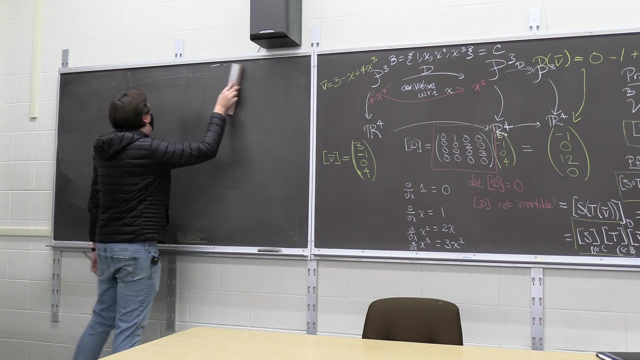 But maybe in the last couple of minutes I'll show you one other example of a derivative map where this does work. We're not going to go through this proof. it's very similar to the proof of compositions, so you can prove. this is also in the text. 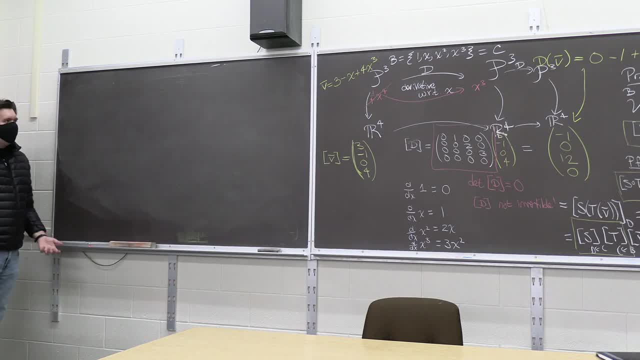 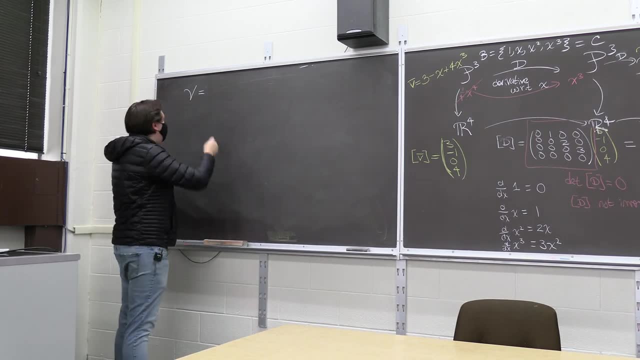 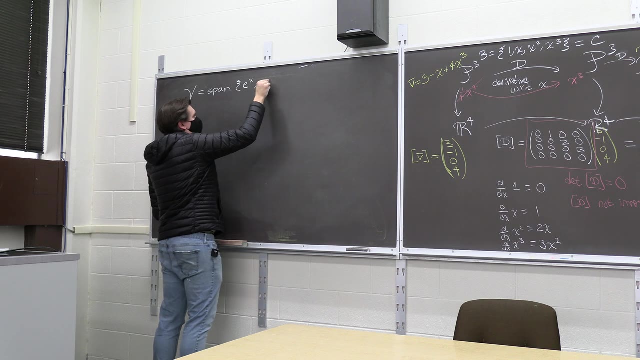 but I rather want to illustrate it. So what I want to do is I want to think about some vector space, v, which I'm not going to make these polynomials. instead I'm going to make it just the span of the elements e to the x. 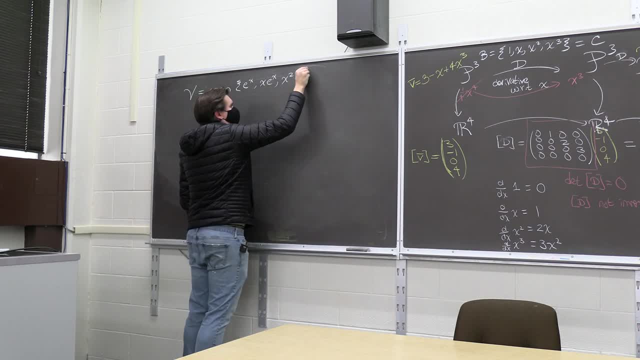 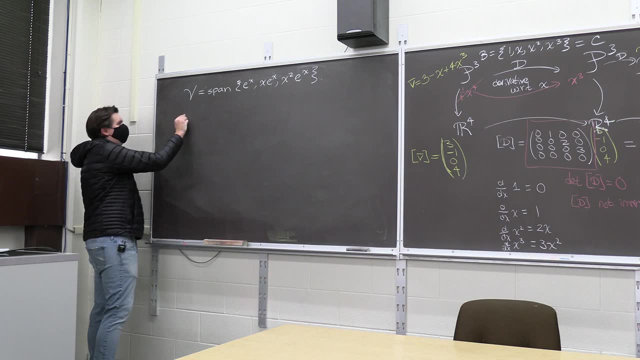 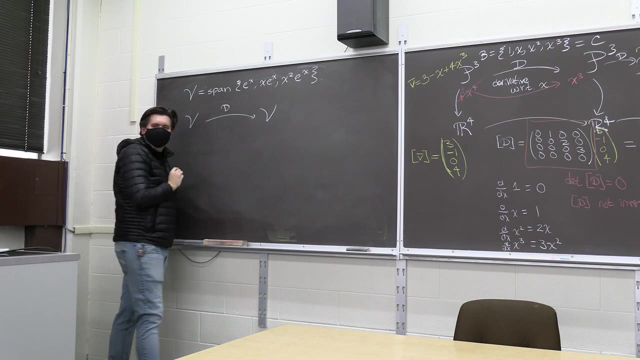 x, e to the x and x squared, e to the x. Then I claim there's some nice map d, the derivative map from v to itself. You might worry about this a little bit, so let's check this really fast And this is going to be over the reals. 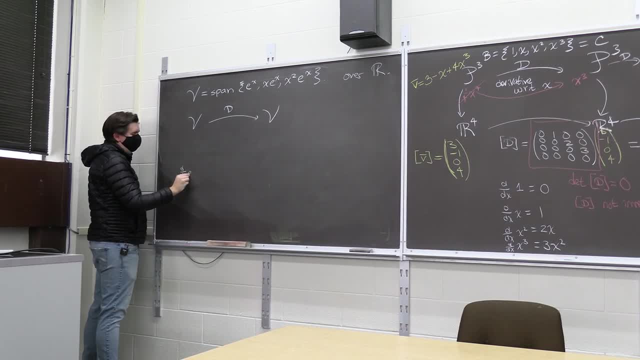 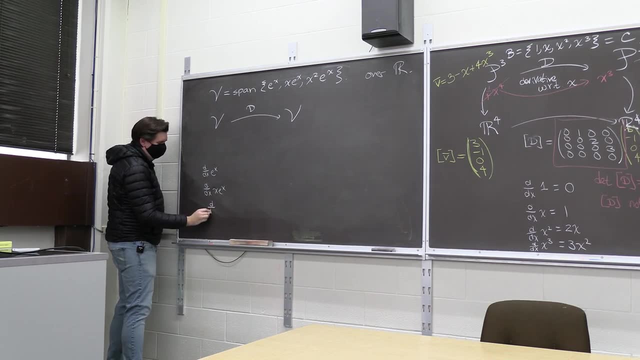 So what is the derivative of each of these? What is the derivative of e to the x, What's the derivative of x? e to the x And what's the derivative of x squared e to the x? See, if we can fly through this really fast. The derivative of e to the x is just e to the x, the derivative of x, e to the x. remember you have to do product rules. you hold the first drive of the second, which is just another copy of x, e to the x. 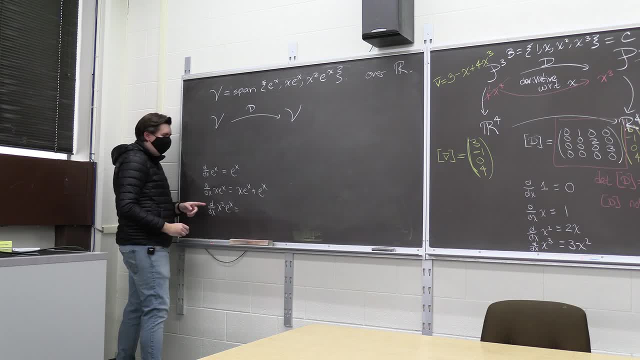 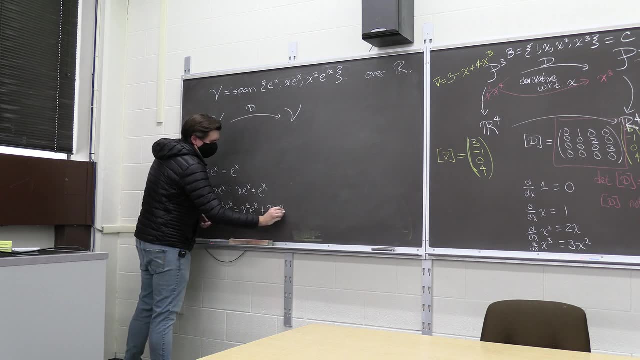 drive the first, hold the second, which is just a copy of e to the x down here. hold the first. drive of the second stays the same, plus derivative of the first, 2x e to the x. Note, these are all. 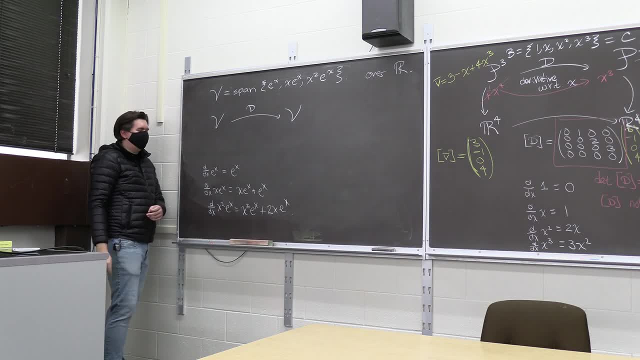 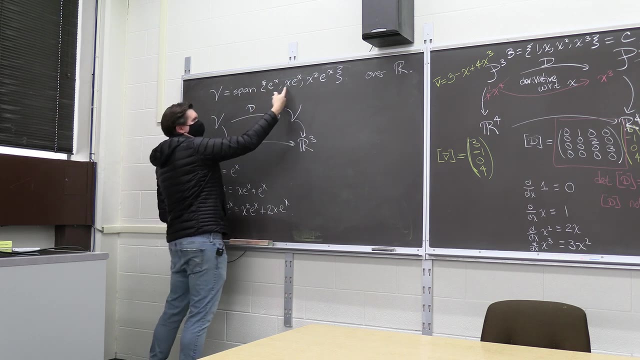 linear combinations of that same, of those same three vectors. So this really is a map from v to itself. So if we look at the corresponding matrix down here between r3 and r3, so this is just your basis- what does the matrix look like for d? 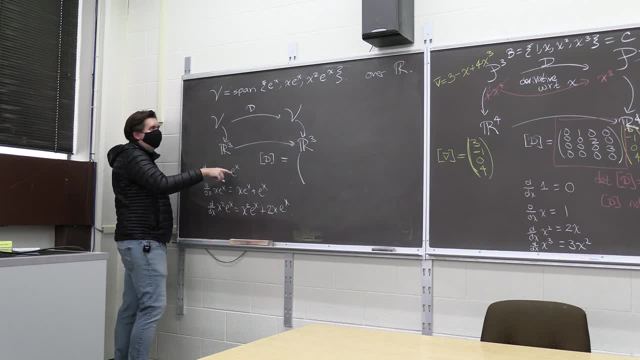 Well, e to the x gets sent to, e to the x. so this first guy gets sent to himself. so it's just 1, 0, 0.. This second guy gets sent to a copy of himself plus a copy of the guy prior. 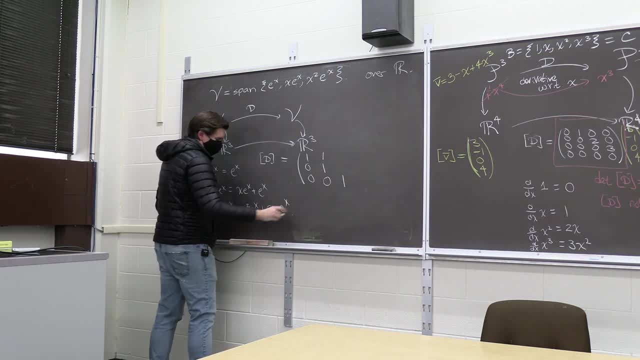 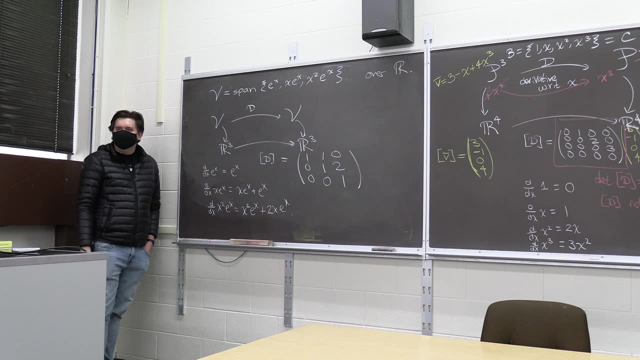 and the last guy gets sent to a copy of himself plus two copies of the one prior. So that's your matrix d And, like sure enough, you can check if you have some. you know, guy, here there's a linear combination of these guys. 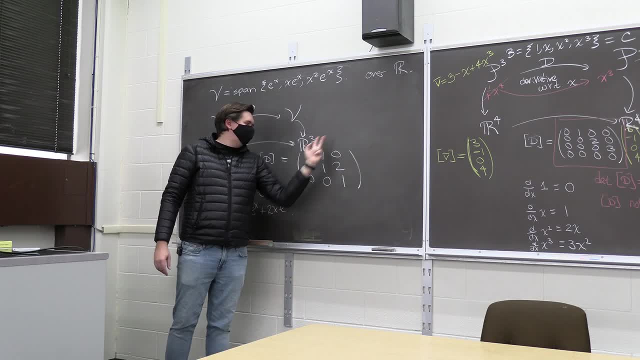 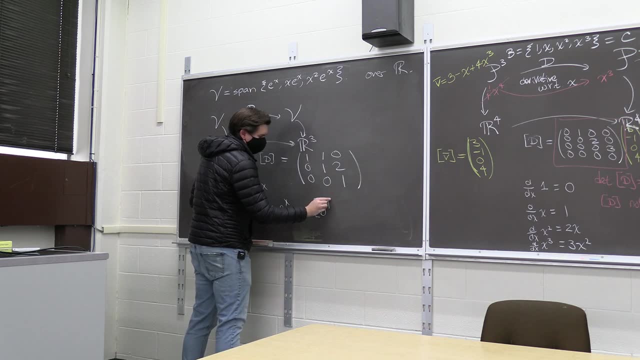 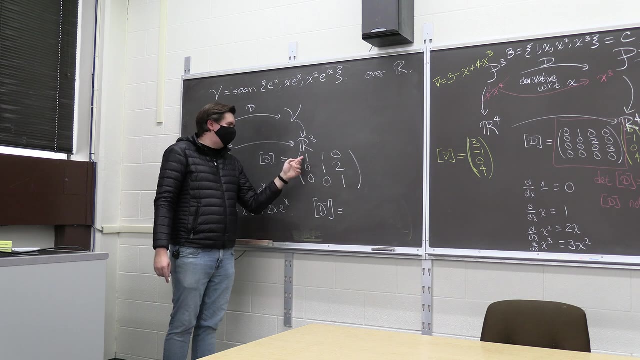 taking the derivative is the same as just multiplying its coefficient matrix by this guy. But what is d inverse? What is the matrix corresponding to d inverse? Well, does this have an inverse? It's upper triangular, so its determinant is just the product of its diagonal. 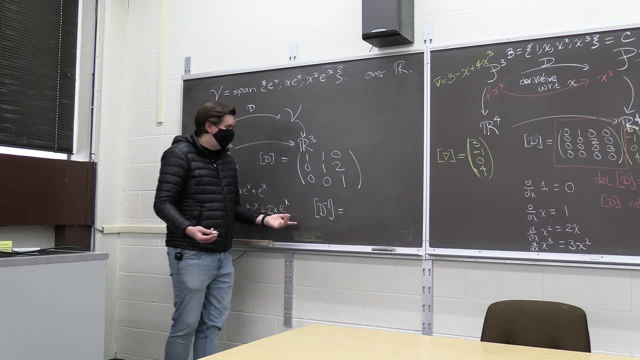 So its determinant is 1, so it's invertible, And so this is just going to be whatever the inverse of this matrix is. And so you can do it out on paper or you can do it like with a calculator. I wrote it down. 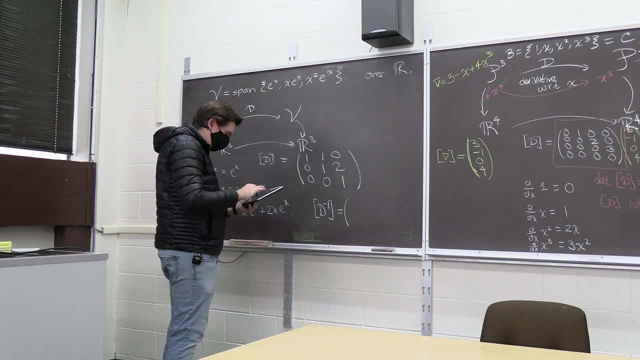 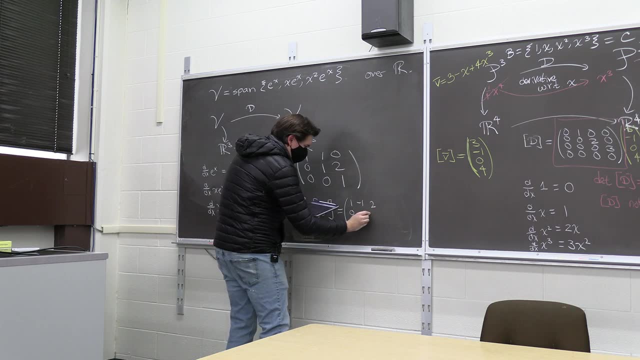 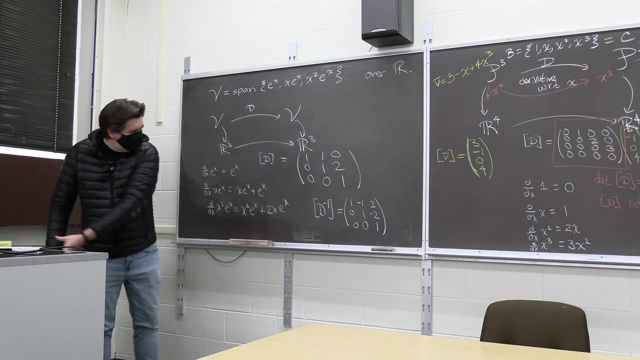 here The inverse comes out to be 1, negative, 1, 2, 0, 1, negative: 2, 0, 0, 1.. There's the inverse. So what does this matrix correspond to Like? what is your inverse?